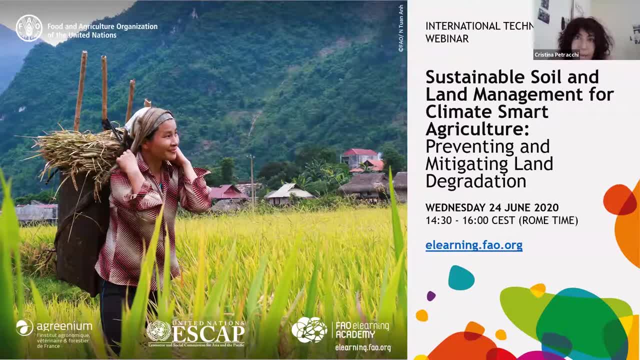 a number of thematic areas, And today we are going to be covering the area of soils management and restoration. The idea of these international technical webinars are really to find a space for exchanging experiences and sharing with each other knowledge and experience, And for this we are inviting a number of professionals throughout the world. 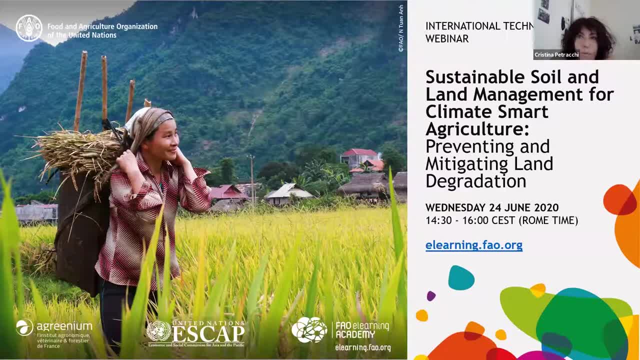 University professors, UN officials, United Nations, So we are trying to bring to the space a number of professionals throughout the world. So today I am extremely pleased to give the floor to my colleague, Feras Ziadat, who will be talking to you specifically about the webinar today. 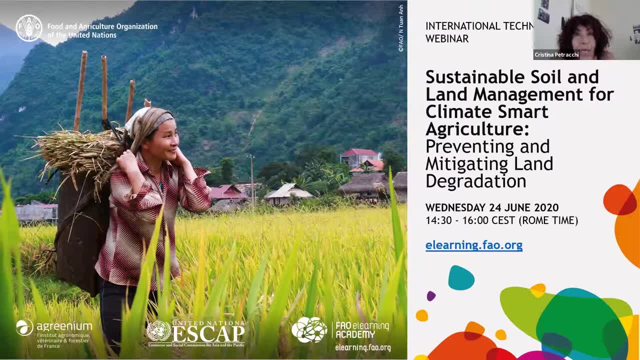 I also wanted to invite you all to visit the FAO e-learning academy. It is a multilingual platform that offers, free of charge, a number of e-learning courses that are on the various thematic areas that I mentioned before. So you have the link here. 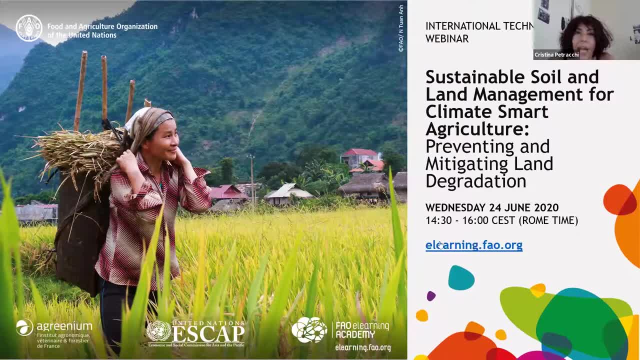 And so please try to visit the FAO e-learning academy, Feras. the floor is yours. Thank you, Christina. Good morning, good afternoon and good day for everyone from everywhere. Thank you, This is very good chance, and thanks for the organizers for organizing this important webinar. 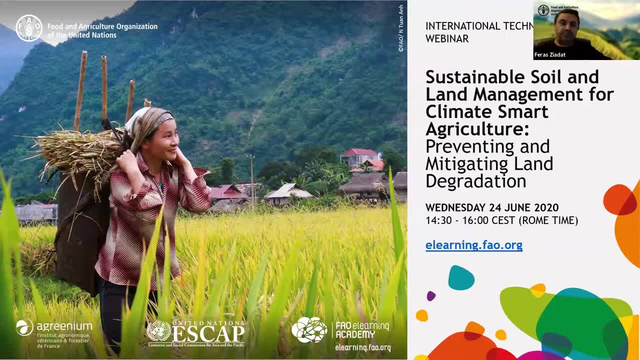 We are going to talk today about the climate change and how it impacted the agricultural productivity and food security And, of course, agriculture here is a source of emission and it's a victim affected by climate change, And we would like to see what kind of challenges and opportunities we have. 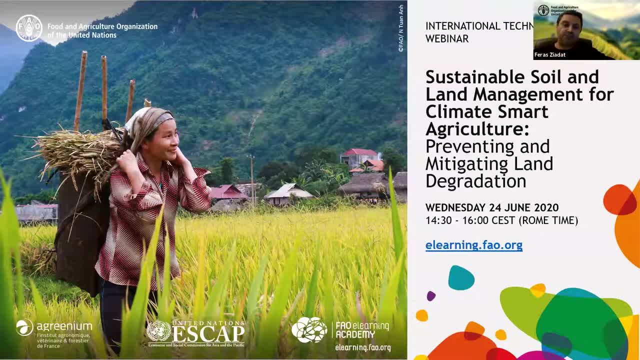 Climate change, adaptation and mitigation is very important And there is a role for sustainable soil and land management to play, And we would like to see how different practices on sustainable soil and land management will help in promoting sustainable agriculture. Thank you, Thank you. 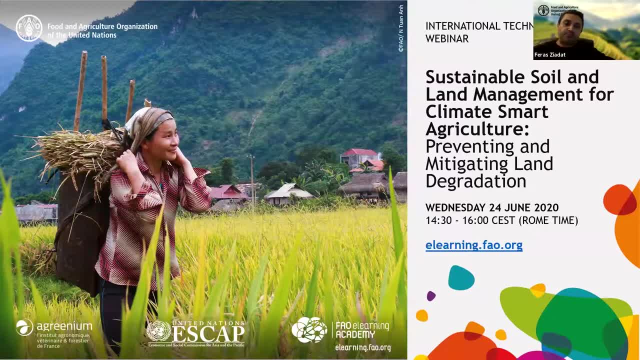 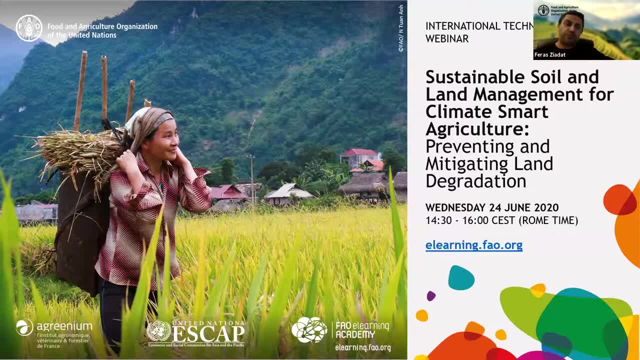 And then how to provide the conducive enabling environment that will help and support the implementation in suitable areas. and then the monitoring of these practices and other environmental aspects of implementing management practices in different environments. and then how do we look at the impact assessment and how these practices are enhancing food security. 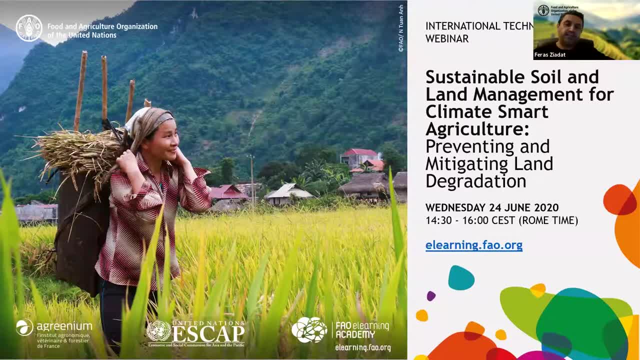 and creating enhanced adaptation and mitigation to climate change. So the issue is: the objective of this webinar is to look and present the impact of climate change on soil and land resources and then to look at some land management practices that will help us in tackling land degradation issues. and then what are the tools? 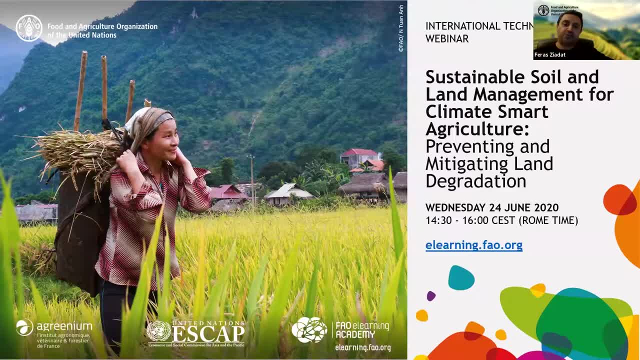 that are used to support the implementation of sustainable soil and land management measures. I would like to bring to your attention, as Christina mentioned, that this webinar is also documented in the Climate Smart Agriculture Sourcebook, and especially in Module No 7,, which is looking at: 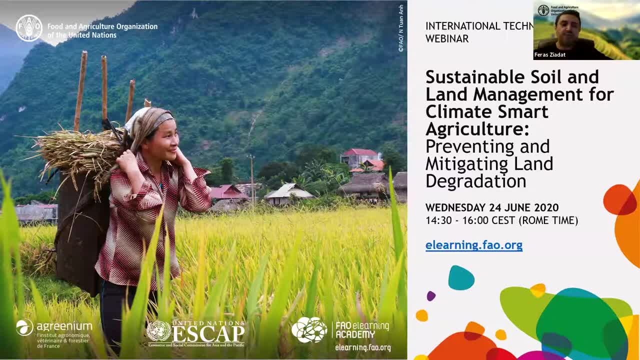 sustainable soil and land management for climate smart and land management, And there is an e-learning course dedicated to look at sustainable soil and land management in climate smart agriculture and I welcome you to look at this e-learning course and to go through the presentation. 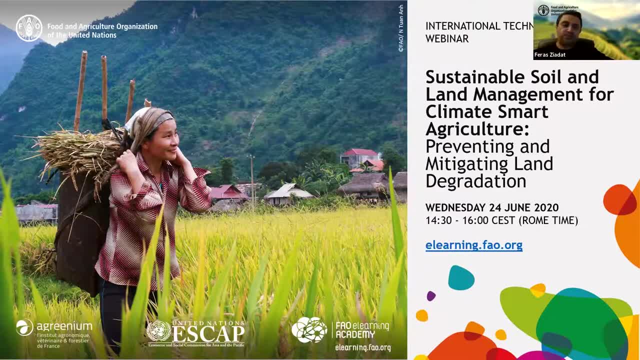 Finally, I would like to welcome the two speakers to this webinar: Professor Claire Tenoux, Director of Research at the French National Institute for Agricultural Research, INRA, and Professor Bandis Dolly, Senior Research Scientist with the Mediterranean Agronomic Institute of Paris. 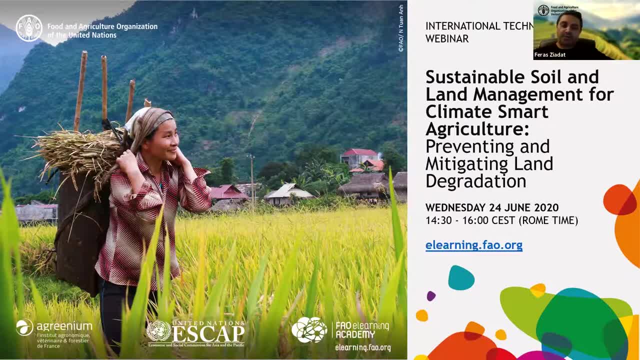 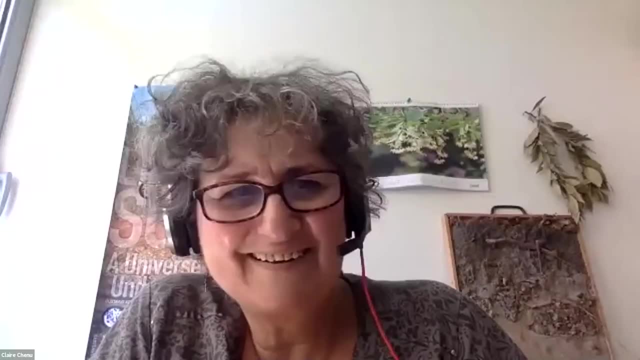 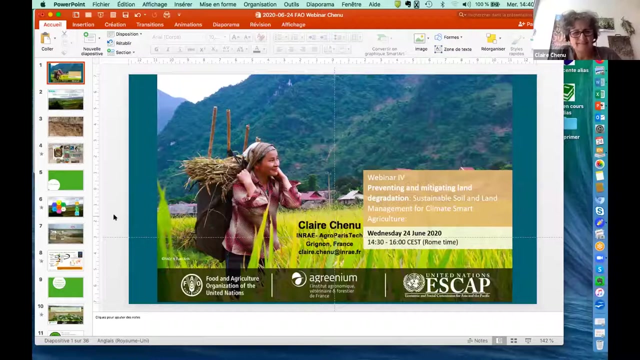 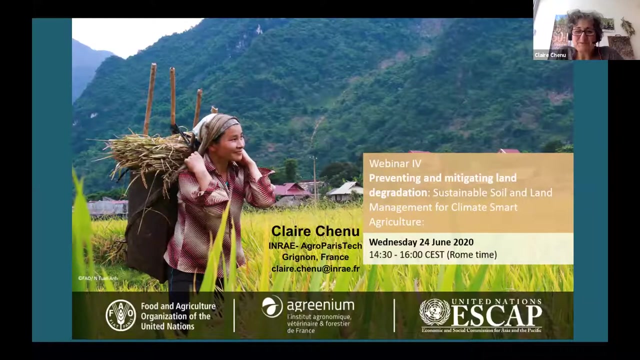 CIAM Paris in Italy. So by this I will give the floor to our first presenter, Professor Claire Tenoux. Thank you very much. Thank you Good afternoon. It's a pleasure to talk to you and discuss with you remotely. 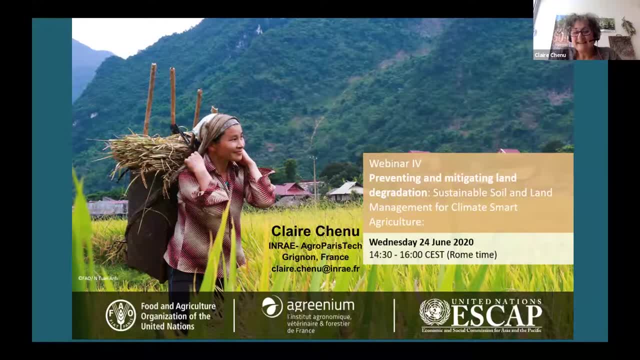 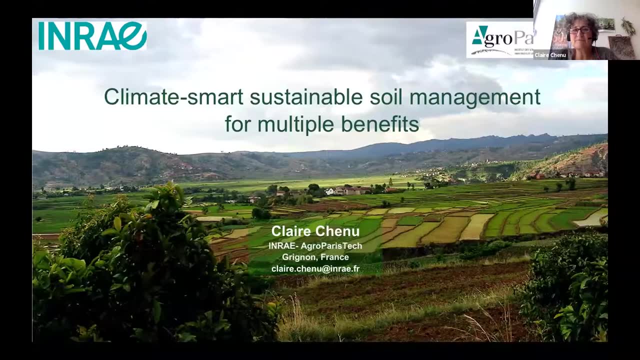 It's an honor to present a seminar here and I would like this afternoon to talk to you about climate smart- sustainable soil management for multiple benefits. So we're going to talk about climate smart- sustainable soil management for multiple benefits. We're going to talk about soils. 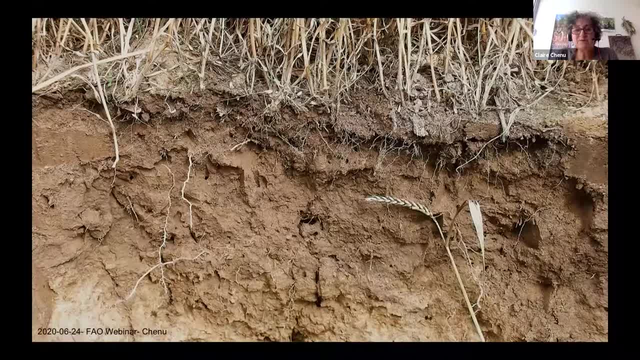 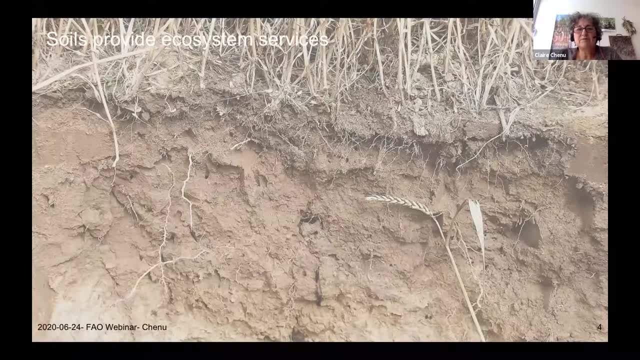 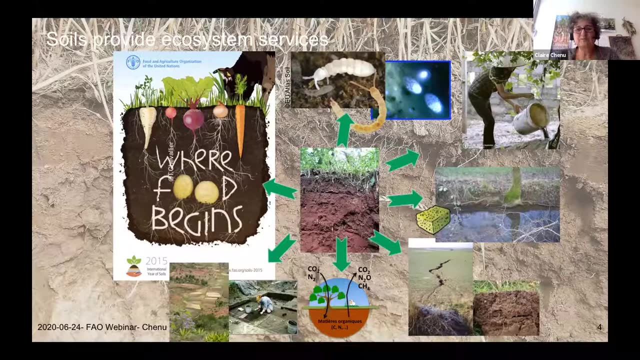 Why soils? Because you know, soils are absolutely key to life, to our human societies, because they provide ecosystem services. They provide, of course, they are first where plants grow, so that's where food begins. They are the provisioning food service. They also host a tremendous biodiversity. 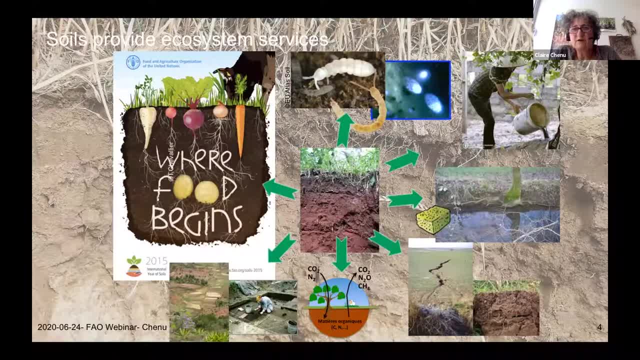 They have an important role in the recycling of nutrients of our organic wasters. They have a major position in the water cycle: retaining, infiltrating, transmitting water. They regulate- or not- erosion, which is a major stress. They have an important role in climate change mitigation and they also have cultural 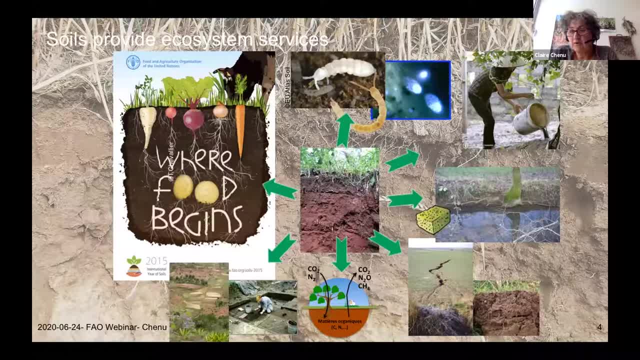 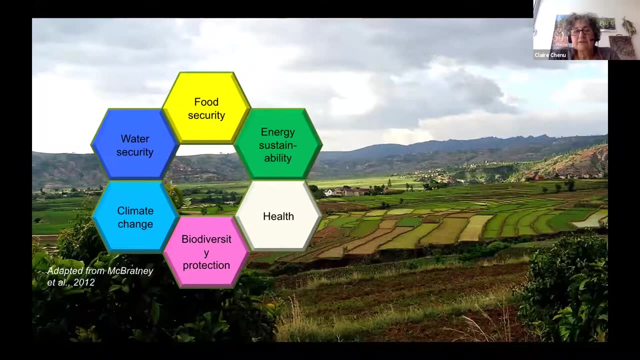 they also provide cultural services. They are hosts of remnants or for previews of our ancestors' activity and they are components of our landscape. But there are other factors, But there are challenges. Soils are important, but there are major challenges First. well, you know the challenges we have in our society now. 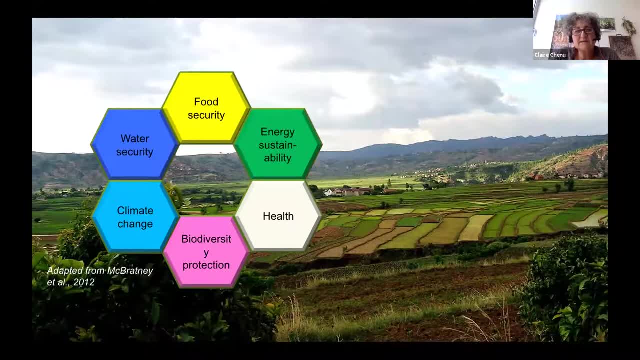 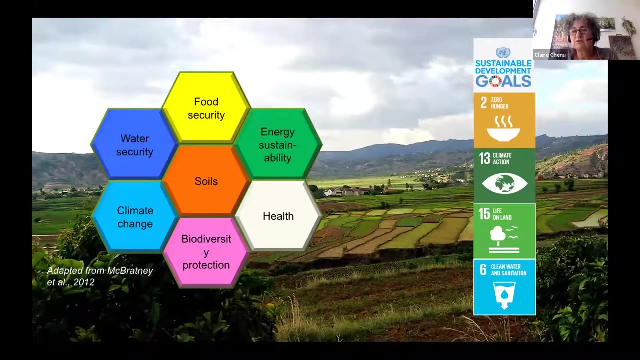 Energy sustainability, food security, water security, climate change, biodiversity protection and health. Well, we are right in the health challenge with this pandemic crisis, and soils are related to every of these challenges, So soils do contribute to the sustainable development goals. 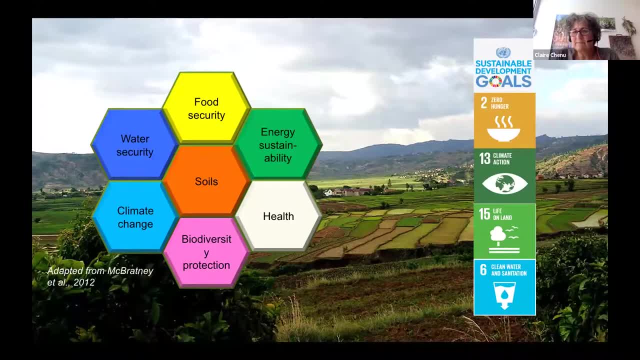 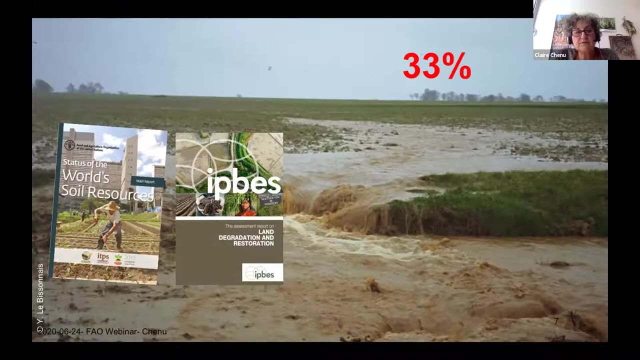 So soils do contribute to the sustainable development goals. So soils do contribute to the sustainable development goals: Zero hunger, climate change, life on land and clean water and sanitation. Soils are essential, but soils are in a poor state. Actually, two important reports: one by the Technical Panel on Soils hosted by the Global Soil Partnership. 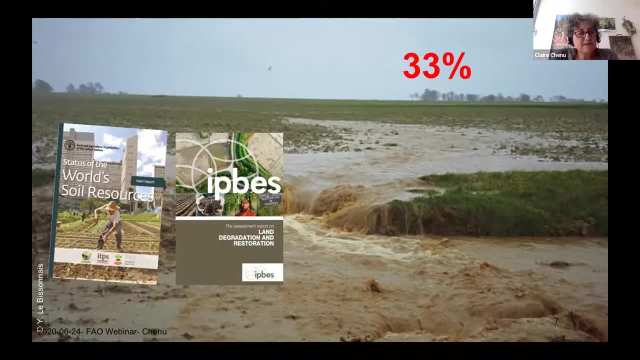 and the other one by the International Panel on Biodiversity and Ecosystem Services, established that, and the other one by the International Panel on Biodiversity and Ecosystem Services established that nearly one third of world soils are moderately or highly degraded. nearly one third of world soils are moderately or highly degraded. 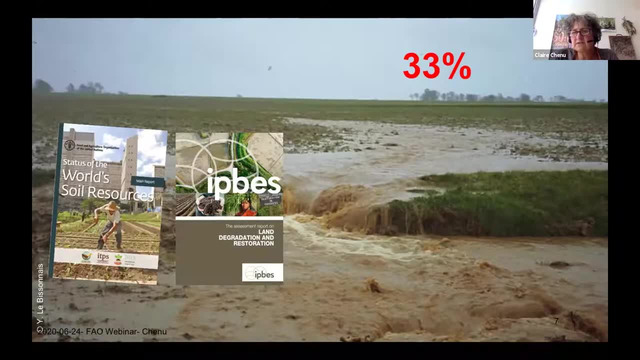 nearly one third of world soils are moderately or highly degraded. So this is really a problem. So this is really a problem. So this is really a problem, And it is particularly a problem in the context of climate change, And it is particularly a problem in the context of climate change. 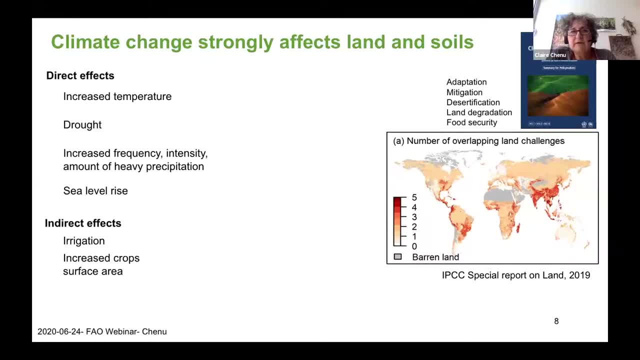 And it is particularly a problem in the context of climate change, where you probably know what are the effects of climate change, where you probably know what are the effects of climate change, where you probably know what are the effects of climate change: direct effect on land and on soils of increased temperature, of drought. 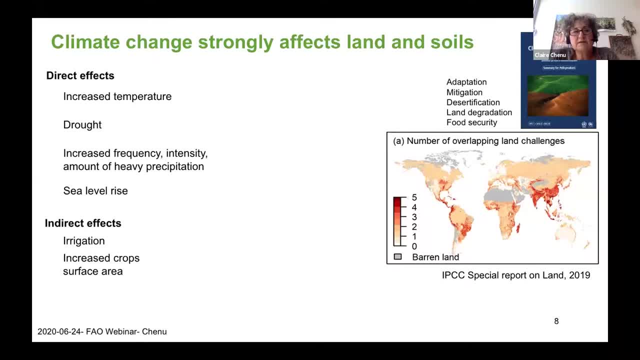 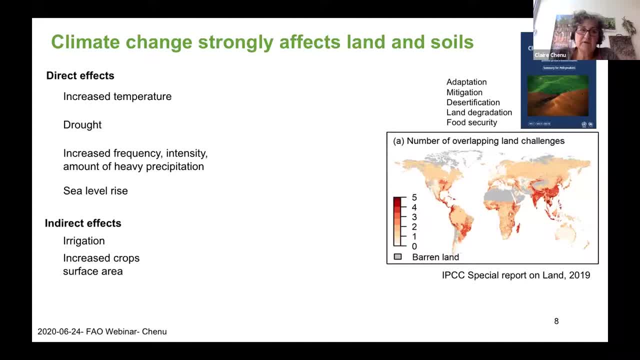 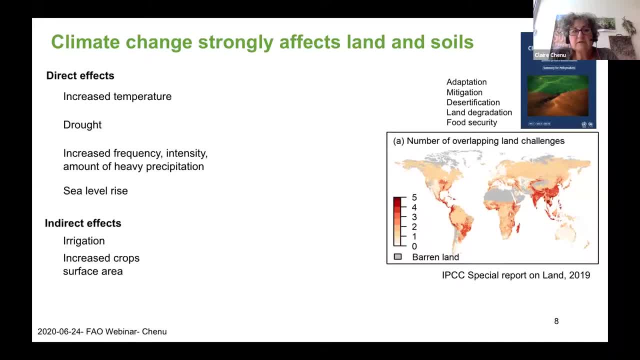 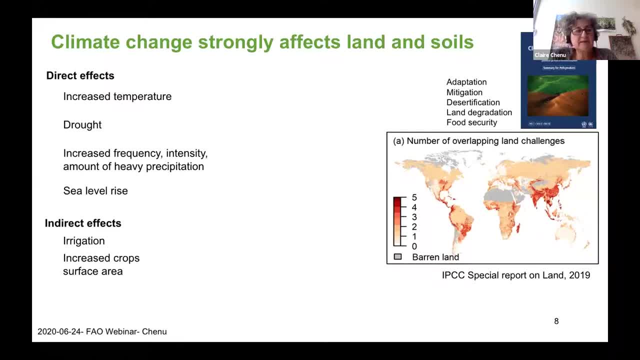 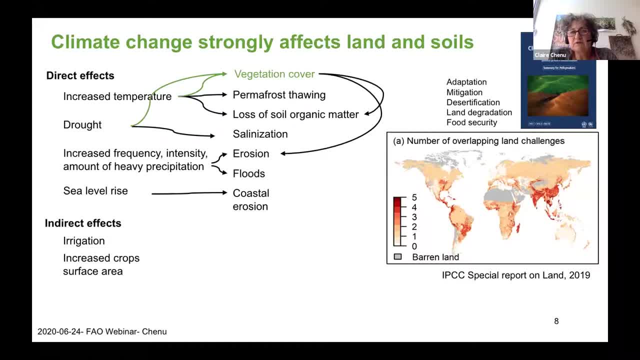 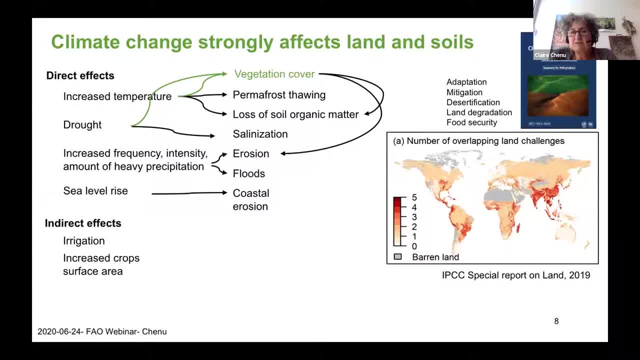 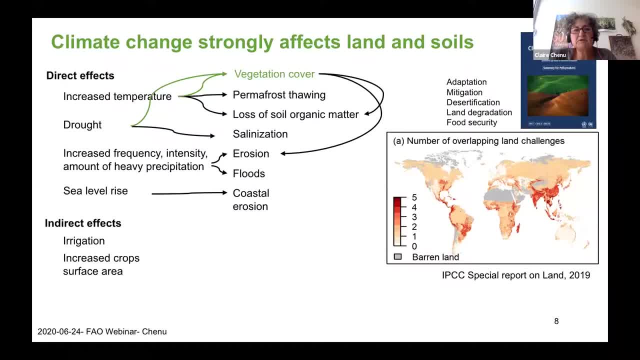 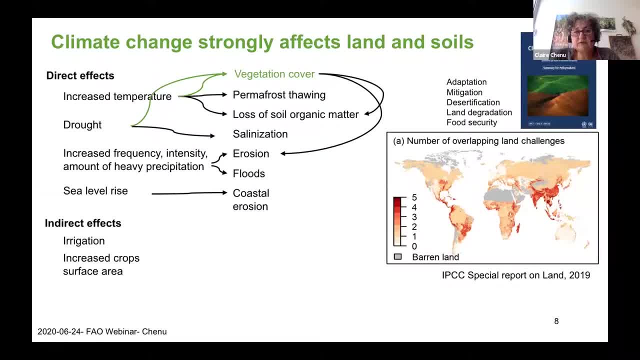 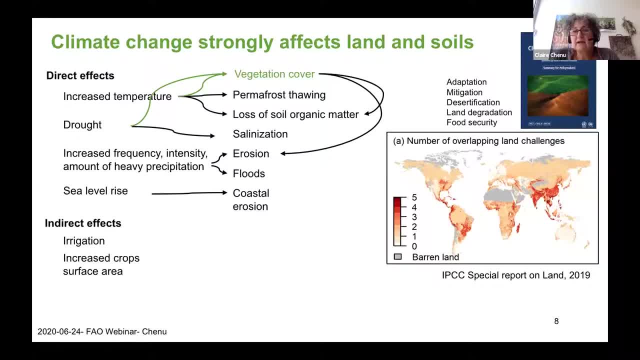 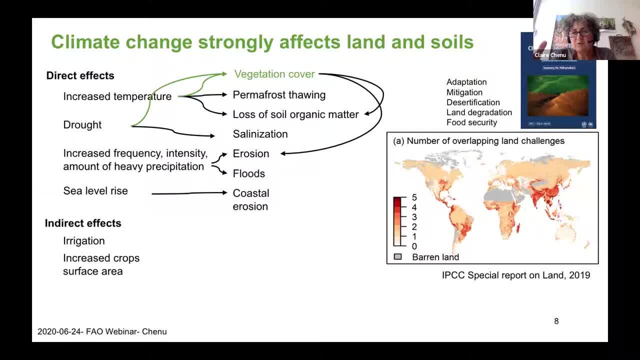 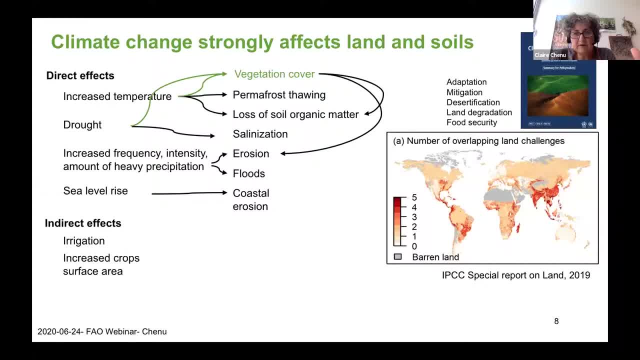 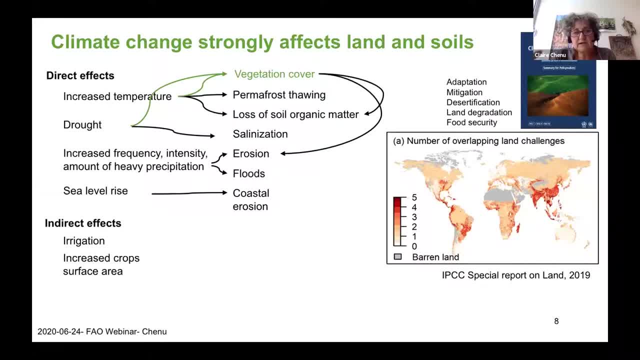 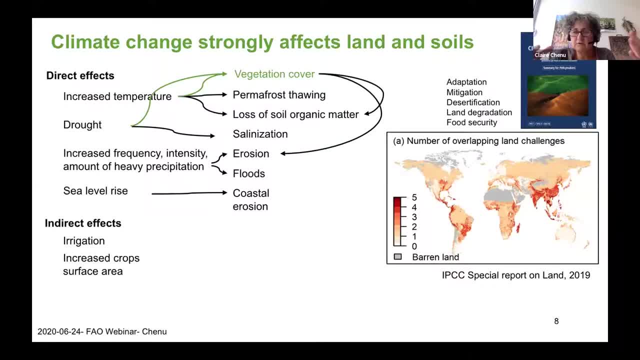 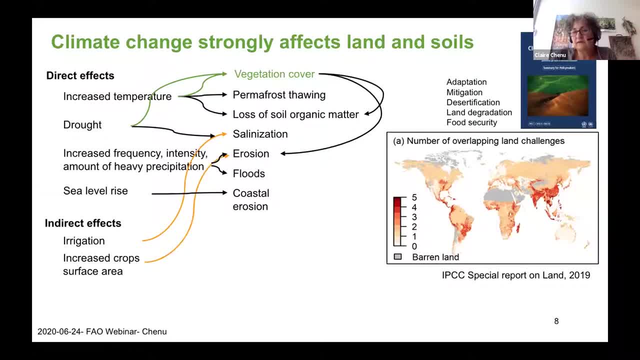 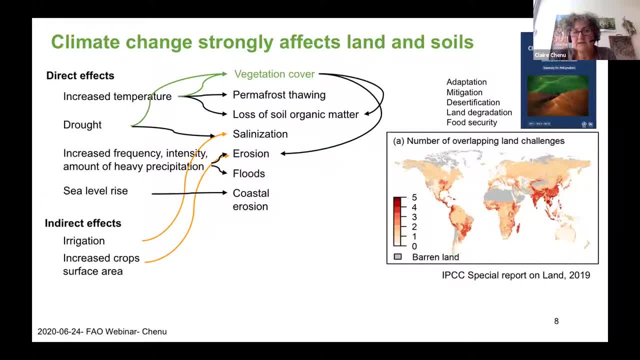 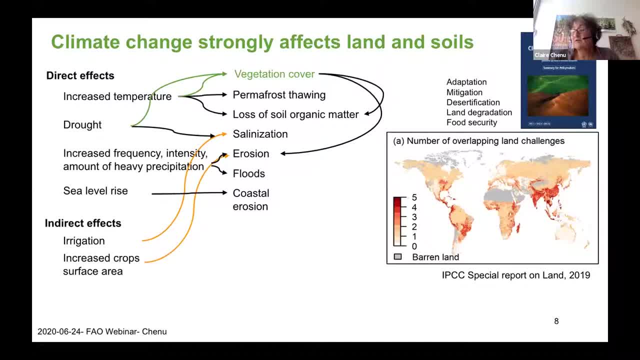 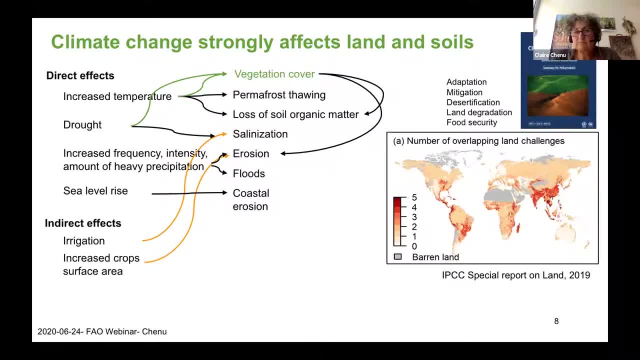 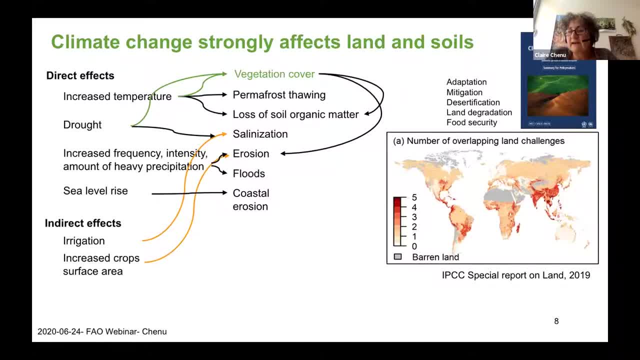 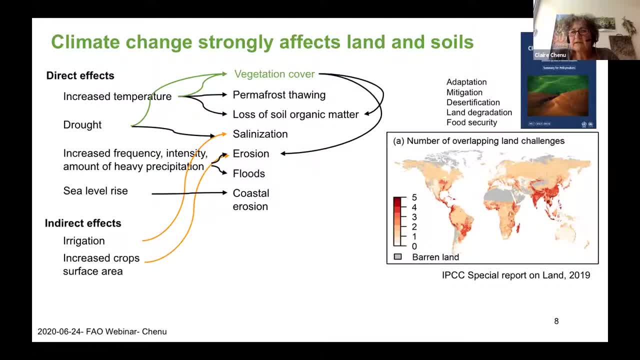 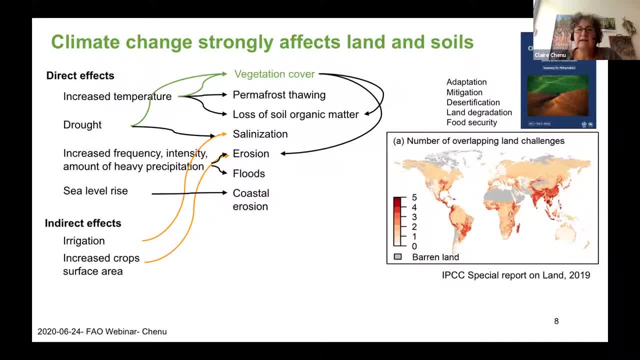 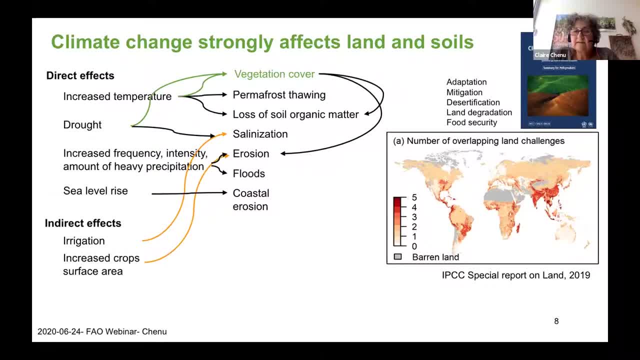 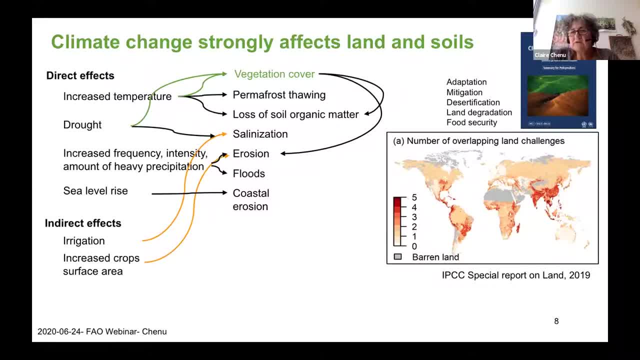 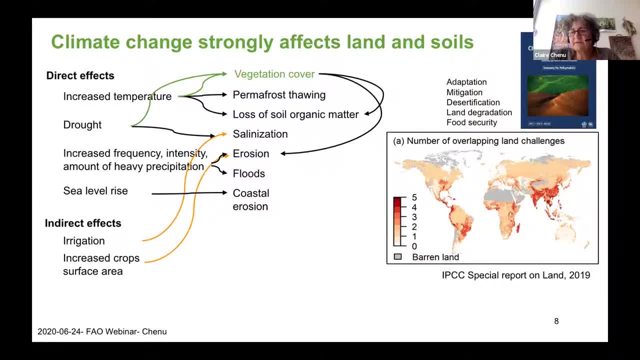 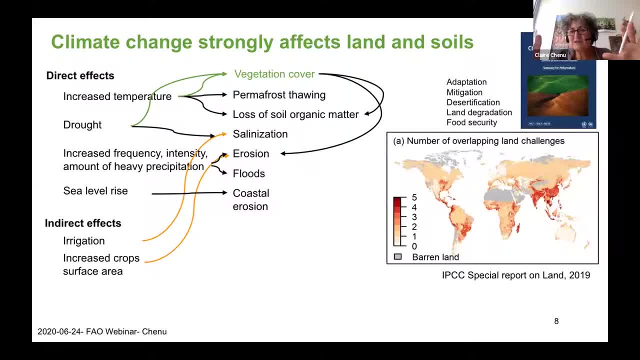 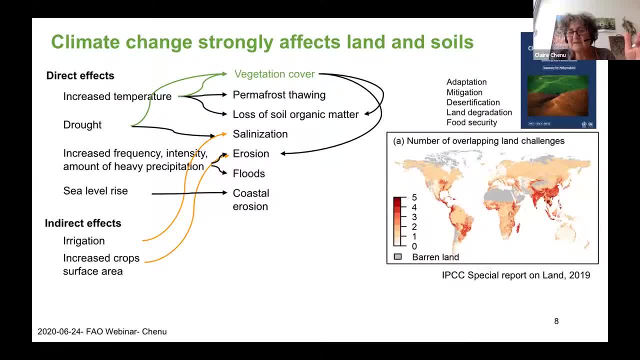 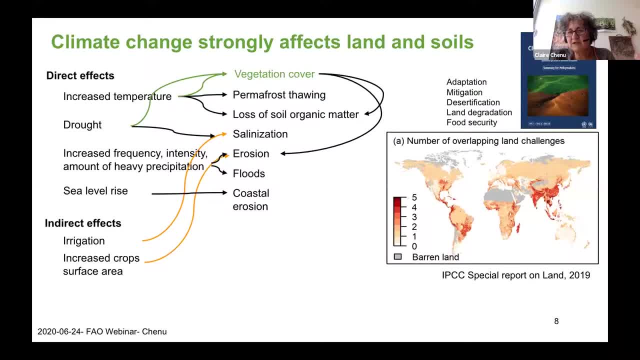 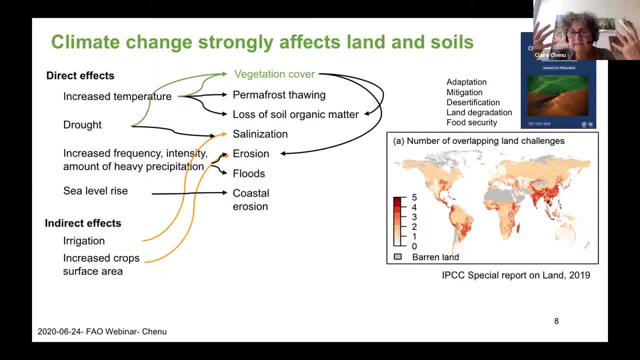 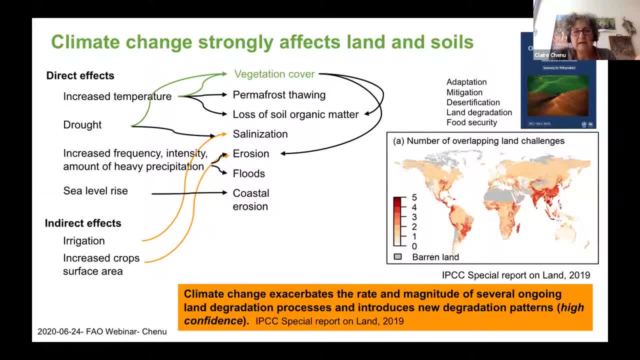 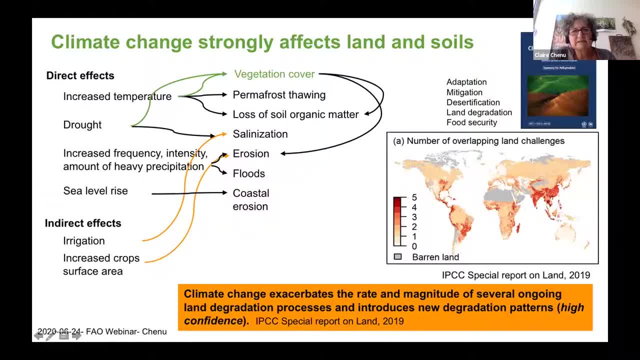 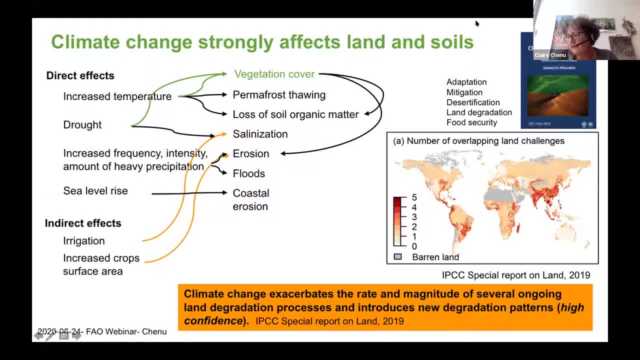 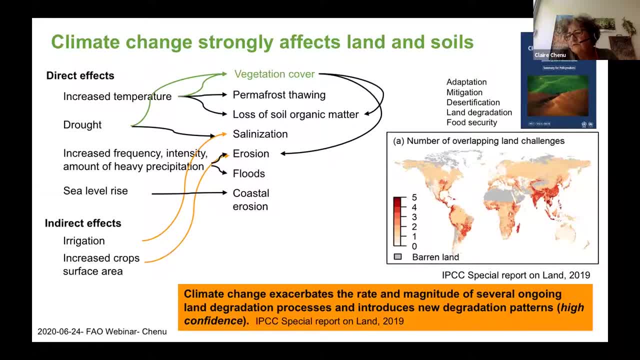 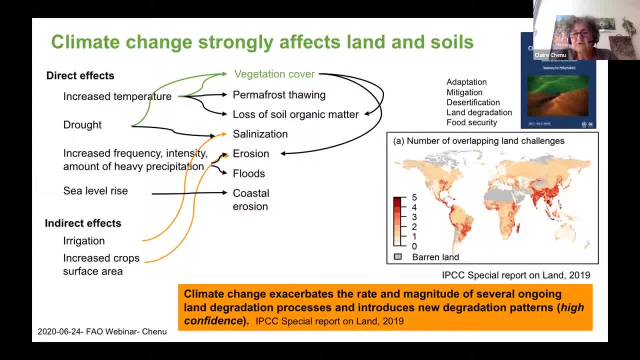 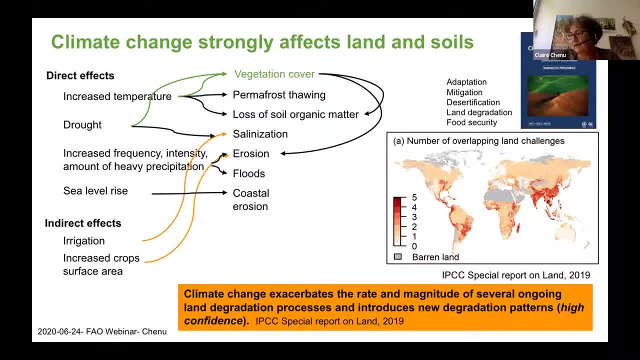 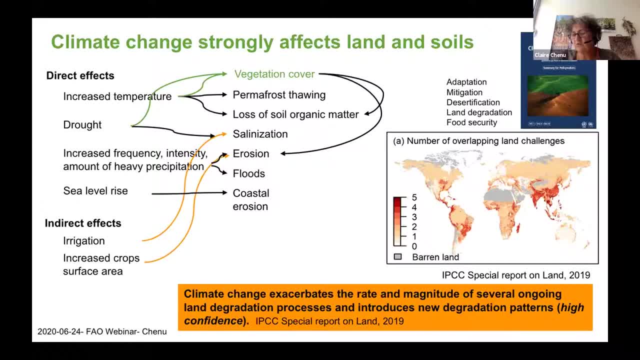 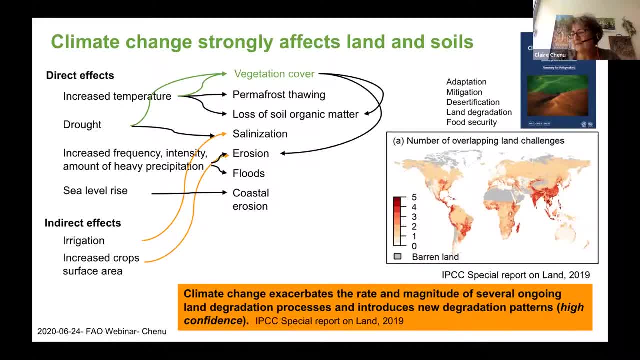 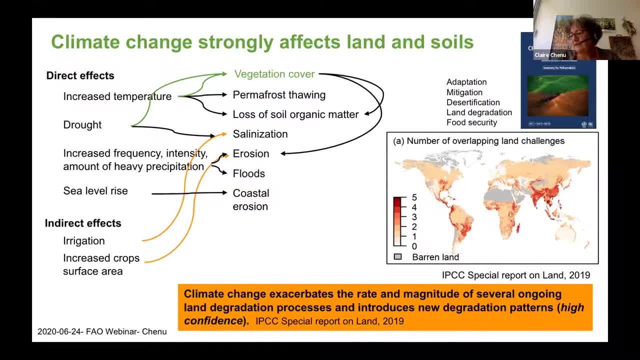 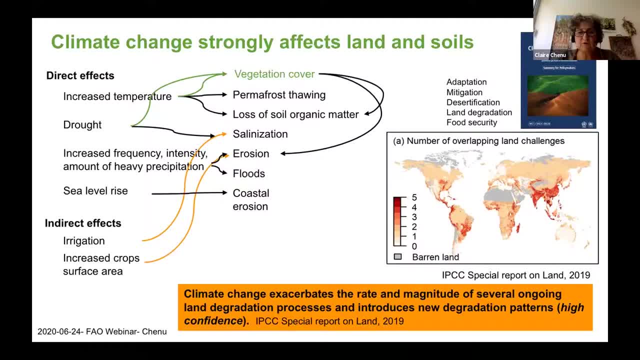 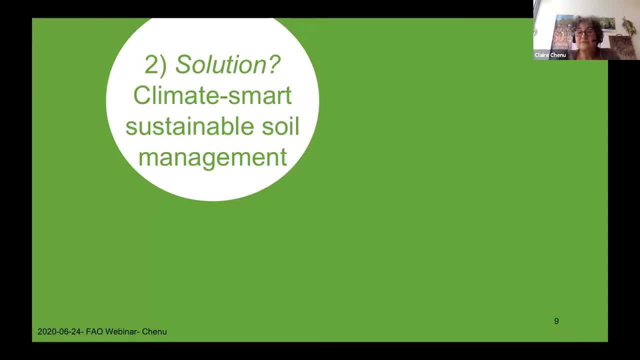 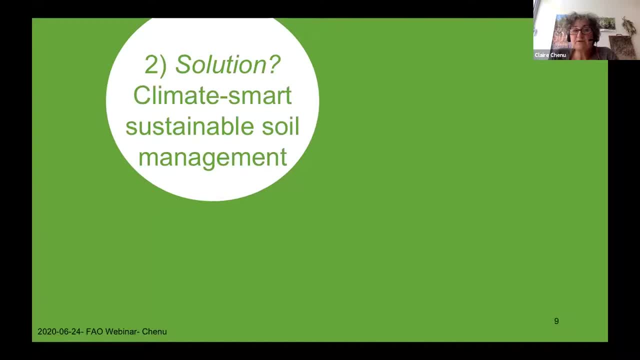 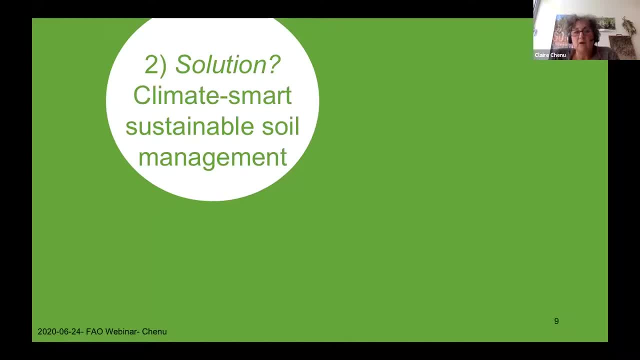 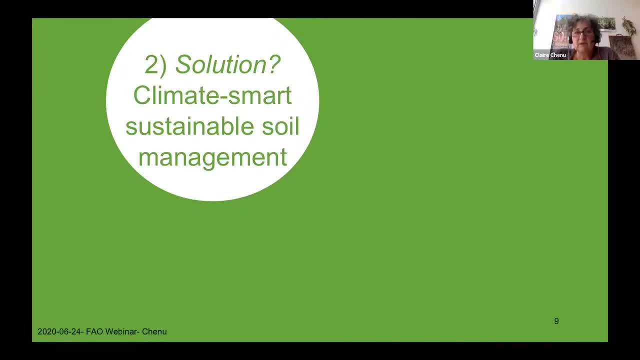 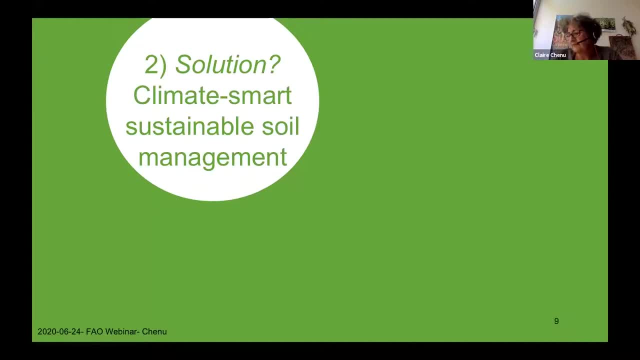 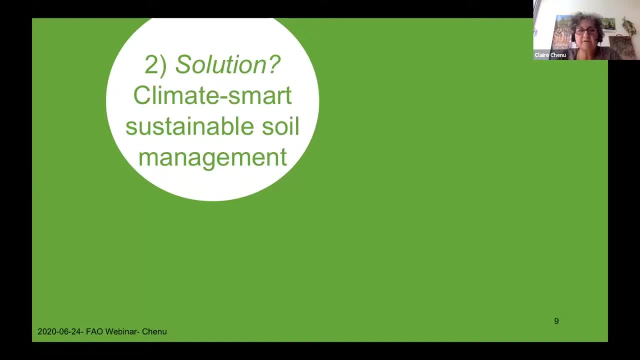 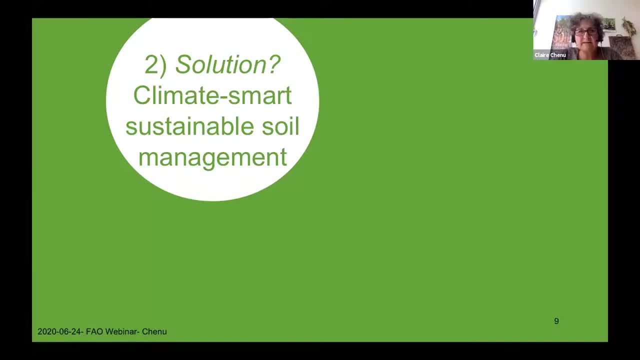 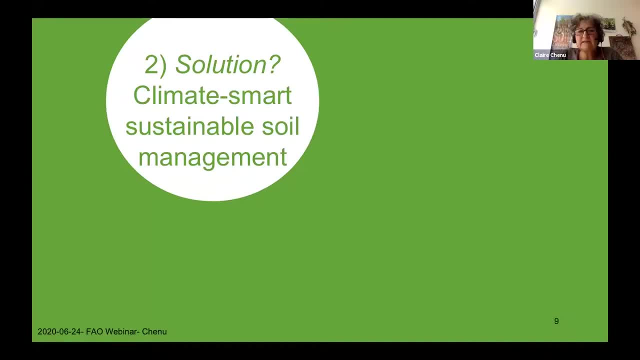 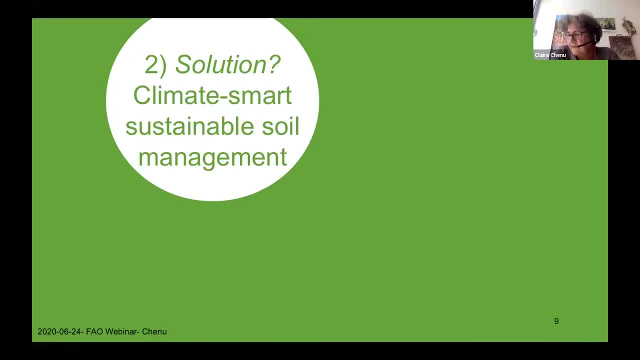 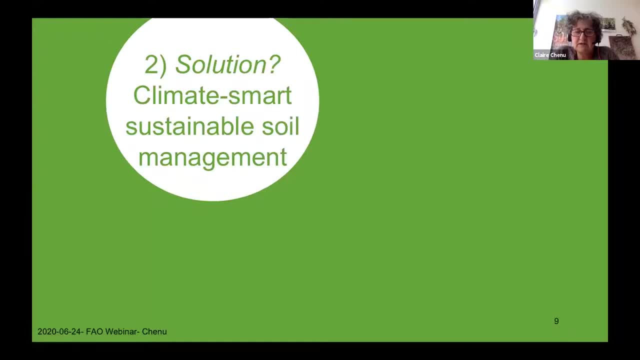 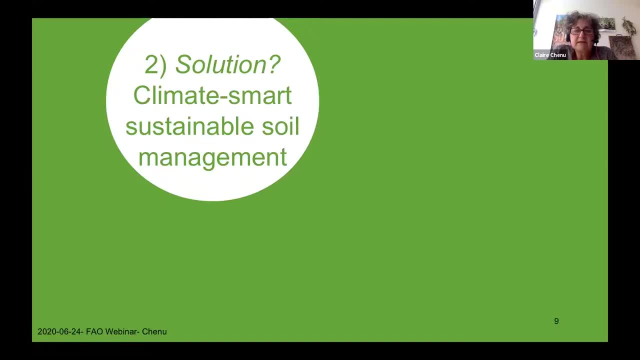 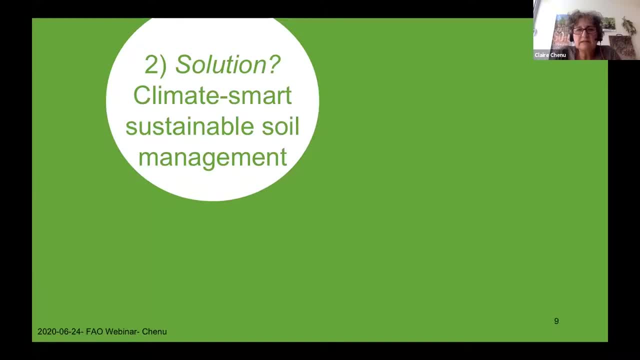 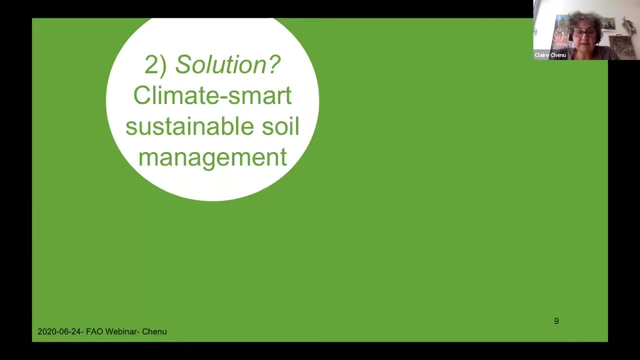 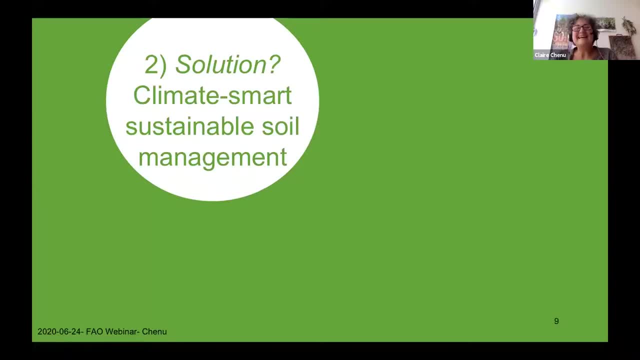 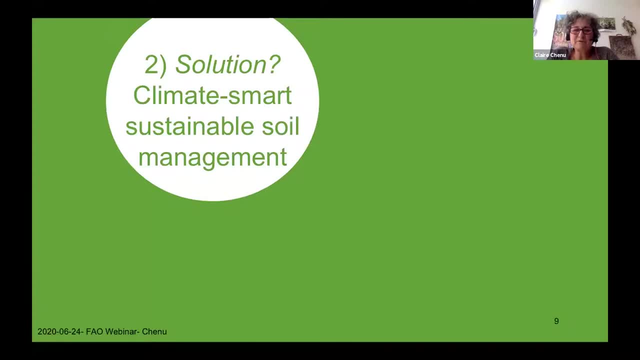 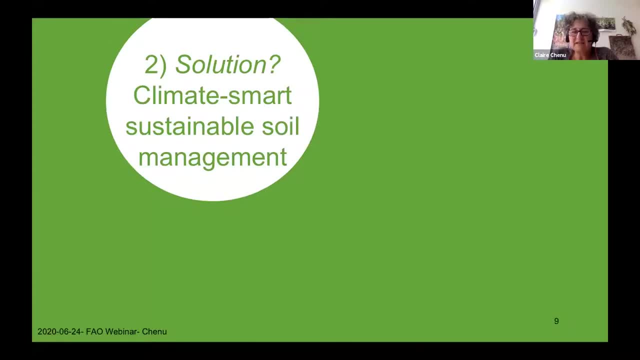 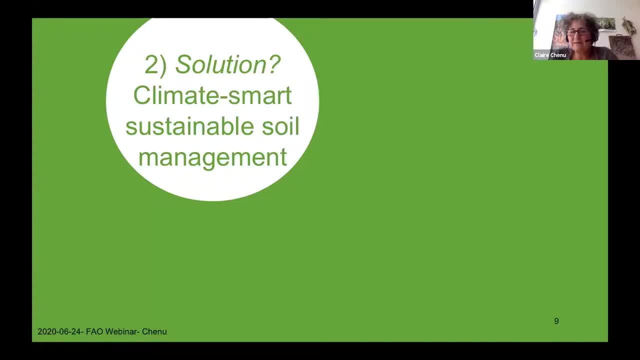 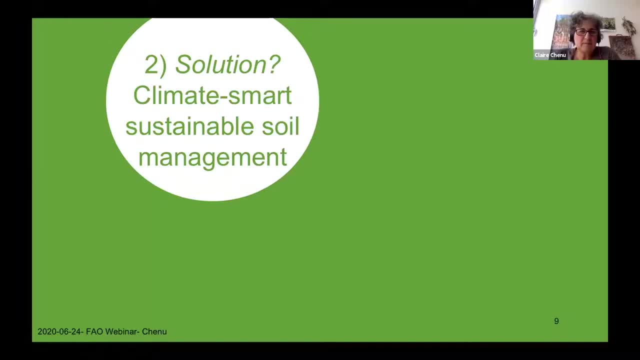 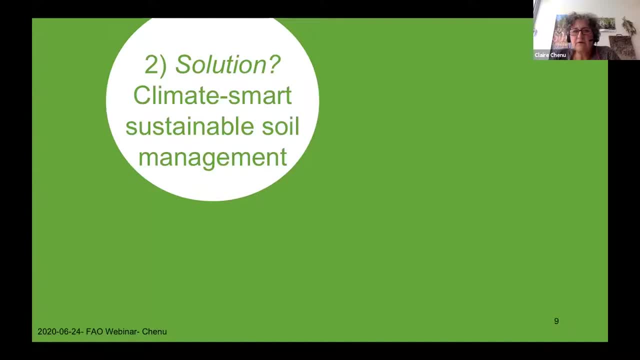 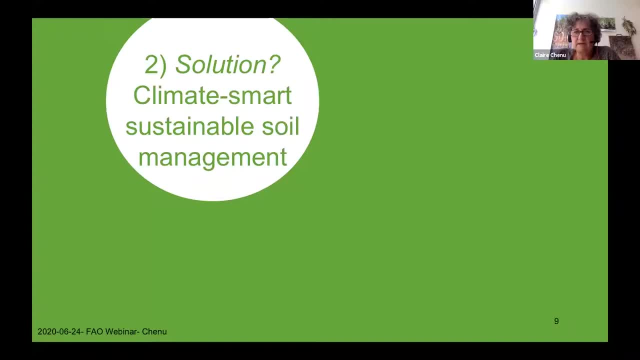 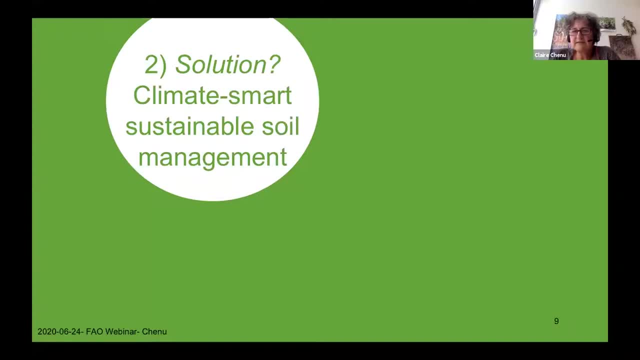 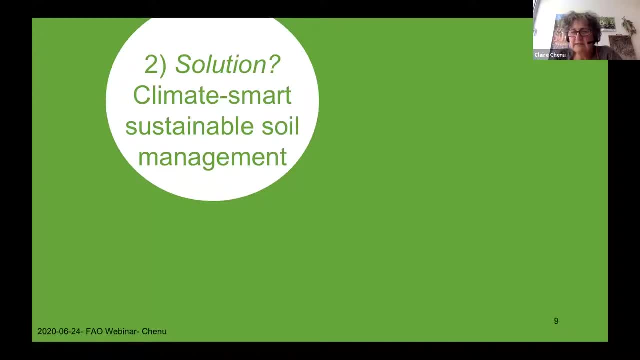 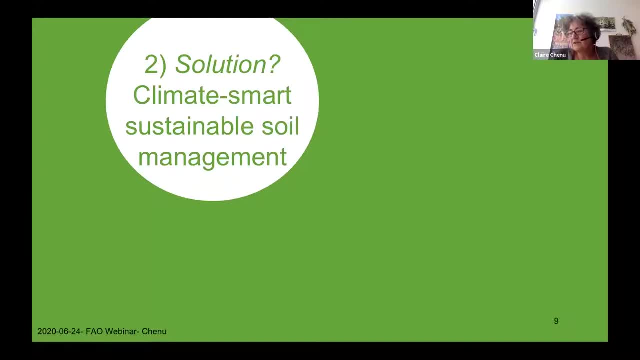 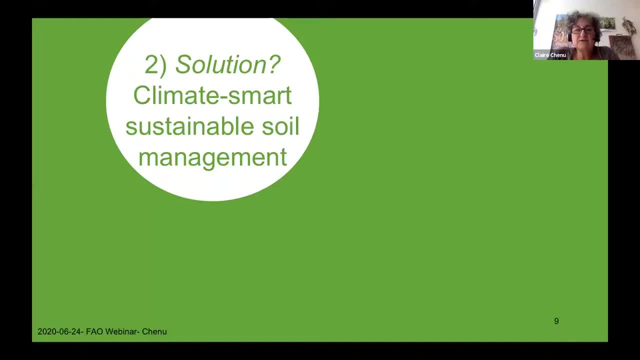 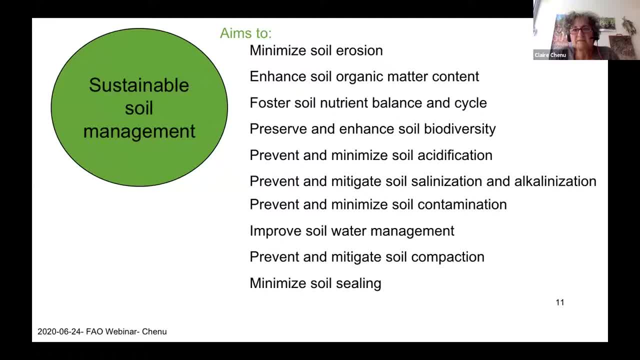 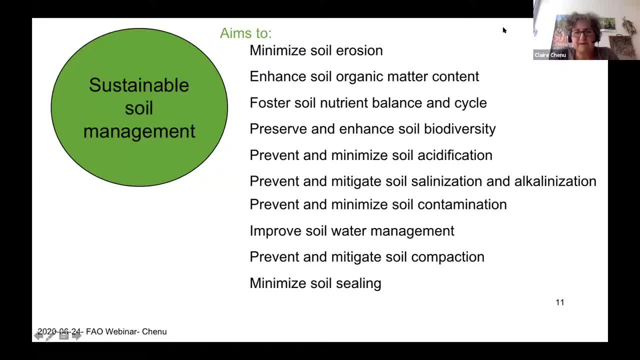 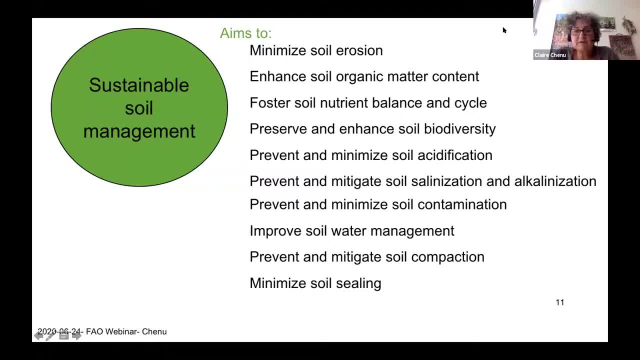 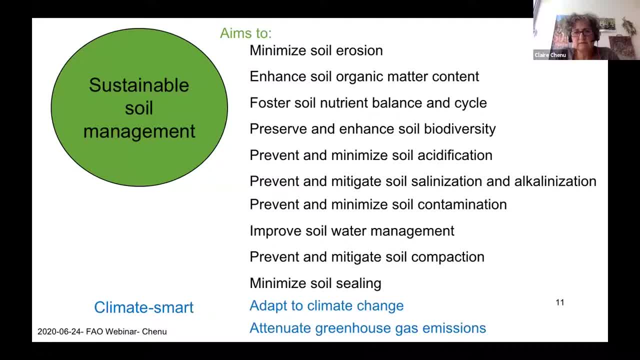 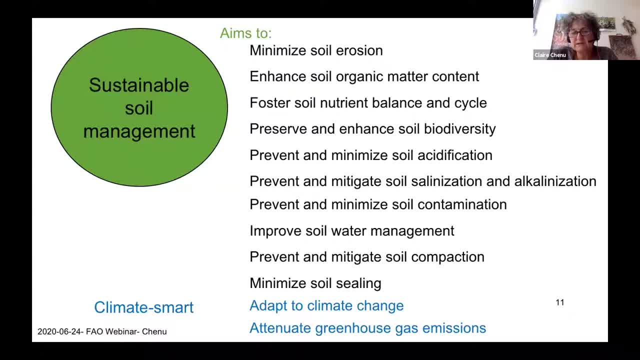 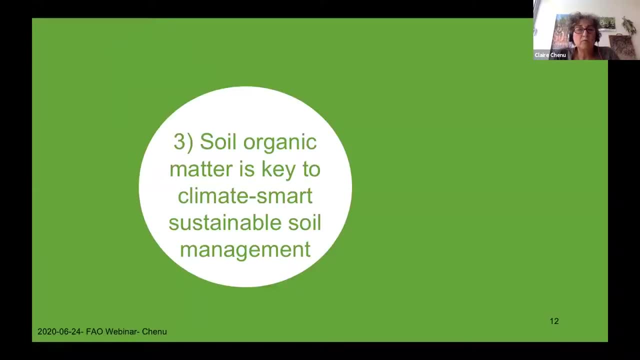 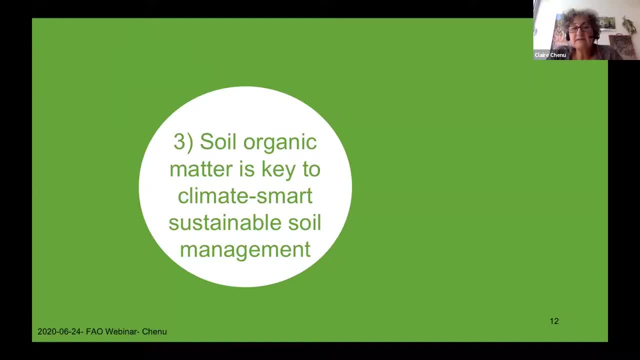 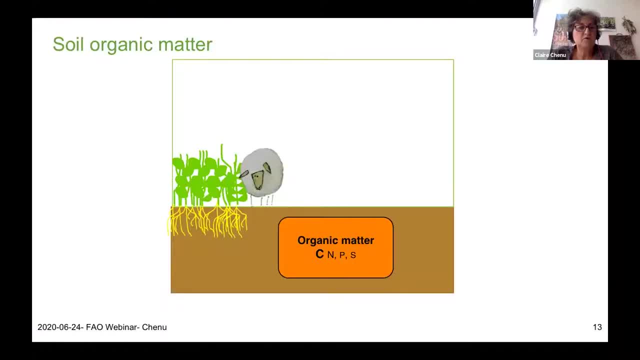 direct effect on land and on soils of increased temperature of drought. direct effect on land and on soils of increased temperature of drought management. You probably know that soil organic matter comes from the decomposition of the plant biomass and also microbial animal residues that its decomposition leads ultimately to. 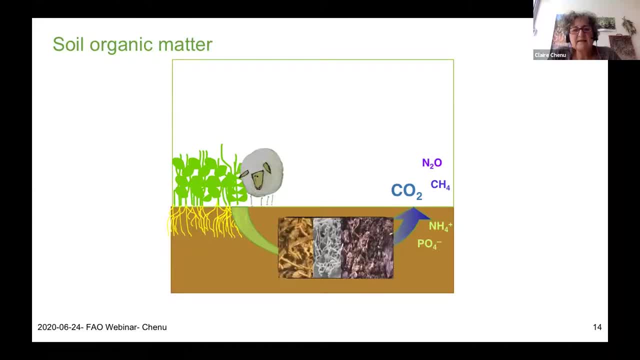 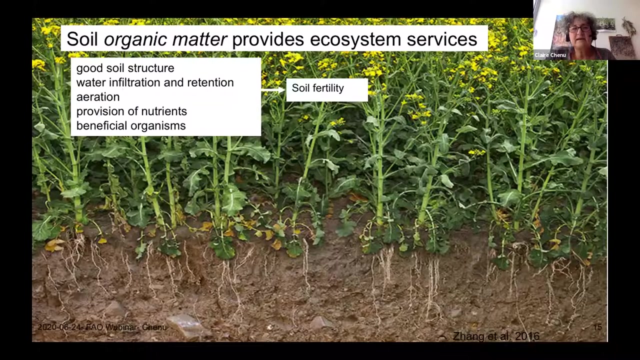 mineralization, with several elements being released, and that organic matter is extremely heterogeneous, being made of plant residues or animal residues, of alive organisms, and of a range of molecules, of very small particles, organic particles and a range of molecules. so a complex matter. A complex matter that provides ecosystem services: good soil structure. 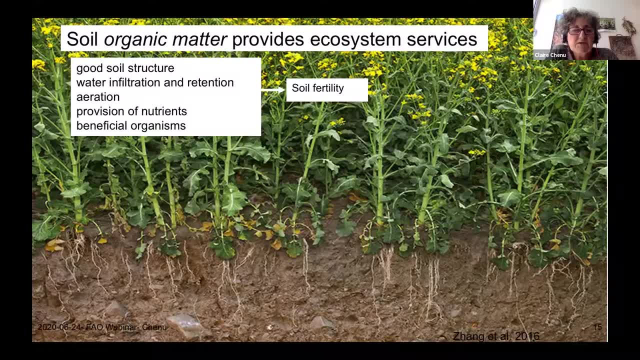 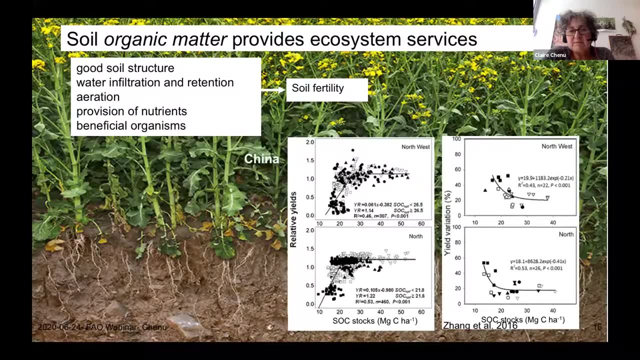 it contributes also to water infiltration and retention, aeration, provision of nutrients, beneficial organisms that are components of the soil fertility. Now one example. one example that comes from a meta-analysis that I've studied in China, where you have plotted in the x-axis, you may see soil organic carbon. 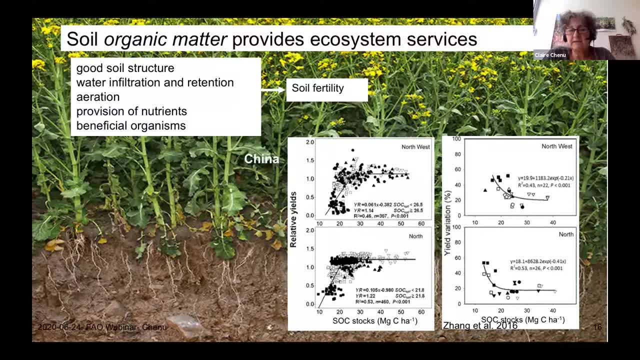 stocks and in the y-axis in the first graph you have relative yields compared to a reference plot. well, you see that the yields increase before plateauing: increase with soil, organic matter and maybe most original. more interesting is the second one, where it is the inter-annual yield. 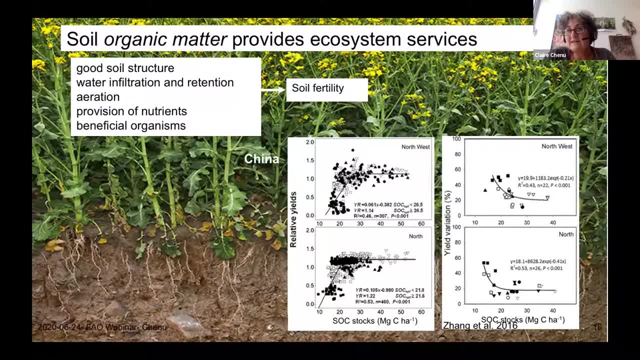 variation that is plotted against soil organic matter, soil organic carbon stocks. So it is actually yield stability that increases with soil organic carbon stocks. Soil organic carb matter and its main components, soil organic carbon, are important to food security yields and to their stability adaptation to climate change. 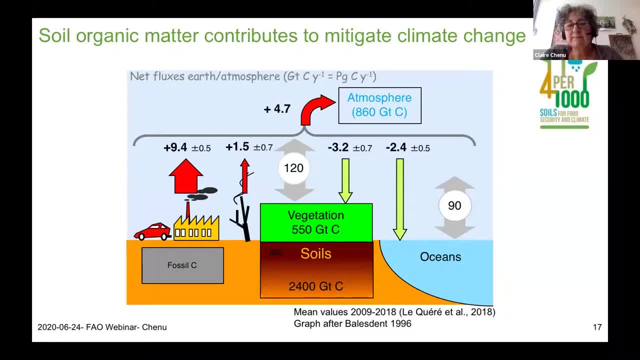 Soil. organic matter also contributes to mitigate climate change. There are huge carbon stores in the soil. There's more than two times as much carbon in the soils than there is in the atmosphere- And hence a very small variation of these carbon stores, even a variation of the carbon stores. 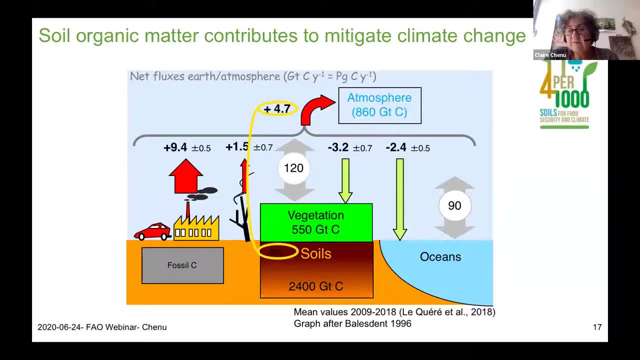 in the upper 40 centimeter of soils could have a strong impacts by increasing on the composition of the atmosphere, either increasing it or decreasing it, And this is the basis of the four per meal initiative: soils for food security and climate, An initiative that aims to promote the preservation. 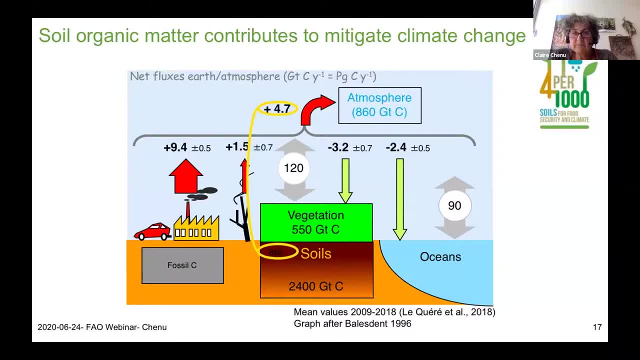 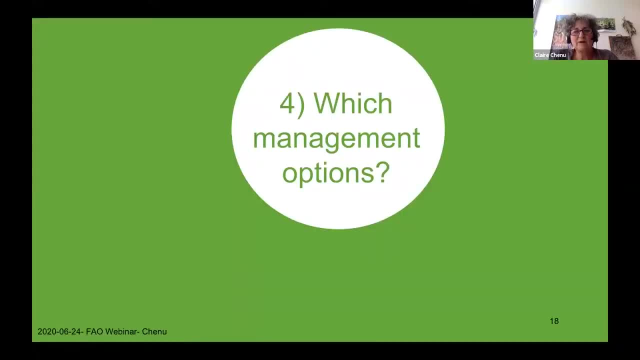 of soil carbon and the increase of soil carbon, in particular in agricultural soils, for food security and for climate. Okay, so soil organic matter is important. which management options to implement? Let me have drink a little bit of water. I will present you only two examples. 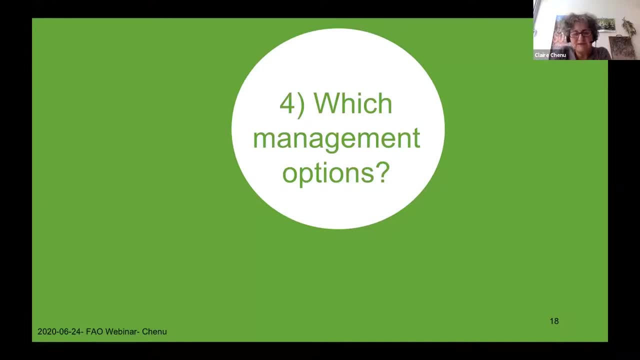 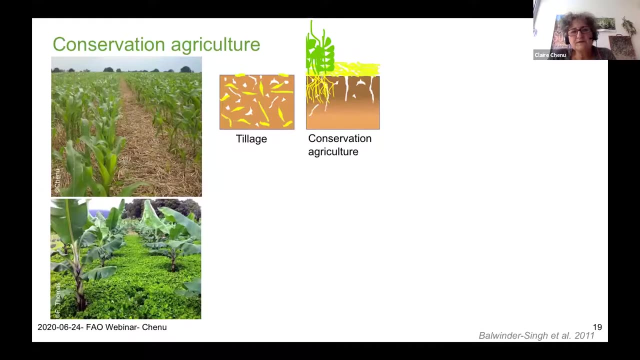 The next speech will develop much more than I will do Two examples of cropping systems. The first one is conservation agriculture. Conservation agriculture is reducing or suppressing tillage. Reducing or suppressing tillage, maintaining a permanent soil cover, either as a permanent soil cover or as a permanent soil cover. 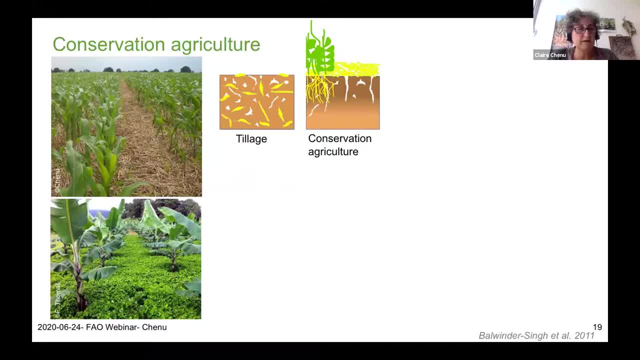 So this is the first example. It is the global that supports as a記得 job moles and as plants, and diversifying the rotation It has very important effects on sites that I tried to some to show partly On these graphs. 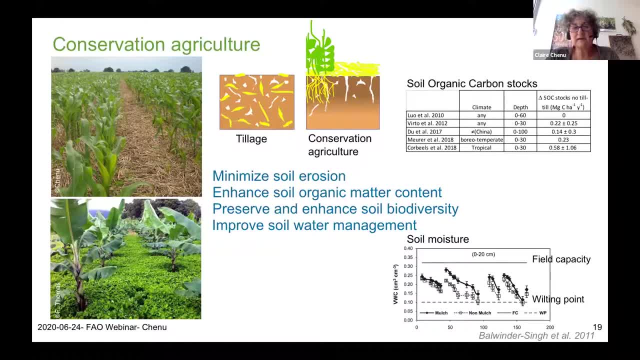 Minimize soil erosion. while it has been shown, and many studies show- that conservation agriculture decreases soil erosion, that it also enhances the soil organic matter content, with actually- and this is my upper table- very variable results depending on the depth considered. 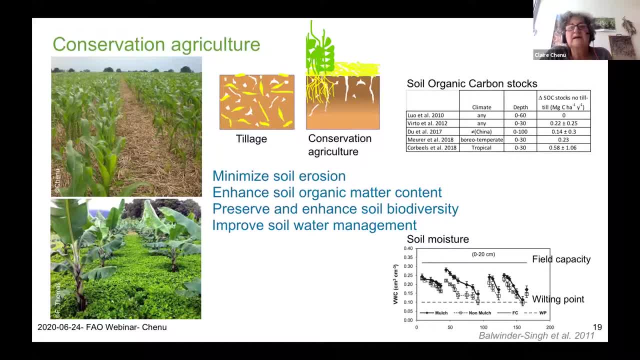 depending on the climate considered and effects. that are especially important when you have a cover crop that is living, that when you increase the inputs of organic matter to soil Conservation agriculture has been shown in many studies to preserve and enhance biodiversity and to improve soil water management. 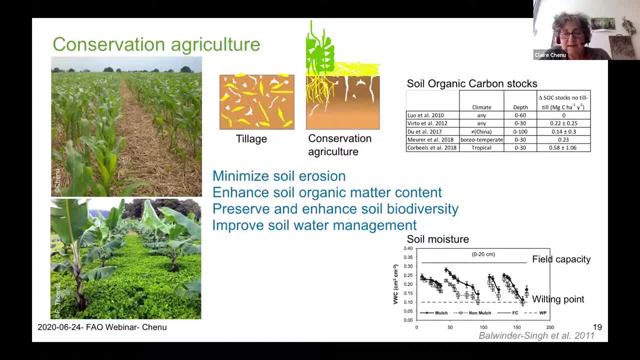 And here I took an example from rice crops in India where you can see. so I'm sorry if it's a bit complex, but you can see the X axis is time and the Y axis is the soil moisture. And you can see that the dots that are black 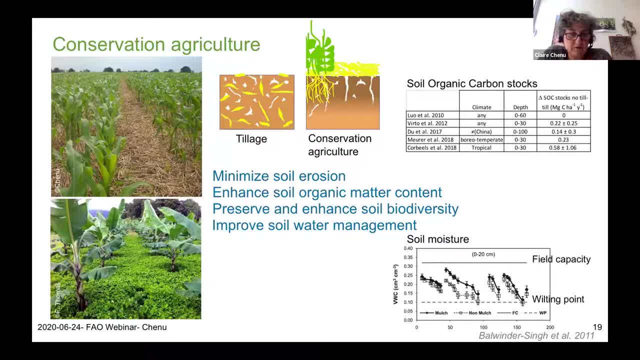 that correspond to the soil moisture and the X axis is the soil moisture. So in the situation with the mulch conservation agriculture, the soil moisture is always higher than it is in the reference plots without a mulch. So conservation, the presence of a mulch. 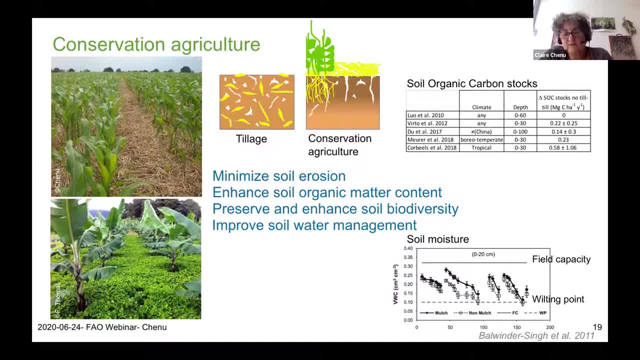 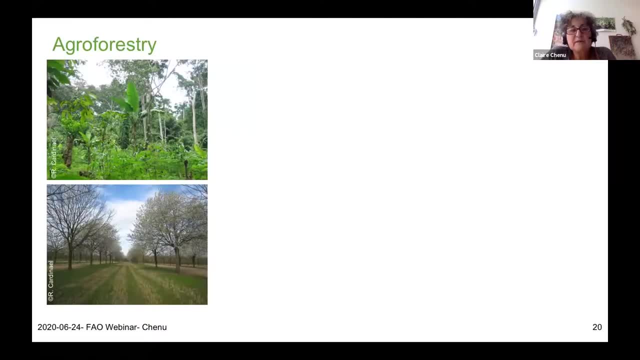 allows to preserve water and hence to better adapt to climate change. The second system I would like to take as an example is agroforestry. Again very extremely variable systems in different areas of the world. We just illustrated with two photographs, same approach. 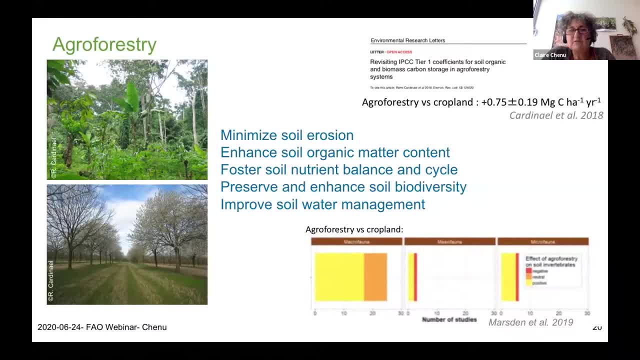 Well, agroforestry has been shown very efficient to minimize erosion, very efficiently to enhance soil organic matter content. And here my example is a recent paper where the IPCC coefficients for soil organic carbon storage were revisited And actually the numbers of these very recent meta-analysis. 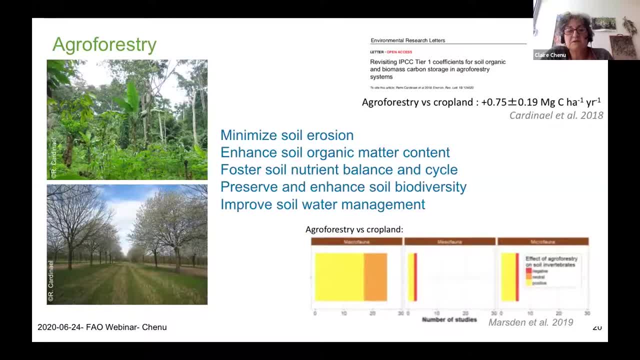 are quite high. So there's carbon storage in agroforestry in soils, not only in the trees, also in soils. Agroforestry has been shown to foster nutrient balance and cycle to preserve and enhance biodiversity and improve soil water management. 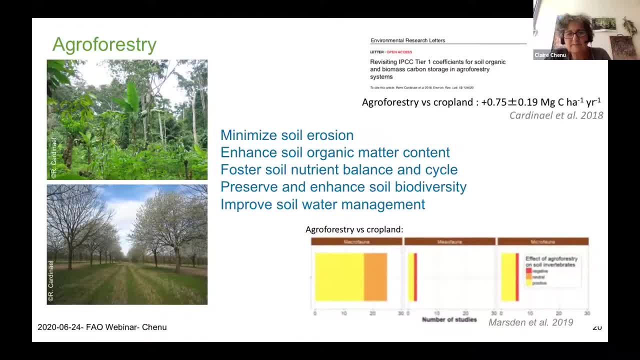 And here what I illustrate. I see that the quality of the graph is not that good. I'm sorry, is you have here? what is represented in this recent meta-analysis is the number of studies that quantified an effect of agroforestry. 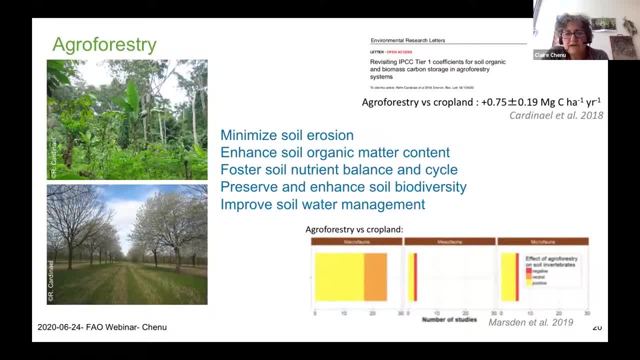 compared to cropland. on macro fauna- the first block, meso fauna and micro fauna- And the positive effects are in the papers showing. positive effects are in yellow, the neutral in orange and negative in black. You see that it's mostly positive effects. 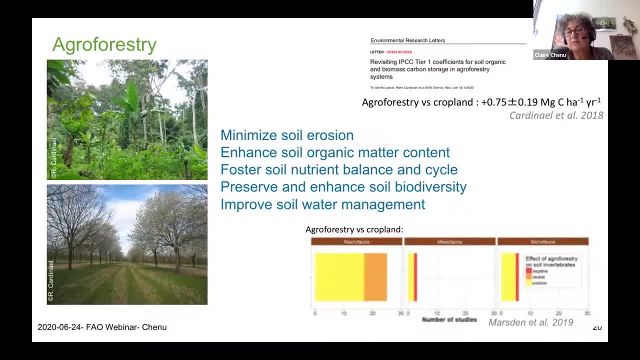 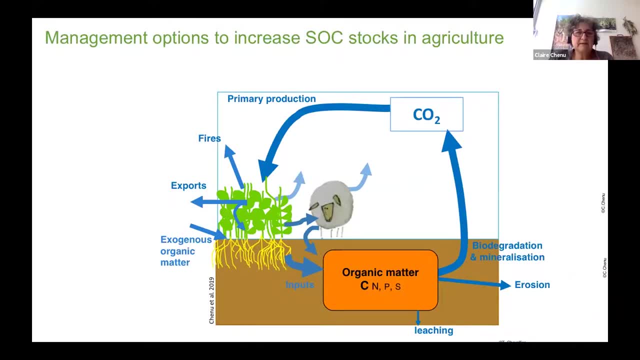 So agroforestry does preserve and enhance soil biodiversity in general. Now, if we focus again on soil organic matter and management options to increase soil organic carbon stocks in agriculture, there's actually a wide range of options that are available and that I will represent with photographs. 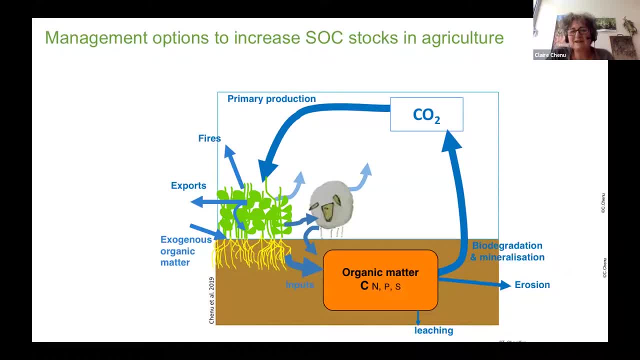 based on this simplified cycle of soil, organic carbon in agricultural soils, where you have the inputs and the outputs. First, primary production can be enhanced with cover crops, with greening or grassing the inter-rows in the vineyards or orchards. 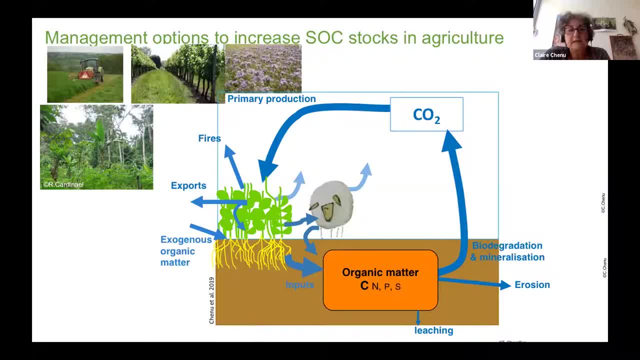 with temporary grasslands and with agroforestry, Fires can be canceled- and this is an issue in several countries. Exports can be reduced and crop residues returned back to soil and exogenous organic matter such as compost, manure or biochar, added to soil. 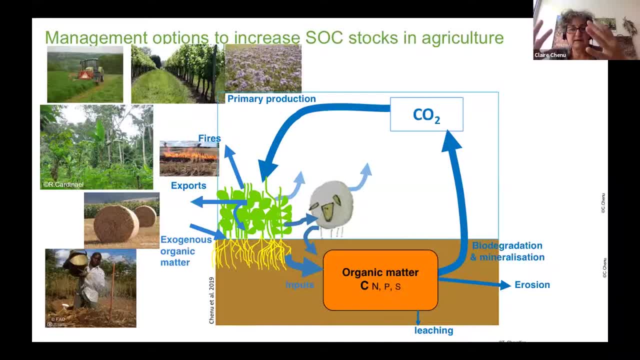 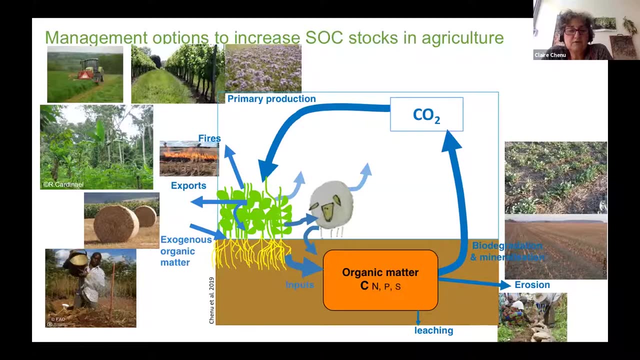 These will increase the inputs to soil and then increase the soil. organic matter stores And other practices can reduce the losses by reducing erosion. so small infrastructures reducing erosion or conservation agriculture to reduce erosion and reduce biodegradation rates of the organic matter. 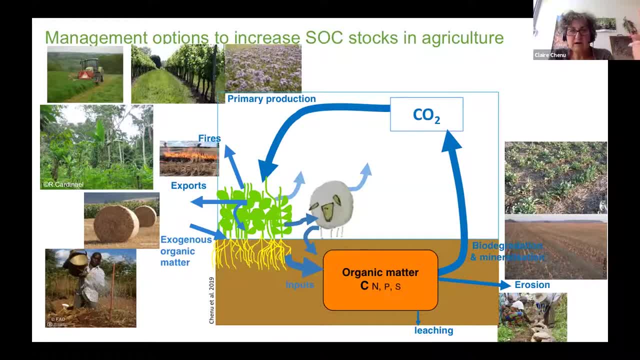 So different management options, and what really comes out very clearly from the literature now is: what is most efficient is to increase the inputs to soils rather than try to decrease the outputs from soil. Yeah, and agroforestrials. Well, you may have guessed that I'm working. 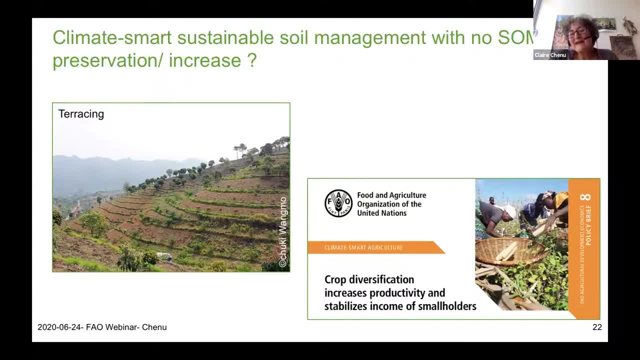 on soil organic matter, and you may have a question that is well, can you do climate smart, sustainable soil management with no major input, no major level going through soil organic matter? Well, I think that, yes, I think that yes, for example, terracing: 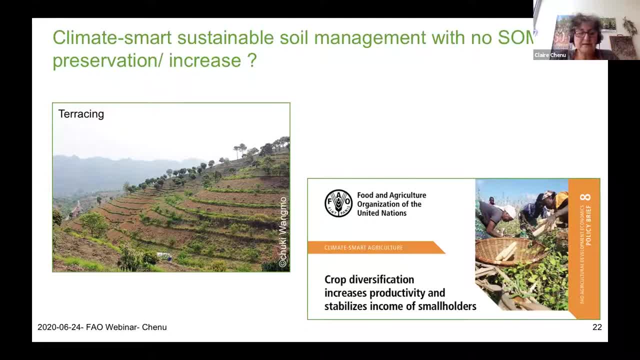 will reduce strongly erosion, but there's no direct effect on soil organic matter. Well, reduce erosion but reduce soil organic matter. reduce erosion might help to preserve organic matter, at least preserve it in the field. And another lever that is promoted by FAO. 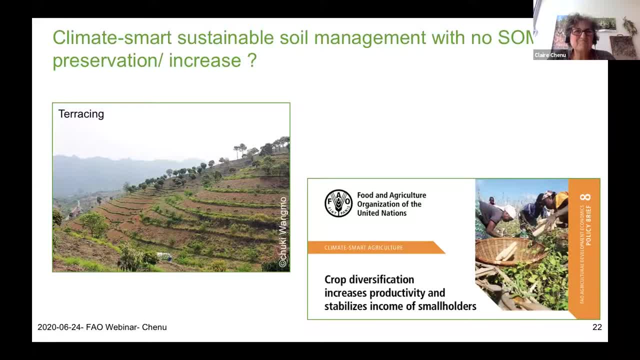 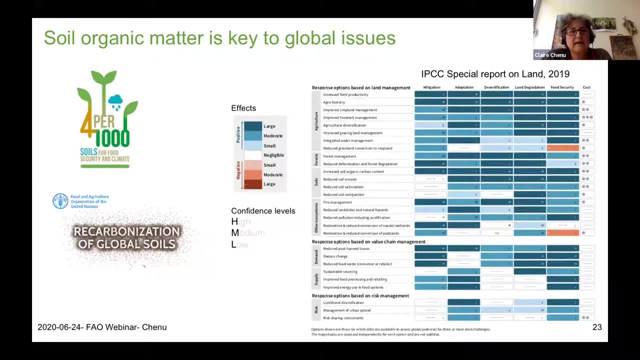 is the crop diversification? It has. no, there's no straightforward effect on soil organic matter, but it has been shown to increase productivity and to stabilize income of small holders in a climate change context. So organic matter is not the only lever, it's an important one. 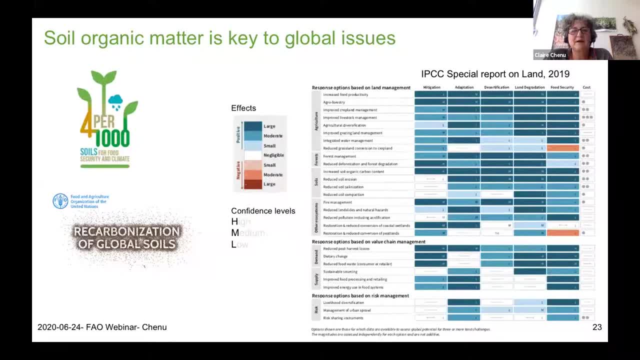 It is key to global issues. Again, here you have a report, a graph that I took from this IPCC special report on land, where you see the columns correspond to the global challenges they addressed: mitigation, adaptation, desertification, land degradation and food security. 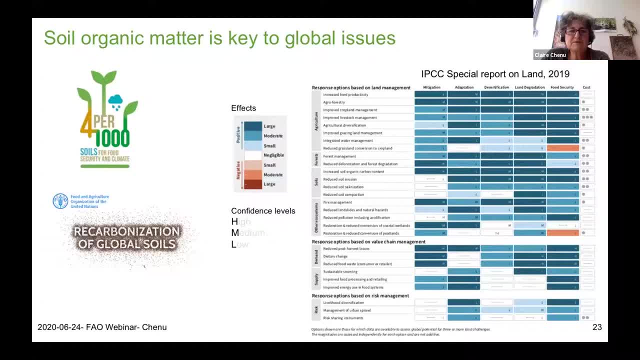 And the lines correspond to the different response options based on land management. they considered, And I would like you to see that one management options option- increased soil organic carbon content has- is considered to have a high, a large effect on all of these challenges. 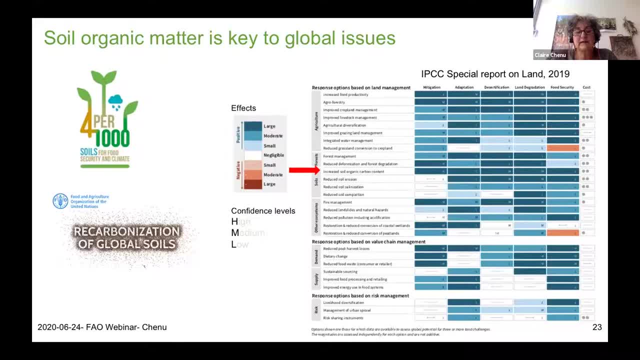 So it's a good solution, And this explains the occurrence with the existence of the FAO project Recarbonization of Global Soils- that started sometime well just, I guess, one year ago- And of the Four Per Mill Initiative. 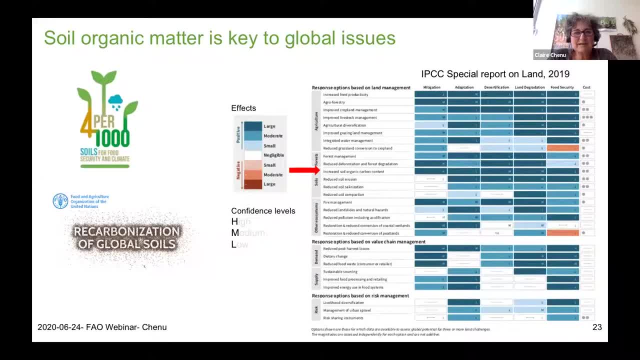 And the Four Per Mill Initiative. so it's a multi-stakeholder initiative and they are essentially focused on promoting and fostering the input of land management options and agricultural practices that help to preserve and increase soil organic matter, by addressing policy makers and addressing farmers and the whole agricultural sector. 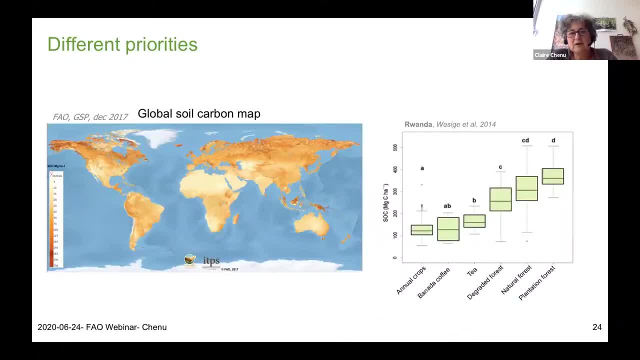 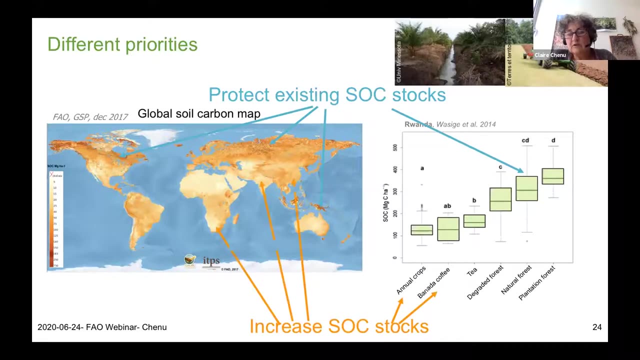 Of course, depending on the area of the world, there are different priorities. In Northern areas, for example, or in forest, the priority is to protect existing soil organic carbon stocks, While in other areas, where the contents are poor and where it's a problem in soil fertility. 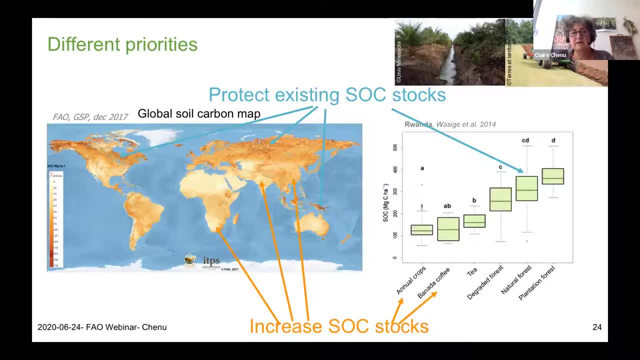 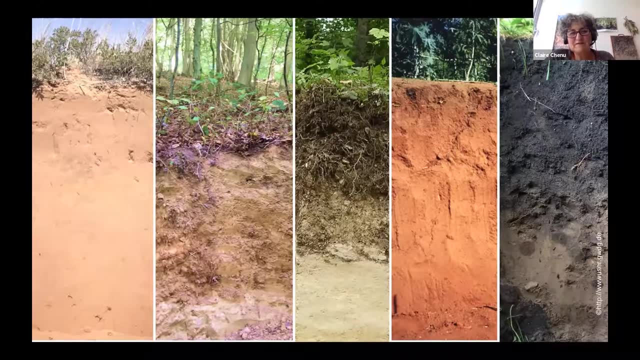 there the priority is to try to increase from the level at present. And also I would like to say that soils- with this, these photographs, that soils are extremely diverse. So management options have to be tackled, have to be adjusted to the soil type. 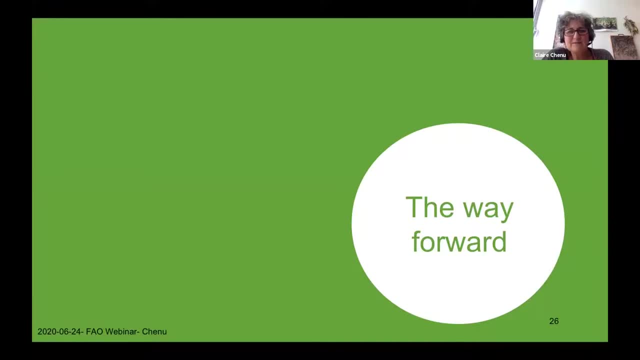 We are close to the end of my talk now And I would like. the way forward is a complex way where we need more knowledge. We need monitoring, verification systems for soil quality, for soil health, for the practices, for the management options. 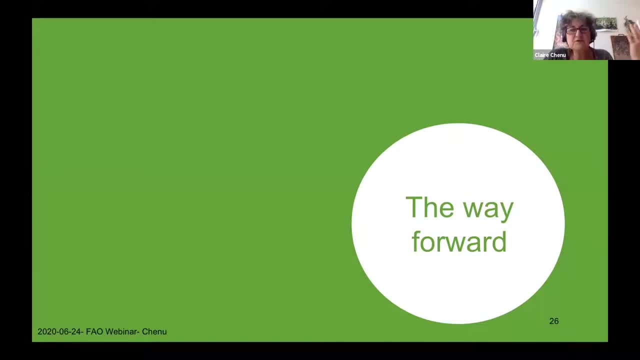 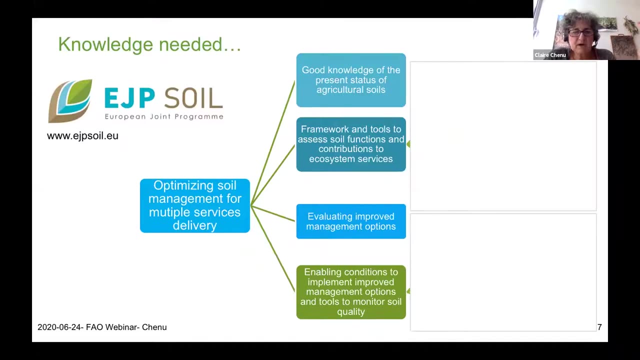 And we need enabling conditions to implement those climate smart, sustainable soil management options. I would like to give you one example, In fact one example, and it is- I would say it's- a working document. So, in this European joint program, 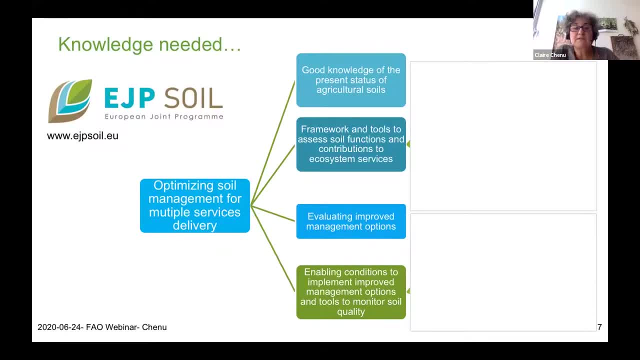 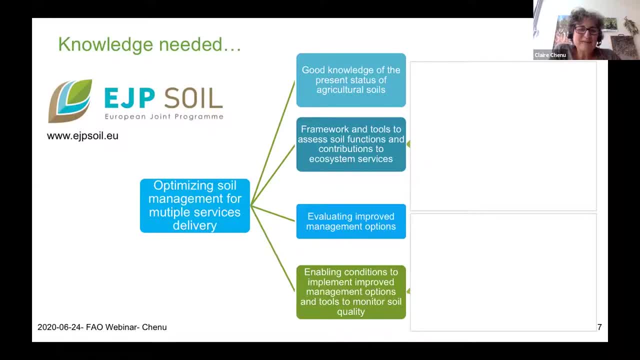 to provide the knowledge, to improve the knowledge, to develop climate smart, sustainable soil management And, for example, regarding the knowledge needed: well, the knowledge needed to optimize soil management for multiple services delivery, which we I covered today. What you need, we think, is a good knowledge. 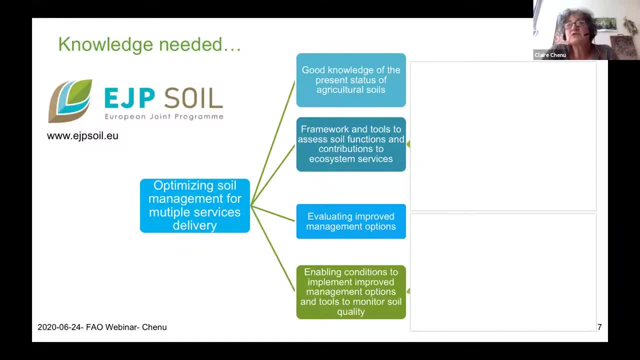 of the present status of agricultural soil, So soil information is extremely important there. You need a framework and tools to assess soil functions and their contributions to ecosystem services, And these can be go to identifying developing indicators for soil quality and ecosystem services. 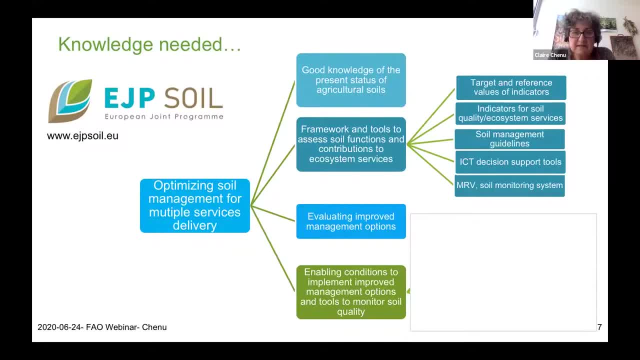 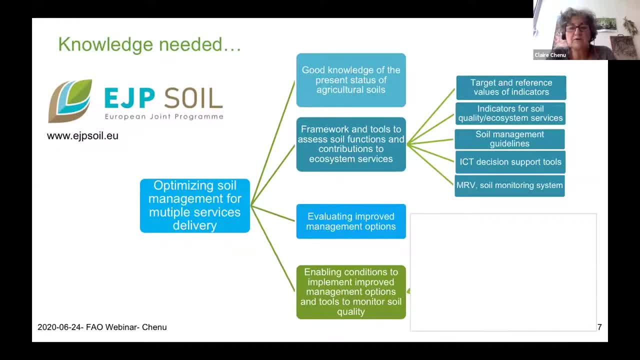 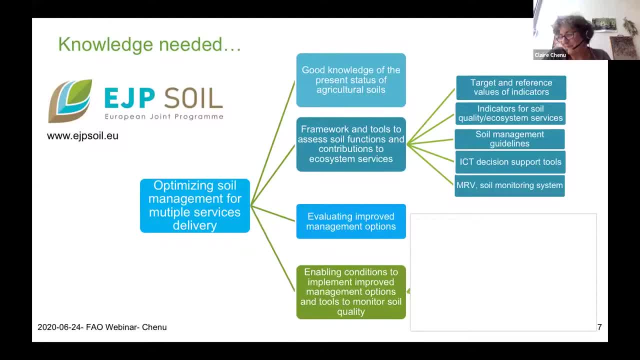 well, the climate smart, sustainable soil management options. well, and the following talk will develop also on this topic and show you two examples and enabling conditions to implement these improved soil management options And for example- well, this is not a complete list, this is examples- 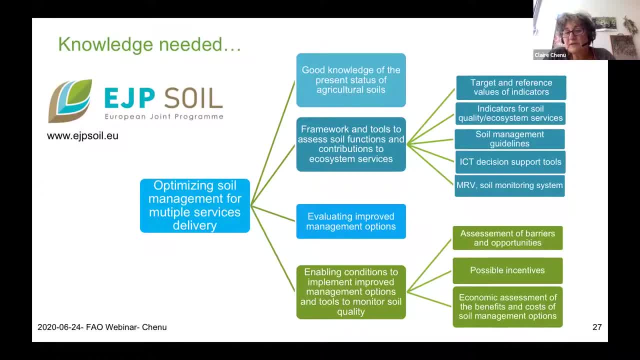 We think that we need an assessment of barriers and opportunities. we need to examine, maybe to propose, possible incentives and to do, for example, the economic assessments of the benefits and costs of the soil management options. So research cannot be only biophysical. 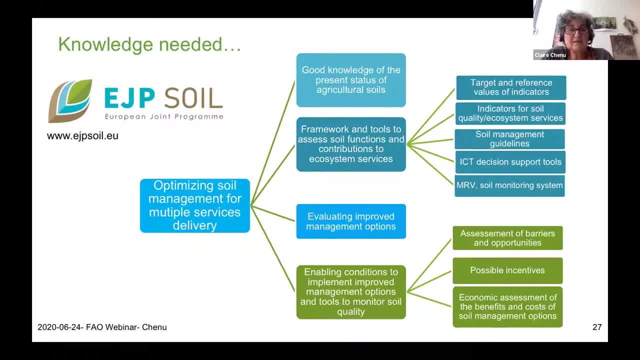 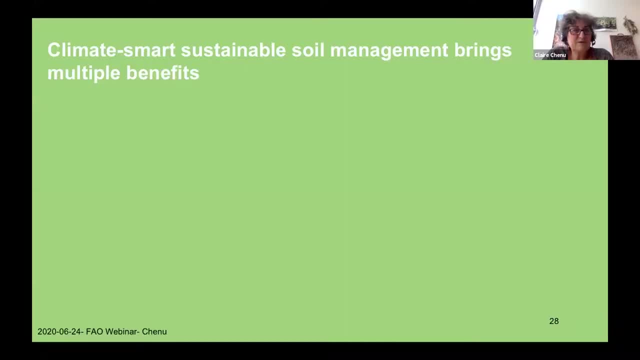 research has also to have political, legislative, social and economic dimensions. On this I will conclude. So climate smart, sustainable soil management brings multiple benefits. I think that our ecosystem services delivery, climate change adaptation and mitigation, reducing degradation and restoring soils and land. 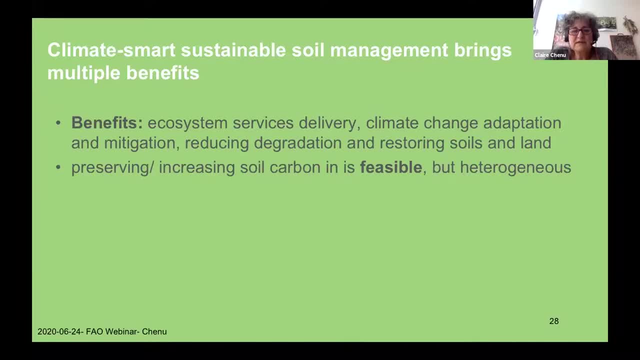 One component of this is soil organic matter, and preserving and increasing soil organic carbon is feasible but extremely heterogeneous. has to be spatially differentiated. Solutions have to be achieved locally and they have to be managed. they have to be devised and implemented locally. 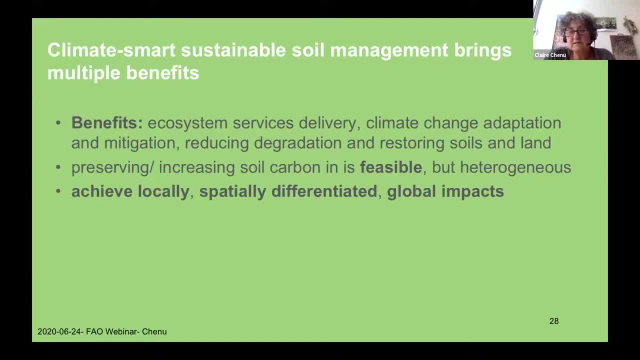 They have to be spatially differentiated. The contexts are extremely different, but they have global impacts. global impacts on nitrogen deposition, on biodiversity, on erosion rate and particles in the air and, of course, on the composition of our atmosphere in terms of greenhouse gases. 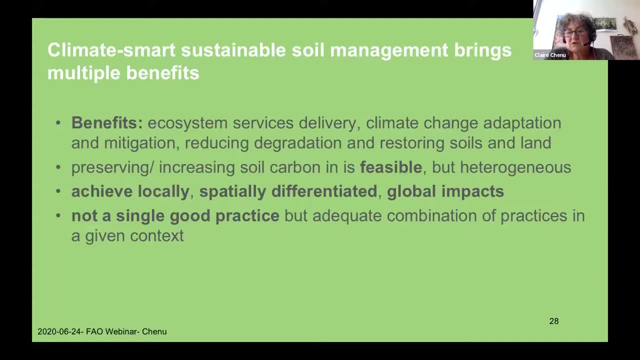 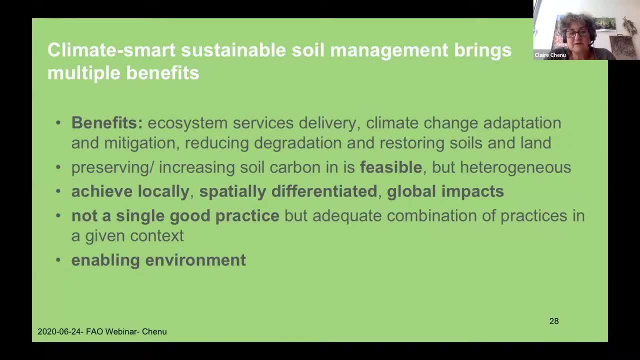 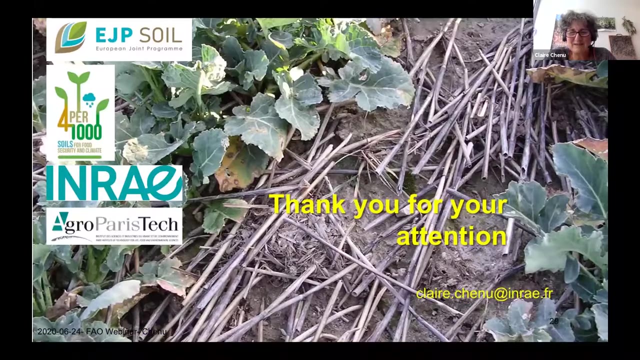 An enabling environment is of utmost importance, otherwise there's no transfer from knowledge to real life. And what- oh, I erased the S- a systems perspective is needed to tackle all these, And on that I would like to thank you for your attention. 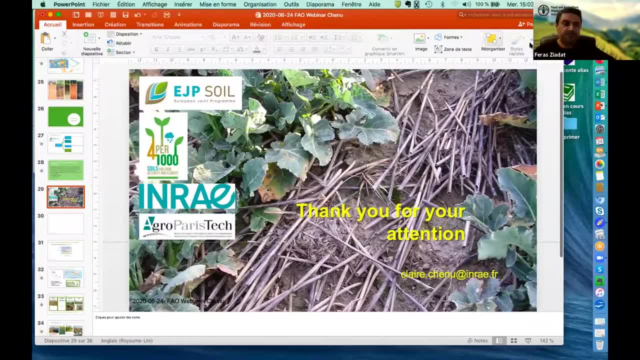 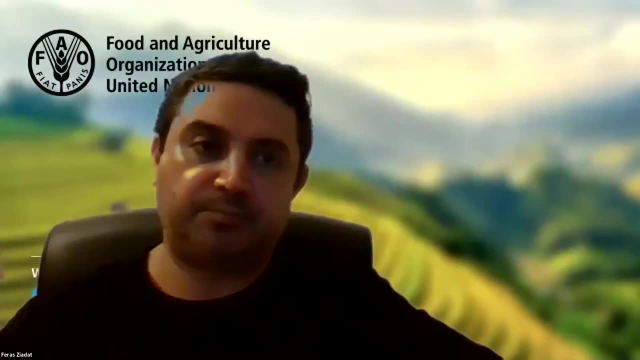 Thank you, Claire. Thank you very much for the presentation. We have some questions in the question and answer and I would probably prefer to do the other presentation because there are some questions that might be answered from the second presentation and then we will talk. 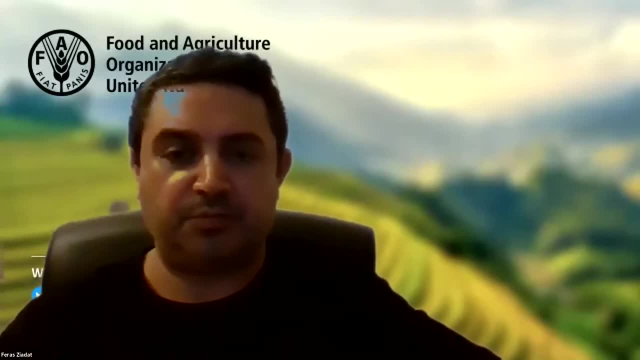 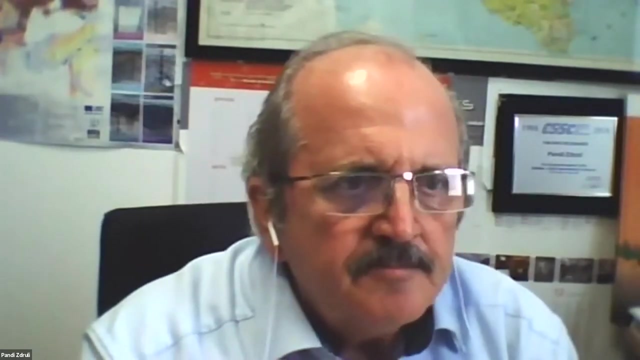 come to some questions from the chat or we open for some questions from the participants. For now, I would like to move to Professor Pandis Dolly from CM Barry to give his presentation on this topic. Thank you, Okay, Thank you. Thank you very much, Farah. Let me share my screen first. 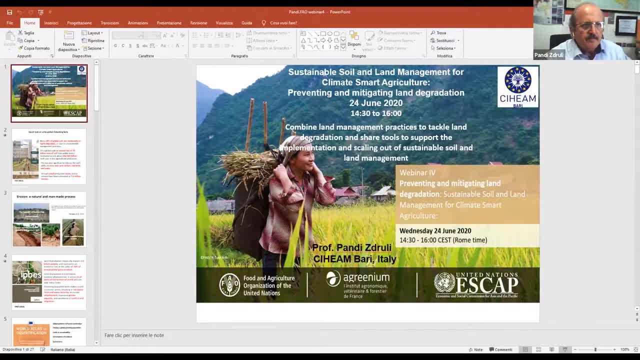 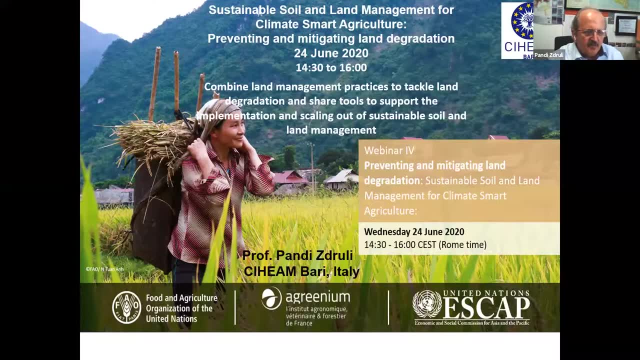 Okay, Okay. So good morning, good afternoon, good evening, wherever you are. In about 20 minutes I will try to give you some feedback on how we could combine these land management practices to tackle land degradation, and then what could be the next step. 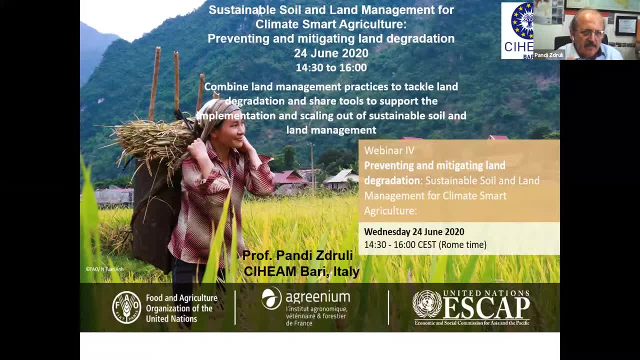 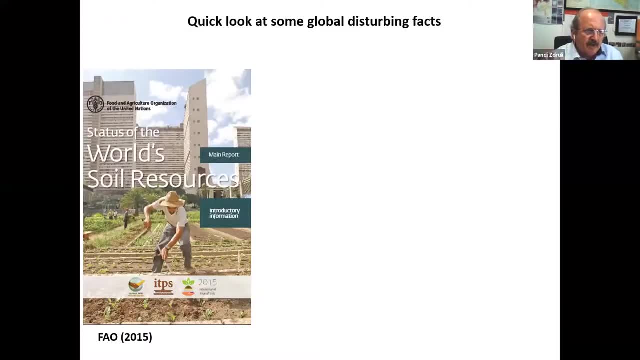 how to outscale them, make them available to other people who may be not aware. Now, as also Claire mentioned, we we have some disturbing facts in terms of land degradation. This report, published in 2015, pointed out a number of things that are ongoing. like Claire mentioned, 33% of the global soil are 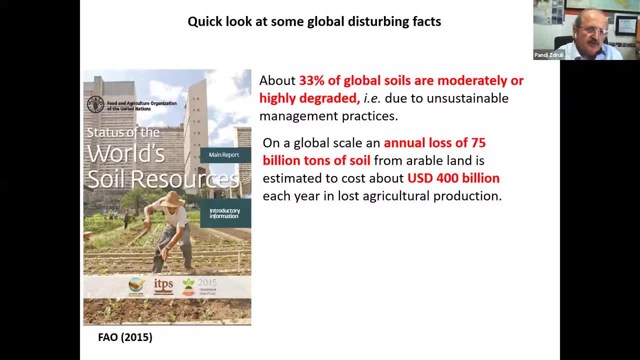 moderately or highly degraded, and mostly that is due to unsustainable management practices. We lose on a global scale annually about 75 billion tons of oil and if you convert them to how much it costs, we talking about 400 billion US dollars each year lost in agriculture production. 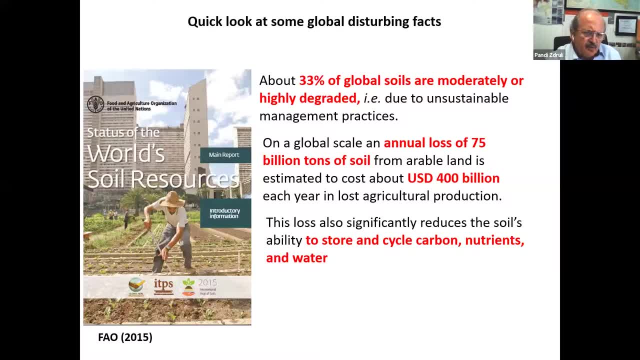 And then we also significantly this reduces the ability of the soil to store carbon. we heard how much important is this- organic matter, for example, and nutrients and water- and you can also try to figure it out. how much is damaged, for example, from erosion and we. 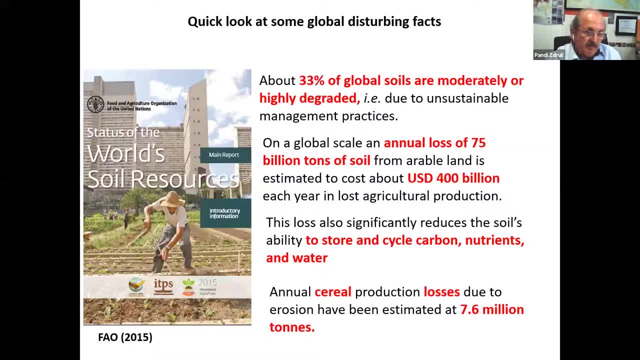 estimate that losses to that report are about 7.3%. Fascinating, Very interesting. Thank you, Farah. Thank you so much, Farah. Thank you. 6 million tons a year. So erosion is a problem and many, many other problems. 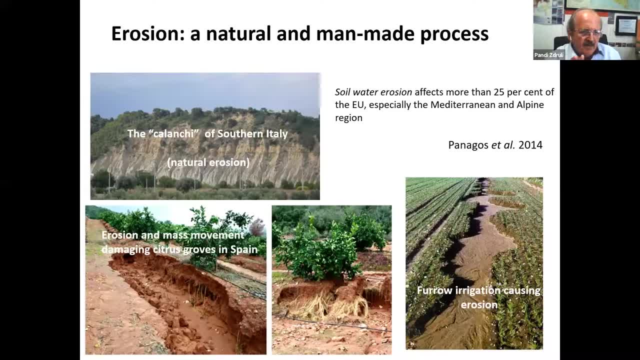 like that. This is the only one slide on bad things that I will show, and I'm showing this for a reason: because erosion affects every place on earth. It's also an HR process, by the way, and it affects about 35% of the European Union, So don't think it is only an issue outside. 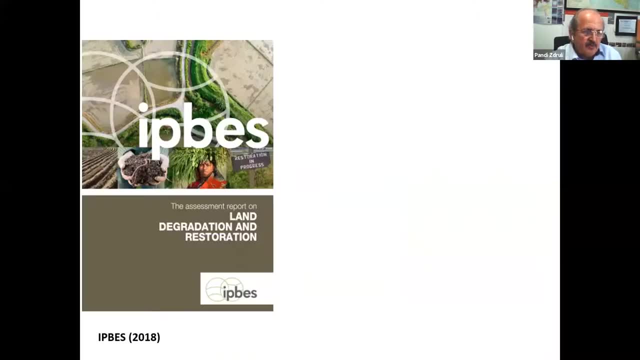 developed countries and sometimes it's due to unsustainable land management practices. This report- and Claire mentioned it as well- of IPBS came out in 2018 and again some very disturbing facts like: land degradation impacts 3.2 billion people and represent an economic loss about 10% of the annual GDP. It is a 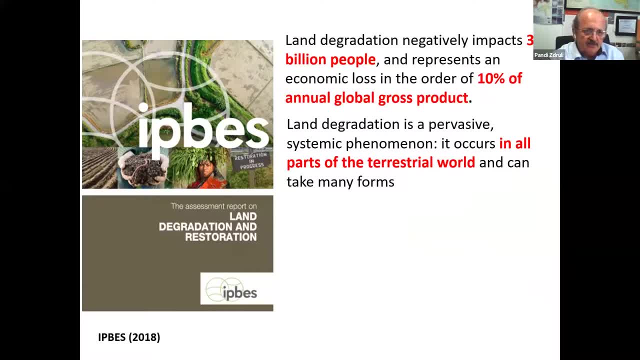 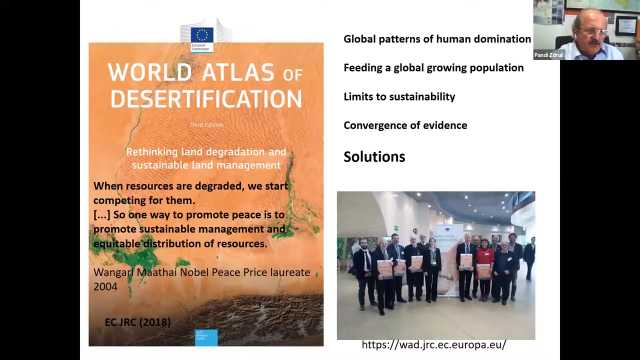 pervasive systemic phenomenon in, of course, all parts of the world- and I mentioned Europe in that regard- And restoring degraded lands makes sound economic sense because it could result in increased food and water security, employment, gender equality and could avoid conflict and migration. Now, in 2018, was published also the World. 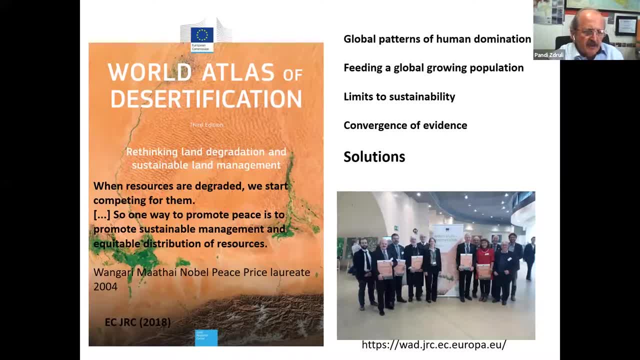 Atlas of Desertification. That was the third edition. I gladly participated in developing this product and it opens with a very interesting phase. It is a very interesting phase and it opens with a very interesting phase. It is a very interesting phase and it opens with a very interesting phase. 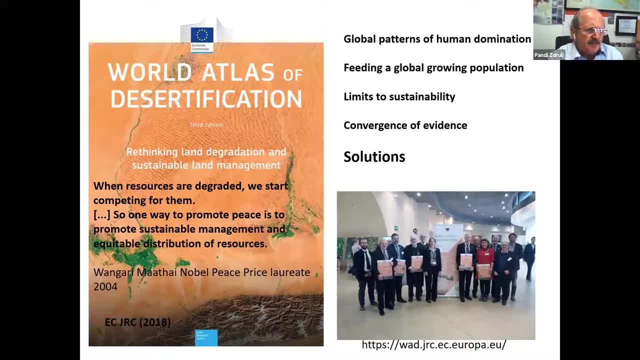 Rethinking land degradation and sustainable land management. and there is a saying by the Mangari Mahaya- Nobel Peace Prize laureate, I guess from Kenya- and she says: when resources are degraded, we start competing for them. So one way to promote peace is to promote sustainable management and equitable distribution. 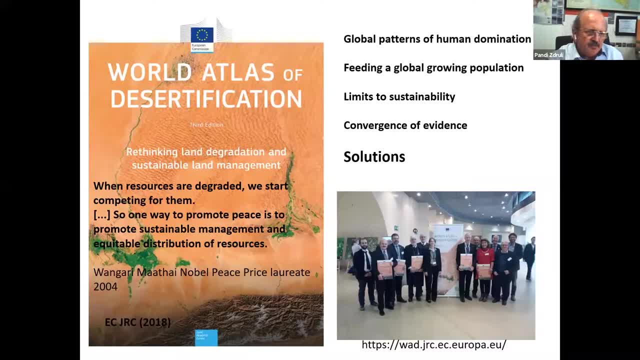 By the way, I have given the links and the presentation will be sent to you so you can look in and link and then find out more. This atlas, it's a mixture of maps as well as text, and I will focus mostly on solutions. 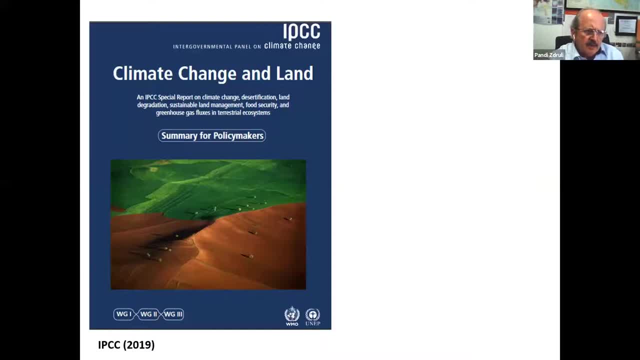 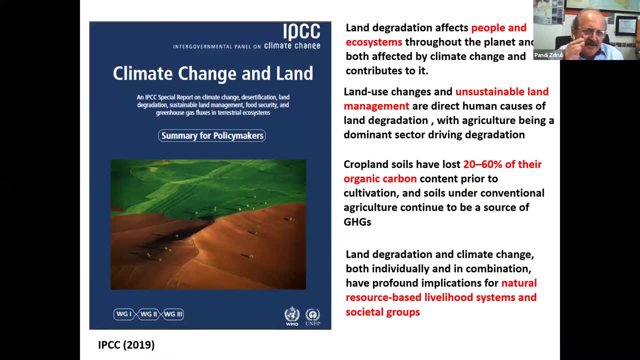 Now, Claire mentioned this, but this is also quite a good report: important report of IPCC on climate change and land and a summary for policymaker, And again a number of disturbing factors coming out, Like, for example, if you see this one here: 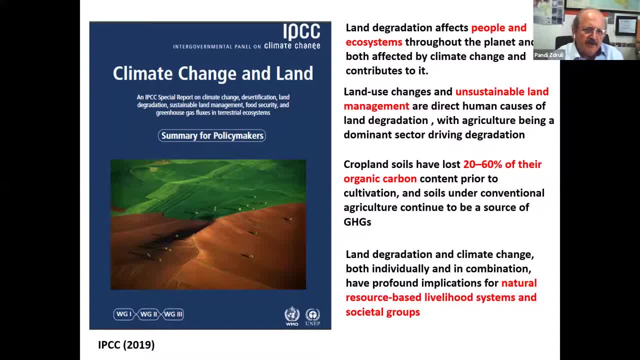 cropland soils, since Claire spoke about organic carbon, have lost about 20 to 60% of their organic carbon content prior to cultivation, And soils under conventional agriculture continue to be a source rather than the solution, And we have to change this. 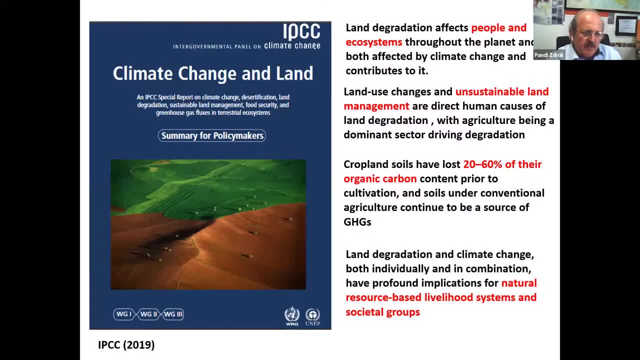 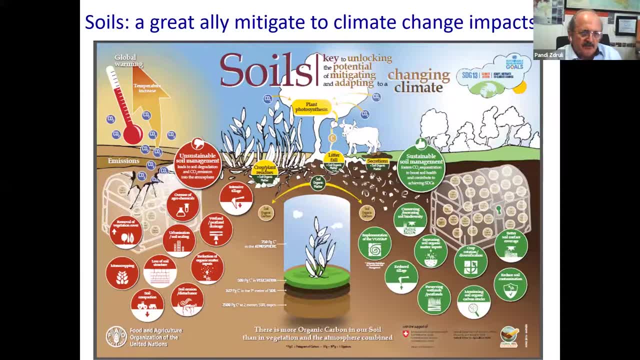 We have to make the soil as a solution to this problem. So we have a great ally, which is soil to mitigate and probably also to adapt to climate change And what you see on the left side. this was developed, by the way, by the Global Soil Partnership. 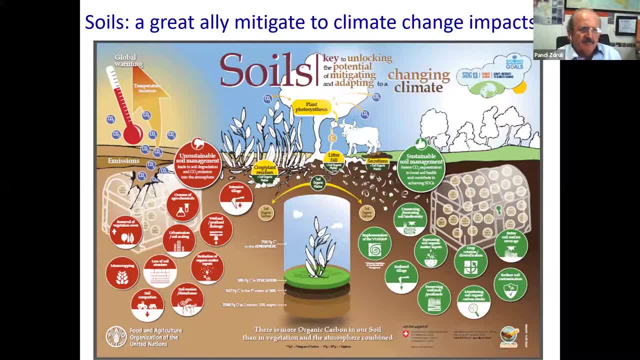 2015 was the International Year of Soil. So many of these came out at that time And you see, on the left side, on what is on the red is all the bad things that we can do. Through unsustainable soil management, we can increase erosion. we can accelerate erosion. 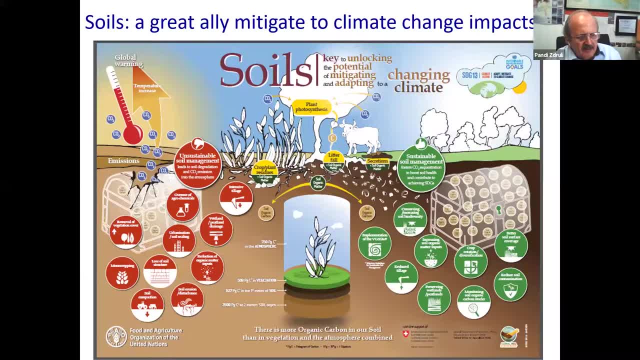 we can compact the soil by having machinery And what we do is that we release the carbon up into the atmosphere And accelerate the climate change. On the right side are the good things you see on the green, And those could be achieved by sustainable soil management. 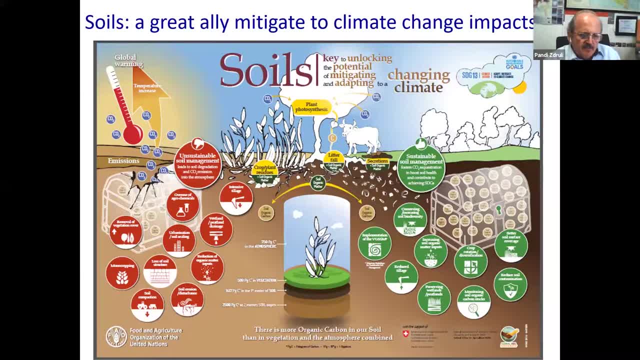 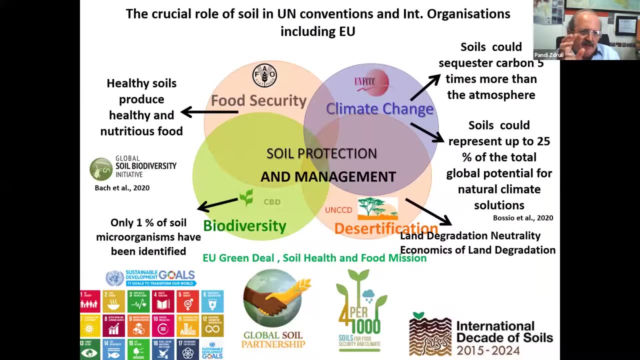 And I will show you with practical example from also my personal experience from some of the projects that have somehow achieved all what it is given. on this right side of the slide Now, soil protection and management stays at the heart, at least for the three US. 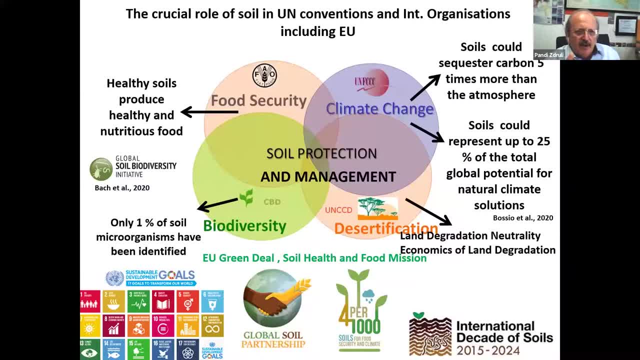 the UN convention We heard a lot about how important is the soil carbon sequestration for climate change, And then the soils on themselves represent up to 25% of the total global potential for nature climate solution. That was a paper that came out. 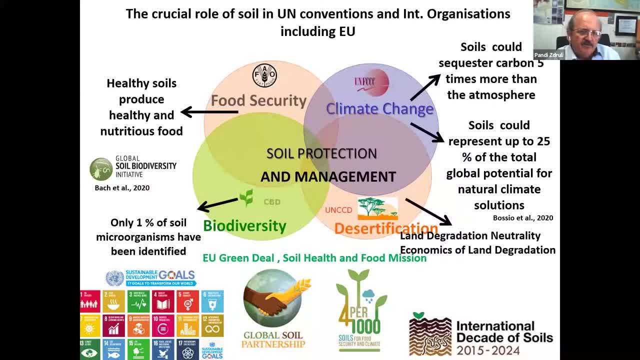 It say, the 60% out of 25 can come out if we implement sustainable land management practices, UNCCD, the Convention to Combat Desertification, involved in land degradation neutrality, And there is also economic of land degradation initiative, And so is the Convention on Biodiversity. 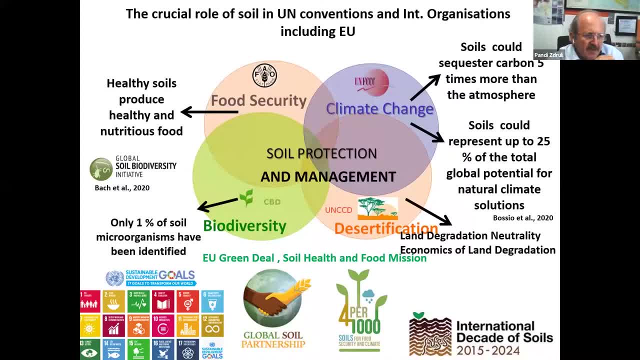 And we only know 1% of all the billions of microorganisms that are into the soil. That's why, also, there is a global soil biodiversity initiative. We have in Europe now the EU Green Deal, which is looking after all these issues, And there is also a soil health and food mission. 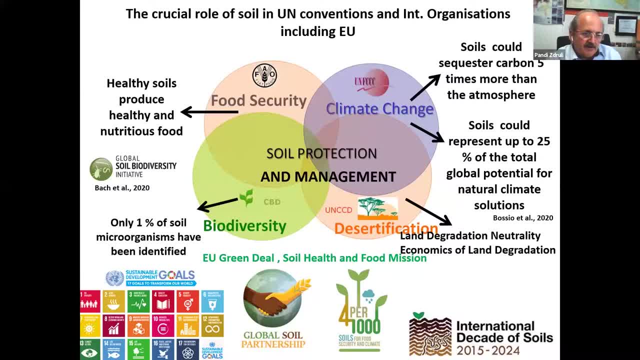 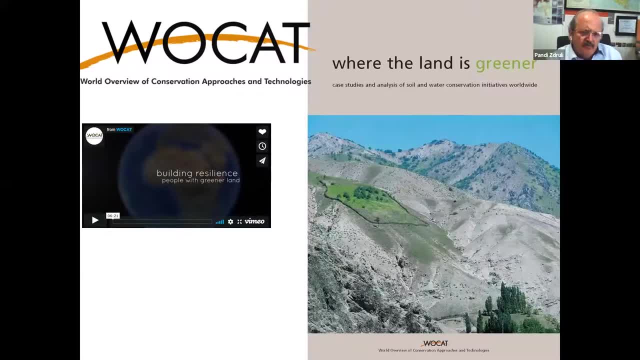 which is trying to put all the targets for the next seven year period in the European Union. So where to find this information? Now? I can't start this by mentioning, without forgetting, WACAP. WACAP is the World Overview of Conservation Approaches. 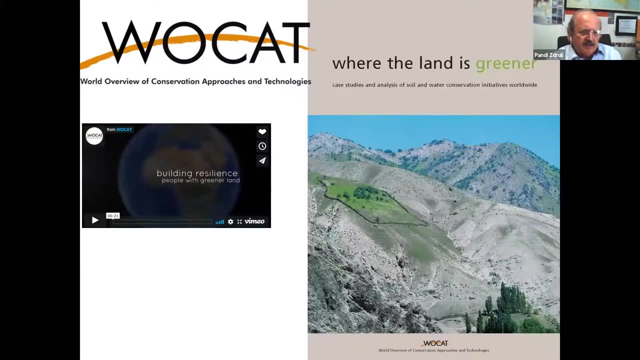 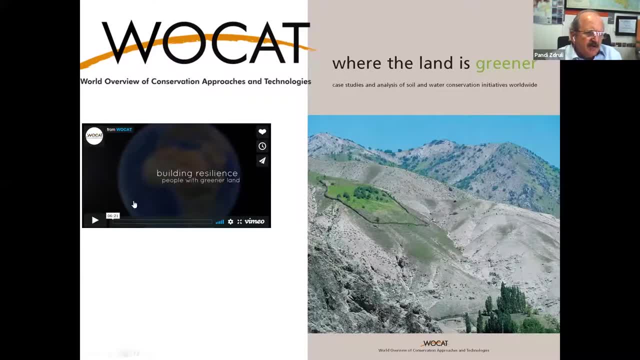 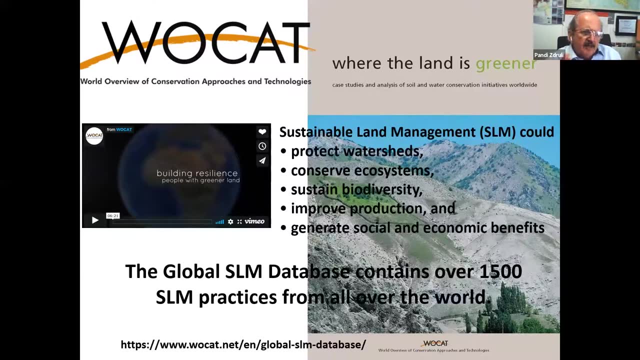 it was a big show Here. it is also a nice video. We don't have the time, but you can click and learn more. So practically the sustainable land management can have a set of of of of good things that can derive out of that. 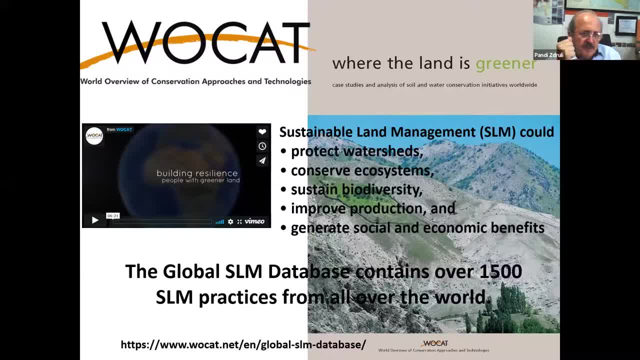 Like you can protect the watershed, You can conserve the ecosystem, sustained biodiversity, improved production and generate social and economic benefits. that are more than a thousand, five hundred of these practices from all over the world into the database of oil company. That's interest the world. That is big measure with that. 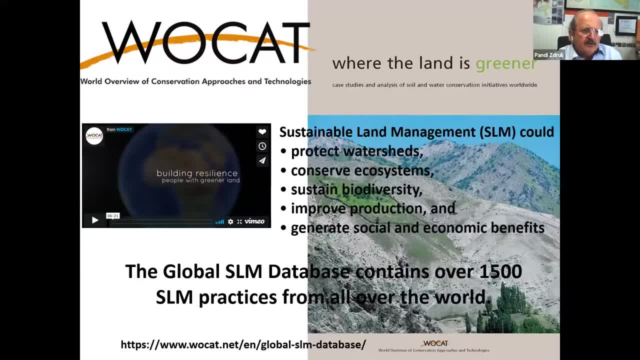 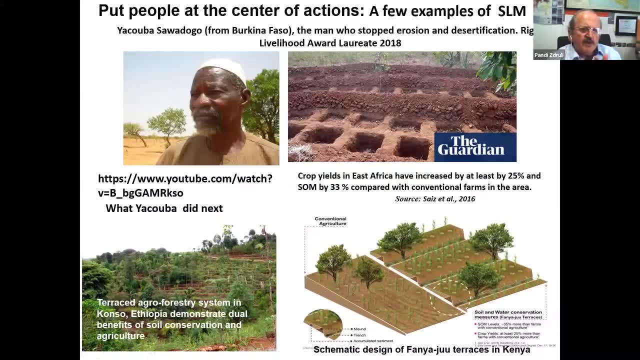 feel free, go there and you will learn a lot more. so how to do this? i think we have to put people at the center of the actions, because not what i showed are the big conventions and the legislation and the framework, but at the end of the day, there are the people on the ground who have to make. 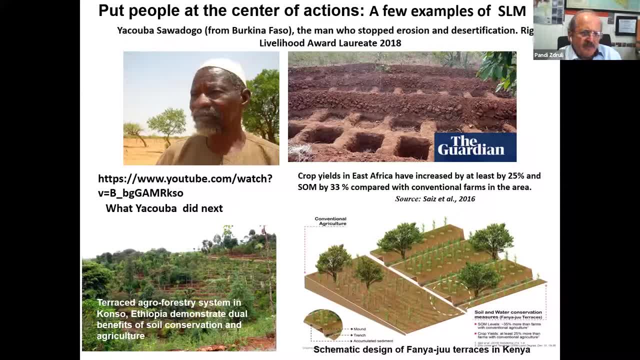 this change, so that's why i'll try to do with some examples. it's like a picture can speak more than a thousand words. this man- for those of my age probably know it, but maybe the youngers that are attending us maybe don't know- is yakuba sabadoga, from burkina faso. 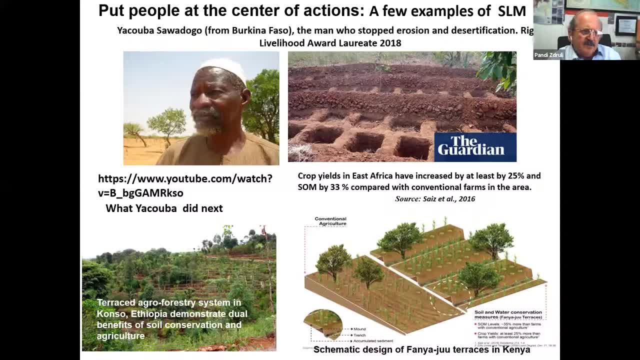 he was called the man who stopped erosion and desertification. he, he, he was kind of as a star invited in the cops of uncd. there is also this video here what yakuba did next, so how he showed. he was in the guardian, that is the, the newspaper in the uk, so practically in. 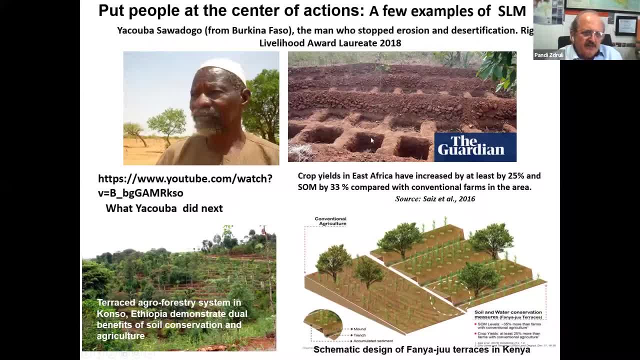 design, it's how they call it. he planted these trees and he put it mulches and he put his organic manure, he put his fingers, he created an agroforestry- man-made system. the first one, uh claire, mentioned the good effects that the agroforestry can have, and there are examples like that one. 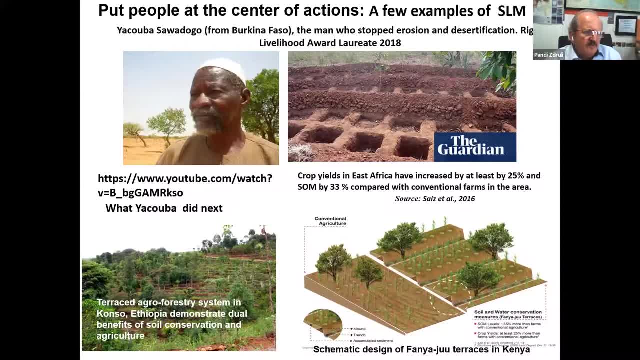 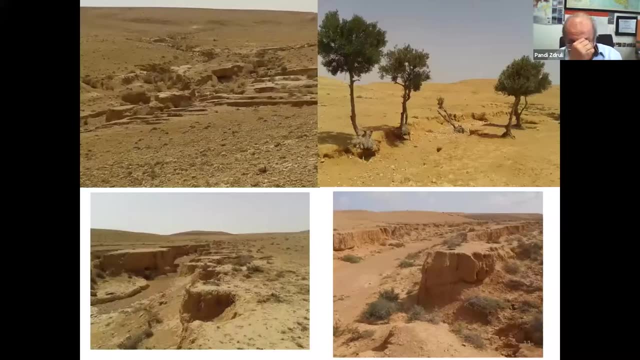 for example, in consul in ethiopia, we have dual benefits for soil conservation and agricultural production, or the terraces, but we are you terraces in kenya, by the way, we are going to have both countries soon a project and we try to implement this practice at a larger scale. uh, i 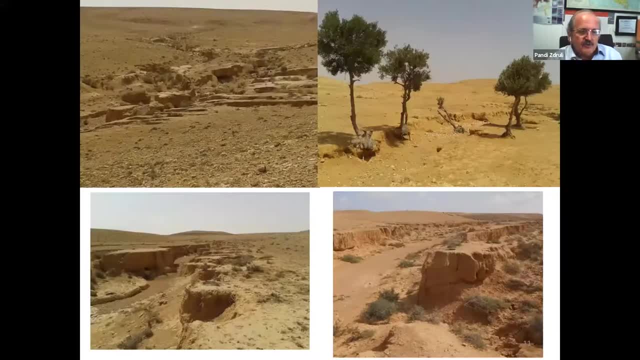 give you another example, and this is quite interesting. if you see these pictures, you probably think that we are somewhere, i don't know- moon, or, or mars, or. this is in the matruh region in the western desert of egypt, and you can see this galley erosion. 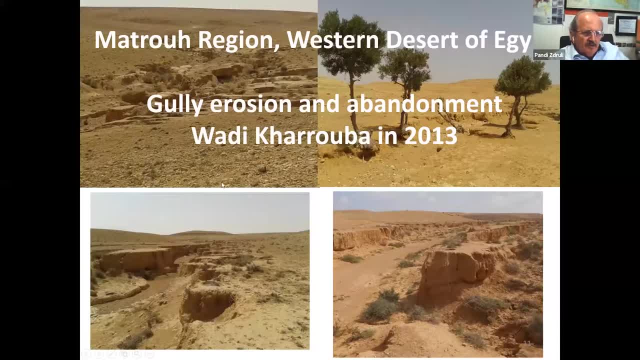 these areas are abundant. wadi- in arabic, by the way, mean watershed or a basin, so it's not something you can find in the desert, but you can see the galley erosion in the western desert and this is a very important part of the project we started. there was like that in 2013 and we 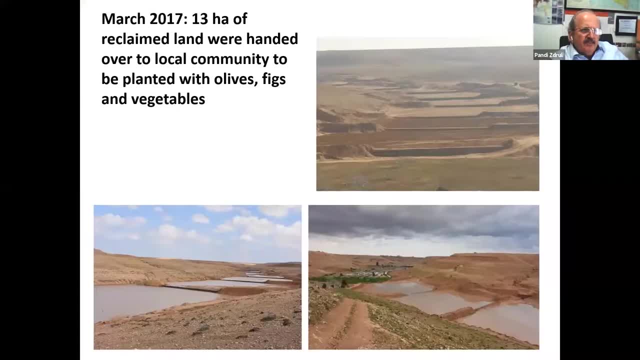 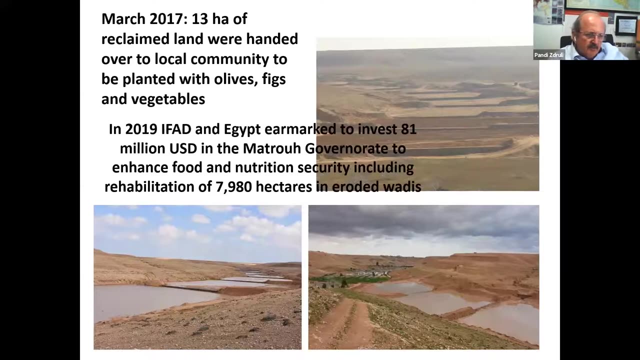 started there. a rural development project was coordinated by our institute in bari and was funded by the italian corporation, and we collaborated strongly with the desert research center in egypt. and that's what it became, like this in 2017: 13 hectares over reclaimed, and it's 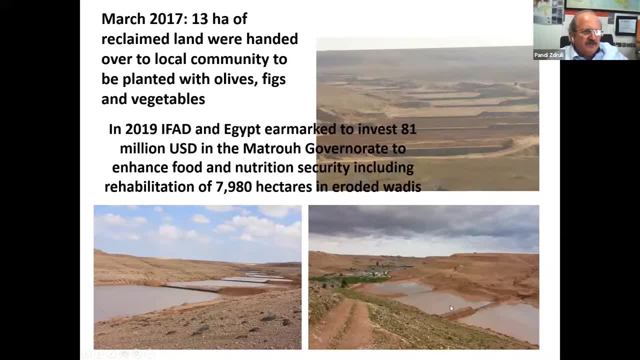 over to the bedouin communities where they grow olives and pigs and vegetables. and guess what it you? a little bit more on the water harvesting and if and egypt decided to invest more money and to rehabilitate something like 8 000 hectares of this aerobic valley, i hope they they are doing. 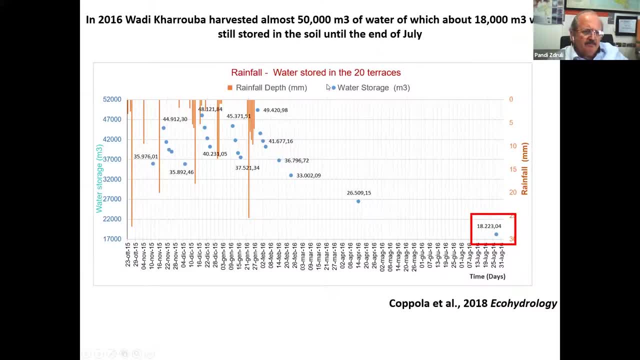 it uh. so we publish even a paper and- and very briefly i will go that, if you see, here we are almost at the end of uh july, also very dry season. here in train that 2016 actually was a bit wet year, but still due to this intervention, we were able to store almost 18 000 uh cubic meter of 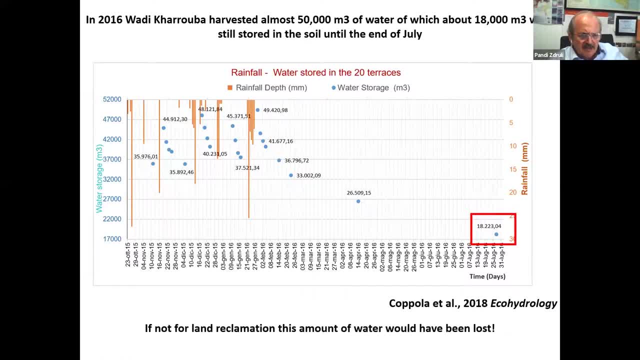 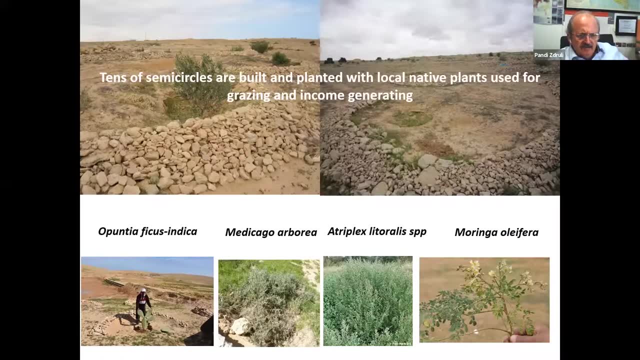 water that otherwise those would have been lost if not for this intervention that we made. so you do, but you don't need to look only at the flat layer. by the way, interventions like this i know from literature and peer review papers that i i also reviewed- are implemented also in 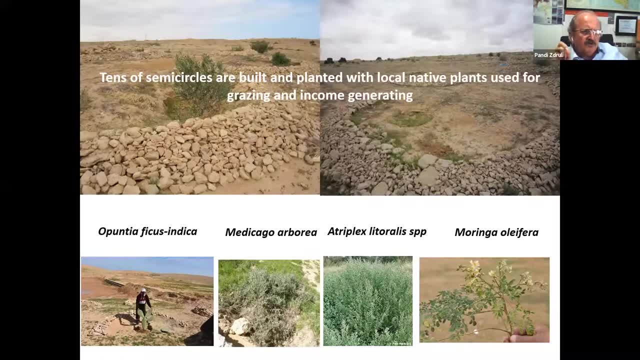 other parts of the world, but that's the case of of egypt. in this regard, we we didn't look only at the flatlands, but we look also on the sloping length of these ones, and then we built semi-circle parapets and we planted this locally adapted- uh, drought resistant salt. 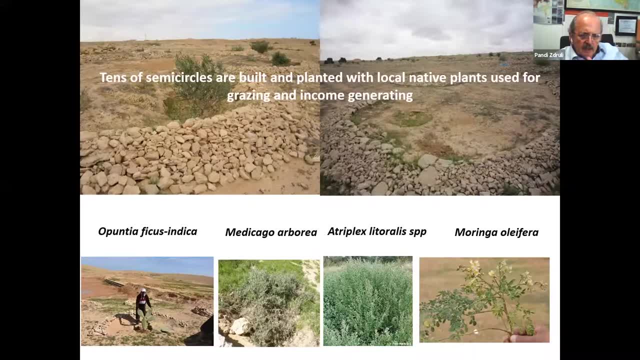 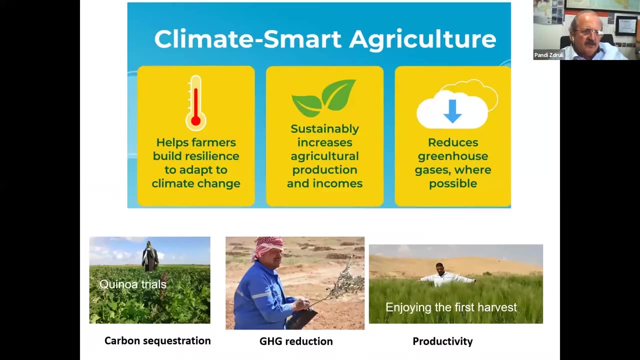 tolerant, resistant crops that were used both for- uh- feeding animals, and i mean people also use the moringa leaves to do as for consumption, but in the meantime, you start accumulating a little bit of carbon in an area that was totally dry before this intervention. we're looking climate smart agriculture. climate smart agriculture is based on. there is three 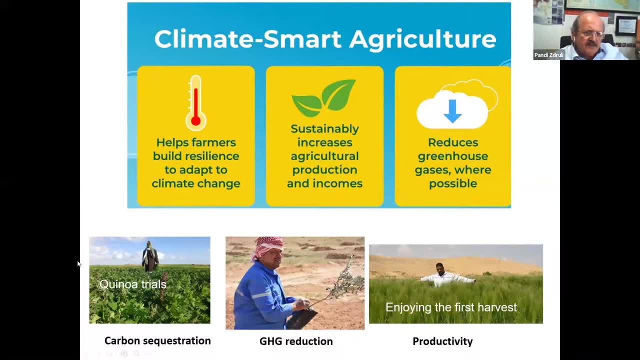 pillars and after all, people know this very well. if you look at the center, you have to have the agricultural production and the increase in income. you have to help farmers build resilience and adapt to climate change and reduce wherever possible the greenhouse gas emissions. so at least with three interventions you can see. we even tested quinoa, a very unknown crop for for that region. 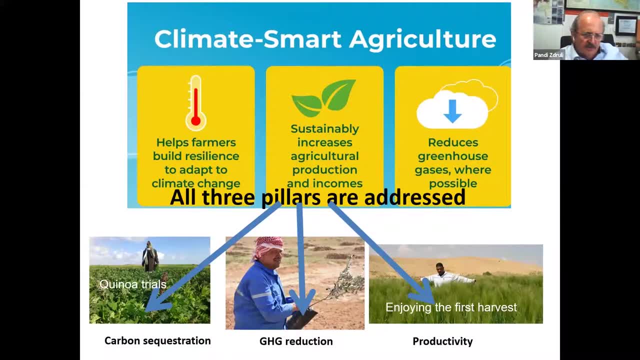 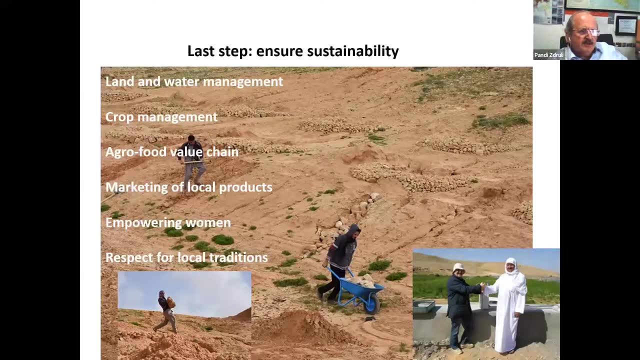 i think we were able to address all these three uh pillars in that particular project. but you have to look at sustainability. it's not just one single intervention, so you need a land and water management, crop management, agro food value chain and marketing a local program, because if farmers have no place where to sell it, 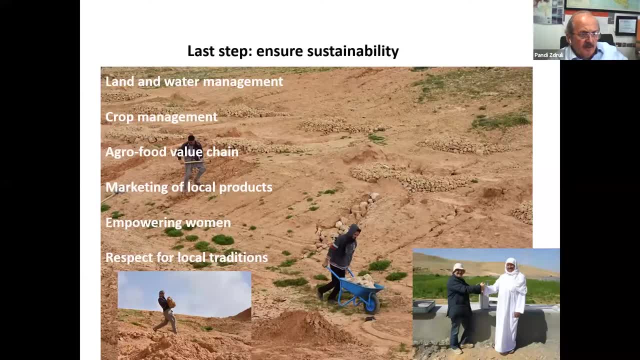 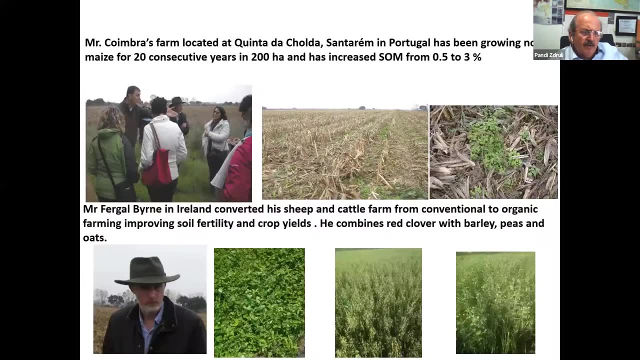 then it become a problem. you have to empower women and to have to respect also local tradition and, by the way, in this particular project we did also implemented this in that way. now there are examples also everywhere and i'm very briefly going to show you some examples of examples of 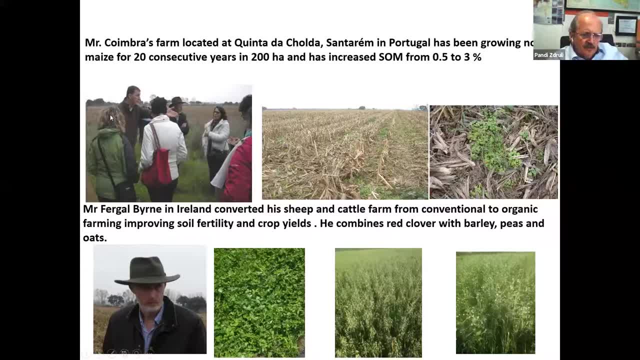 examples also everywhere and i'm very briefly going to show you some examples also everywhere and i'm very briefly, briefly, we'll we'll show you this: this is in portugal. in europe, we have here in europe a european innovation partnership in agriculture network funded by the european commission. 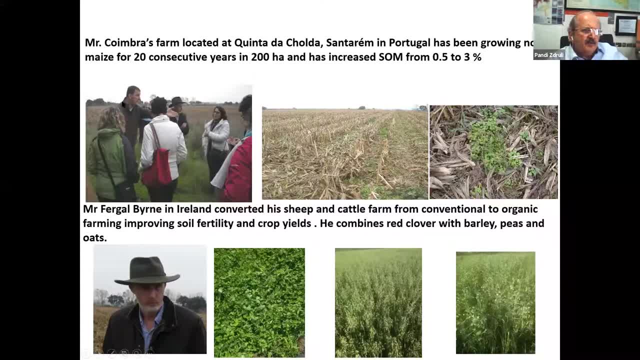 and actually we were visiting this farm in santarém in portugal and this man in here, mr coimbra. he has been growing for 20 consecutive years with cover crop corn with very high yield and he increased all organic matter up to three percent. these are all. 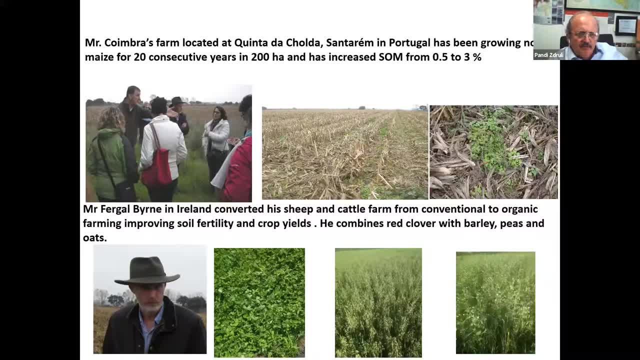 related data. so in maintaining soil health, improving soil health and maintaining good yield, it could be done, and i'll show you also why not everybody is doing. uh, this man also is in ireland, mr fergal bernie. he converted his farm from conventional to organic and by by making a 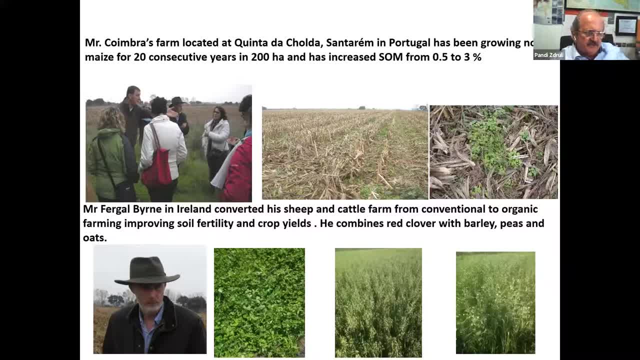 combination of various uh crops that he's feeding his animals and he says that my my fields are quite good and the quality of the my fields are quite good and the quality of the my fields are, the meat is quite good and i'm making also good money. uh, another example, since we are 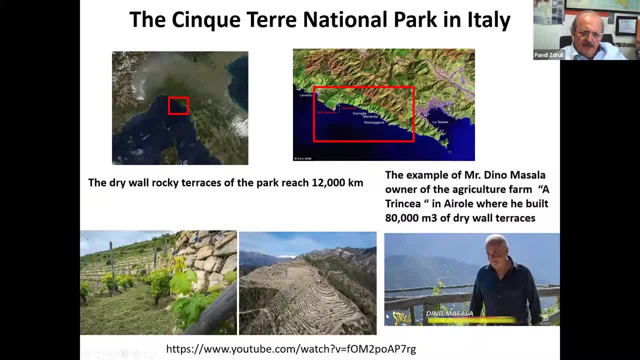 in italy. i'm speaking from italy now. uh, this man, dino masala. you see what he did. this is in. uh, by the way, in cinque terre, this is a national park. he's a unesco property side, by the way. cultural heritage, these terraces, some of them were built even a thousand years ago, but he 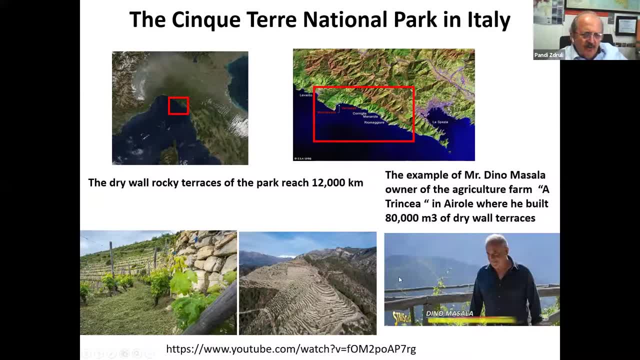 he built eighty thousand cubic meter of drywall terraces in this, a very steep slope growing grapes. he produced a good quality of of wine and he stays there and he was even in the news in the national television media. so let's move to the us. in the us they 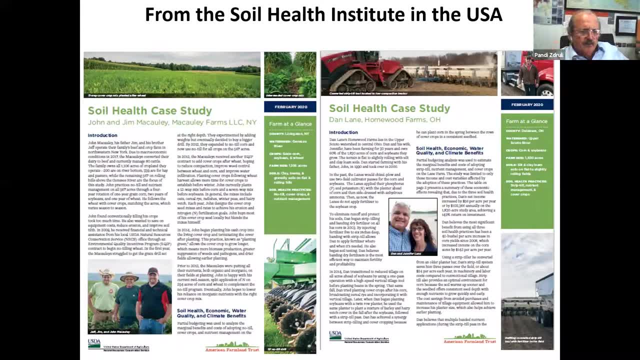 have the soil health institute and there are many things that you can learn out of there, but they produce this very nicely, well done fact sheet on soil health, case studies and they they directly spoken by the farmers. this is three generation of farmers and they look at soil health economic. 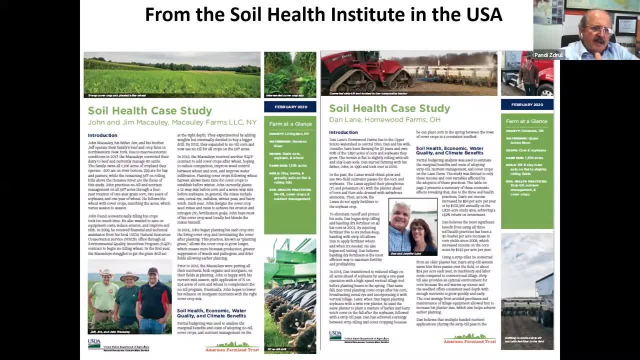 water quality, climate benefits and so on, and i don't have a space now, but if you see, on the next part of this slide of the fact sheets there are also data on economic benefits. so people also were able to make money out of this, because a farmer is also a businessman, there's no question. 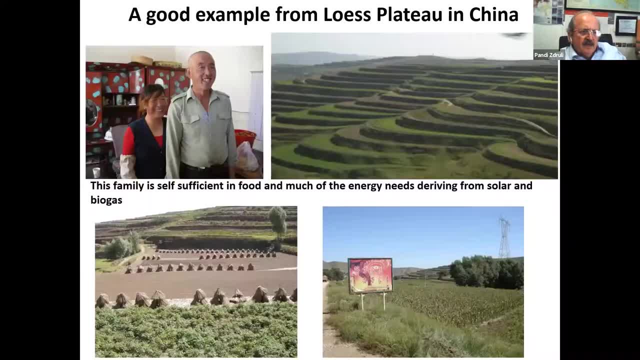 about that. so there are many examples like this. and here let's go to china, and i've been fortunate enough to visit this family in the land zoo with colleagues from london university. we are in the last platform here. uh, they grow potatoes and corn and uh, actually, i, i, we, when we visit with them. 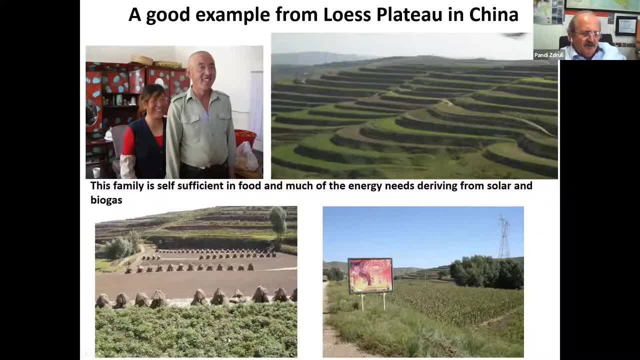 they will. they offered us those very nice potatoes. that was uh quite good for them, and uh they, they also have peaks. they. they use uh biogas for for their energy needs. also a very uh simple done solar equipment, so quite, i would say, also self-sufficient in at least in some part of their 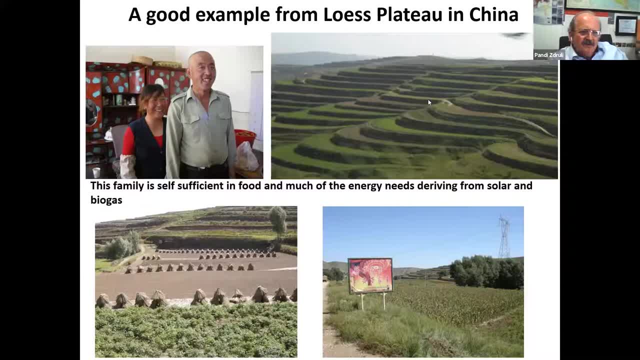 food and energy needs. but there are thousands of factors like this in the last plateau, not only for growing corn and and and potatoes, but also chinese have planted millions of trees and they probably also are accumulating carbon in those areas. so the uncd have this land heroes campaign and i was 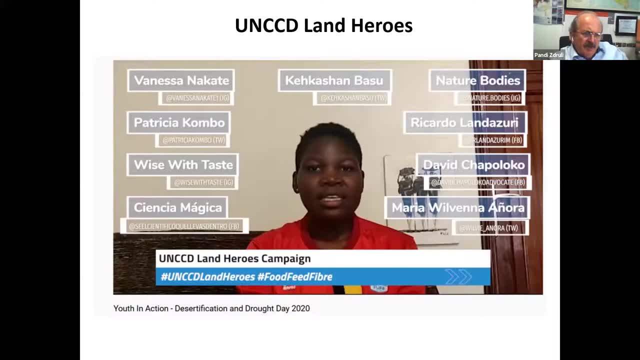 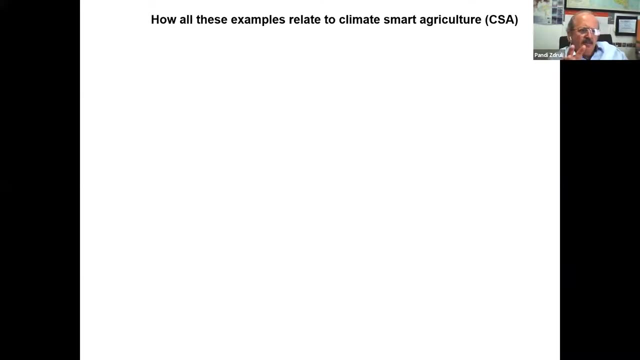 very happy to be part of it because it was just on the 17th a week ago- the day to combat desert, because desertification day- and they showed that there are many other these land heroes around the world that are implementing these practices. so how all these examples relate to climate smart. 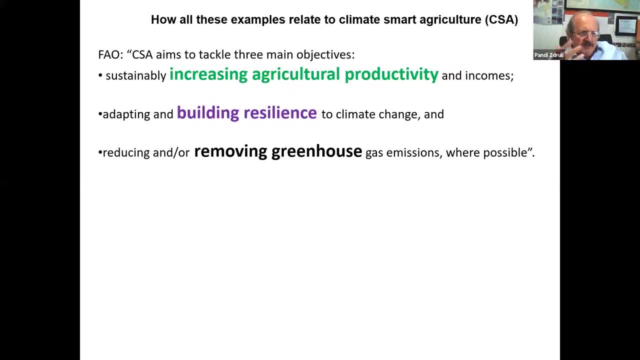 agriculture. now we said that fao uh described the three main objectives that the uh climate smart agriculture plan had in mind. you have to increase agricultural productivity, no question about it- and income, build resilience to climate change and remove greenhouse gas emissions where possible. the issue is how to do this, and i don't think this can be done unless we endorse a multi-stakeholder. 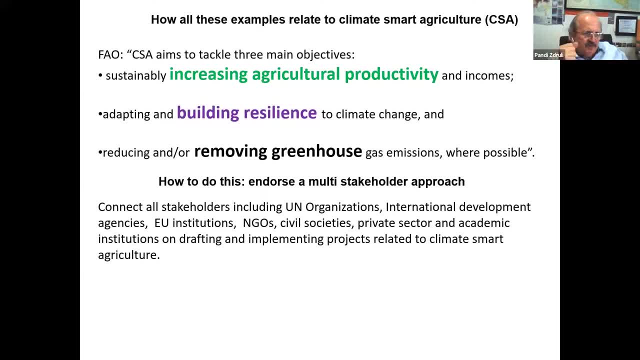 approach where all what i mentioned- the un organization and the international development agency and the eu as well, big player, ngo, civil society, private sector and of course, we need the and research- to come all together and to draft this and try also to implement. Let us don't forget that there is also a global alliance for climate support- agriculture. 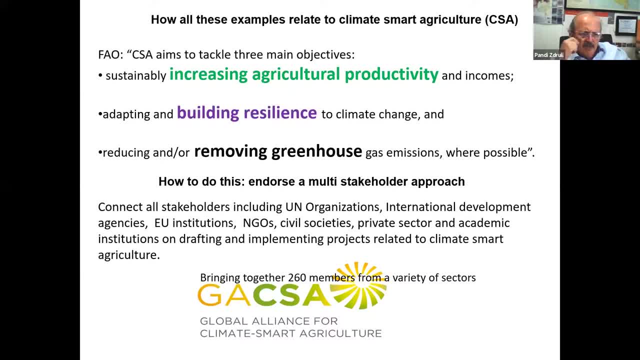 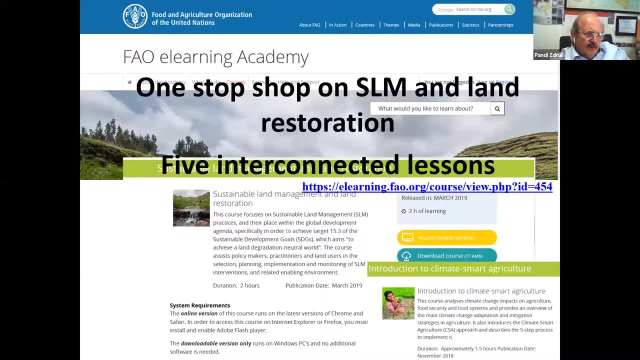 if not mistaken, FAO is coordinating this and brings together 260 members from a variety of sectors. So where to learn more and how to outscale some of these examples that I mentioned? You heard from Kristina that there is this FAO. FAO eLearning Academy was launched also. 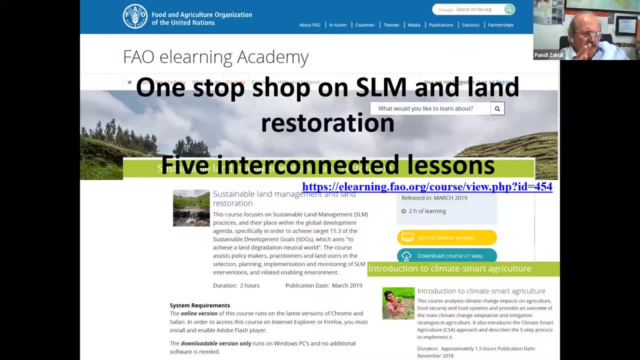 officially a few days ago And within the endless numbers of courses that are there, we, as the Bari Institute, together with FAO and Feras- his team with economics of land degradation, Mark Schauer were there, Lindsay Springer, the walk up people, Hans-Peter Lienegger, Nicole Harris. 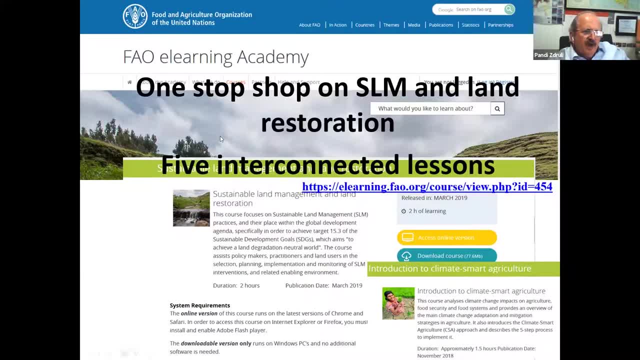 Really all these people. we came together and developed these five interconnected lessons. Here it is the link if you wish to go there, And I'm sure that you will learn a lot because we call that one stop shop on sustainable land management and restoration. 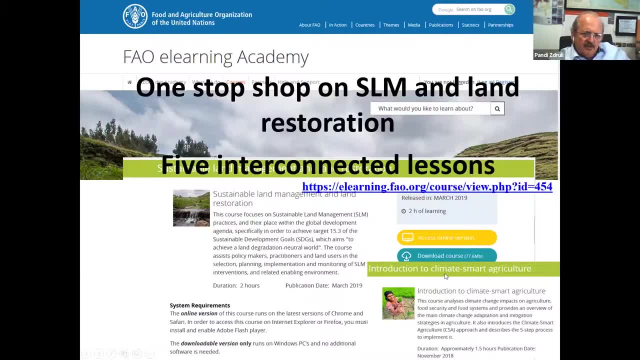 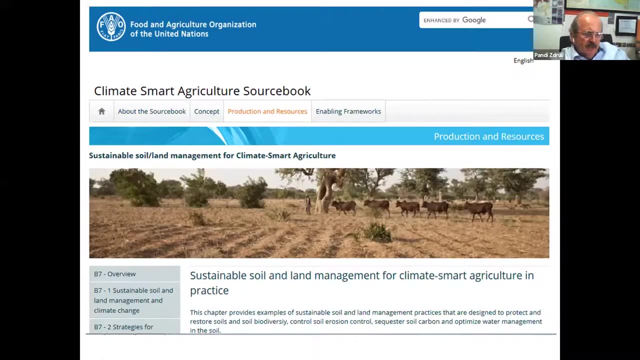 There is also this introduction to climate smart agriculture that also you can find it within the FAO eLearning Academy, So there's plenty of places where information could be found. Feras mentioned also that there is also this sustainable soil, land management, climate smart agriculture in practice, and how the soil can try to fulfill at least these three. 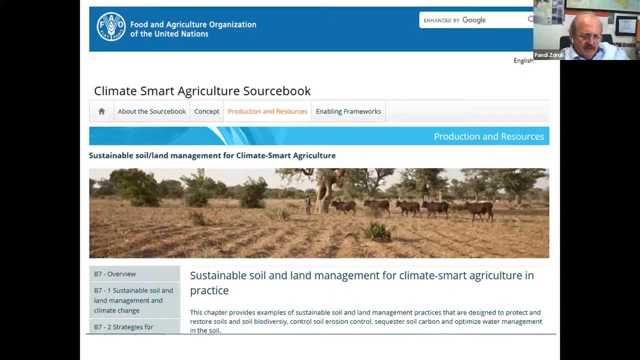 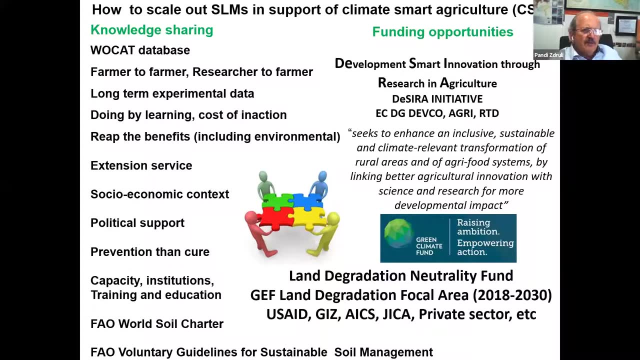 main objectives that the climate smart agriculture has and what I mentioned. So I'm coming almost to the end of my talk and the issue is how we could scale out all these management practices. And there is an issue here because we have to look what you see on the left side of 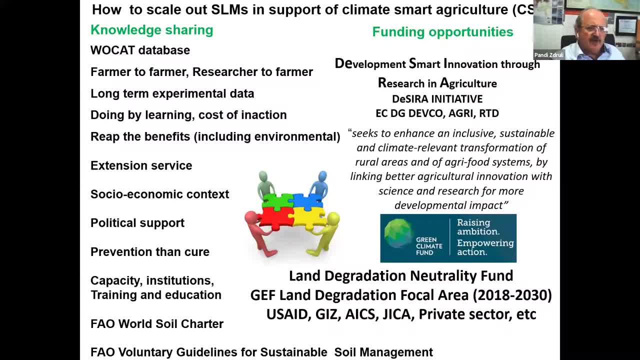 the slide. it is the idea of we have to share the knowledge And I mentioned the walk up. most often, farmer learn from farmer. So there are these. we call it influential farmers, but we also need that the researchers talk to farmers and the researchers have to talk to farmers. based on reliable scientific 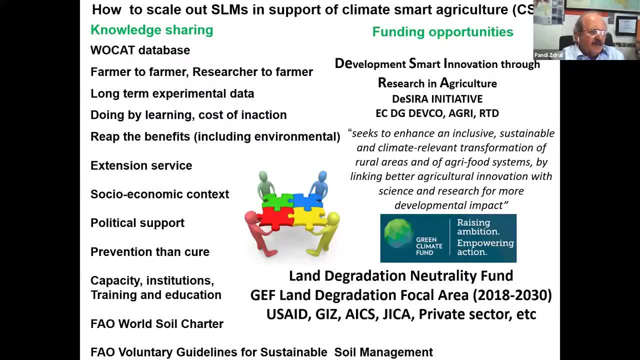 data Based on long-term experimental data. And then it's also quite important that you do things by learning. There's a lot of talk many years now on the cost of inaction, So how much it costs if we do nothing, or can we afford to do nothing now? 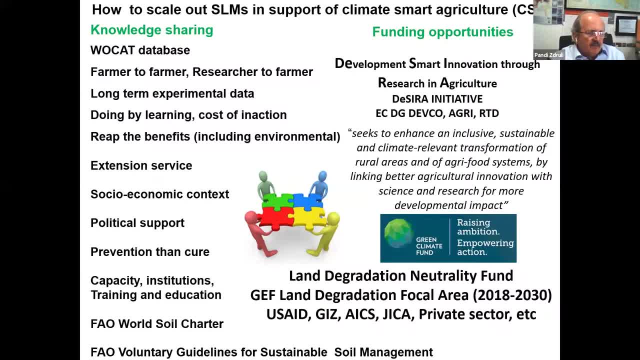 Yeah, I don't think so. We have to, the farmers have to, and us and society have to reap the benefits, which include also environmental benefits. but to do all these things, we need to have an extension services Which are effective, that go straight and tell farmers what they need to do. 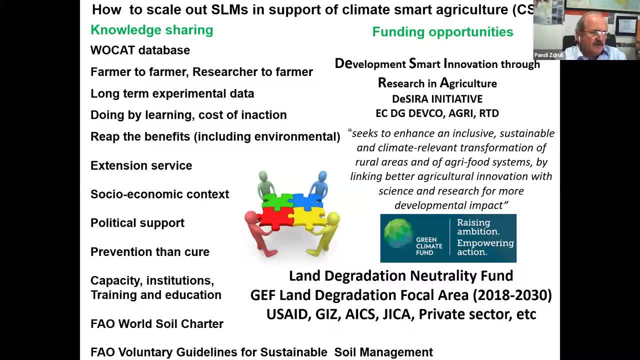 You need to have a socioeconomic context and you need to have also political support. We need to have political support. I mentioned that cost of inaction is very much linked to the prevention than cure. So it's cheaper to prevent than to cure a disease. 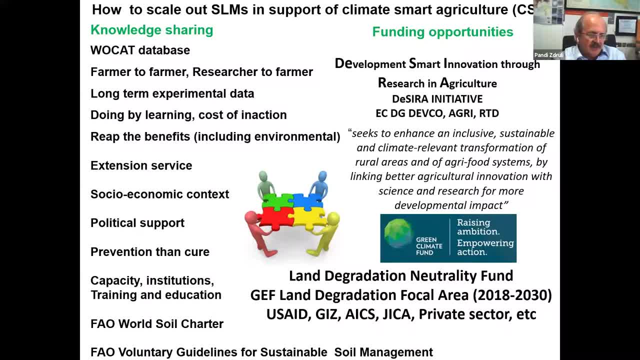 Then you need the capacity, institution training and education, And I'm glad that I see quite a number of students attending today, So that's good for you. The FAO revised the World Soil Charter in 2015 in the occasion of the International 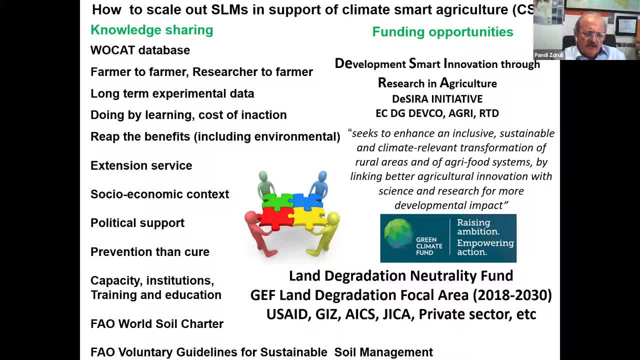 Year of Soil, And there are also the FAO Voluntary Guidelines for Sustainable Soil Management. I would be happy that these, from voluntary maybe become not legally binding but more kind of say, obligatory. Now there is the other issue that, okay, you have to do this thing, but you need money. 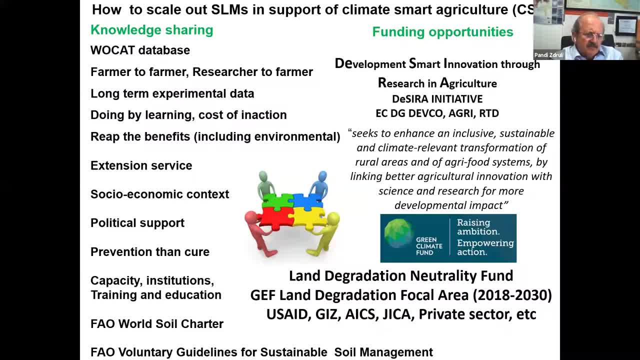 And to do so you need funding opportunities. I would say that there are. There are available a lot of options to figure it out. where is the money? For example, here in the EU, there is this DESIRA initiative Developing Smart Innovation. 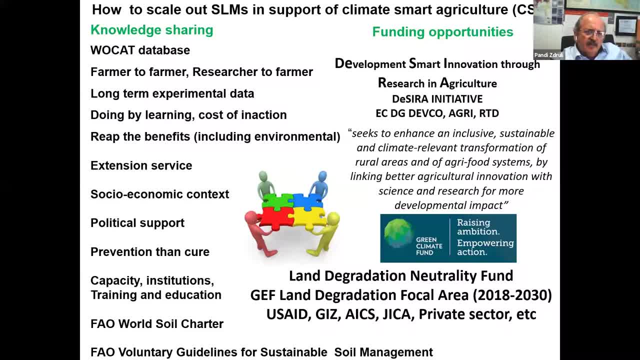 Through Research in Agriculture. It's coordinated by the European Commission DG DEVCO, collaboration with AGRI and RTD. And look at that. How relevant is this initiative to climate smart agriculture? the DESIRA seeks to enhance an inclusive, sustainable climate. 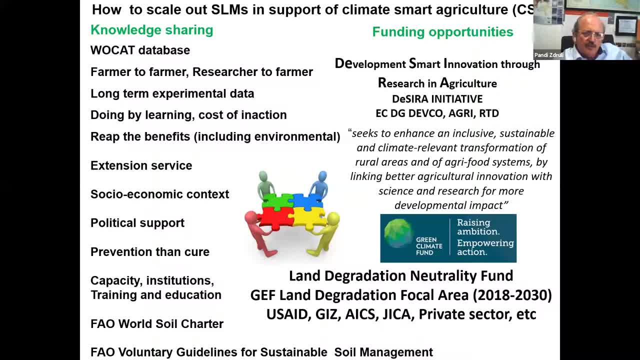 And I think that's a very important part of what we're trying to do here in the EU is to create a climate-relevant transformation of rural areas and of agri-food systems by linking better agricultural innovation with science and research for more development impact. 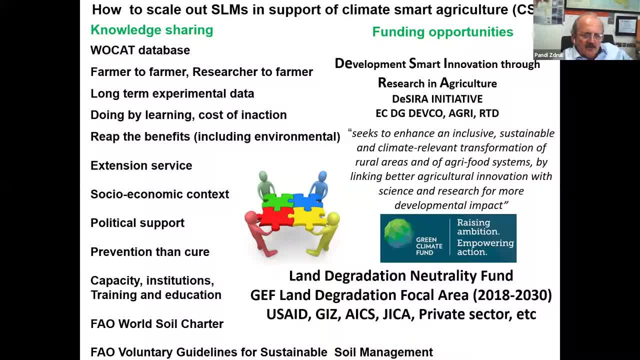 There is the Green Climate Fund, There is the Land Degradation Neutrality Fund that UNCC is following, There is the Jeff Land Degradation Focal Area that has to go all the way to 2030. And, in addition to that, there are a number of development agencies who are like I mentioned. 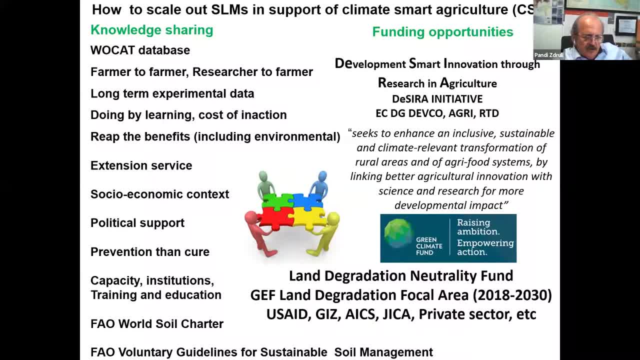 in the other case, non-governmental. We have a project in Egypt, the USAID German Corporation, Italian, Japanese, the list can go even longer- And in many cases let's also say, there is a private sector. So sometimes there is not only an issue of money. 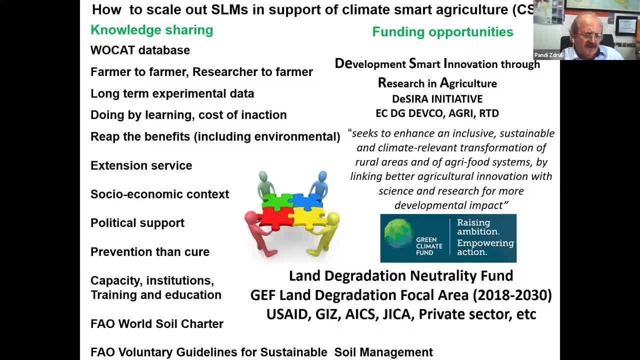 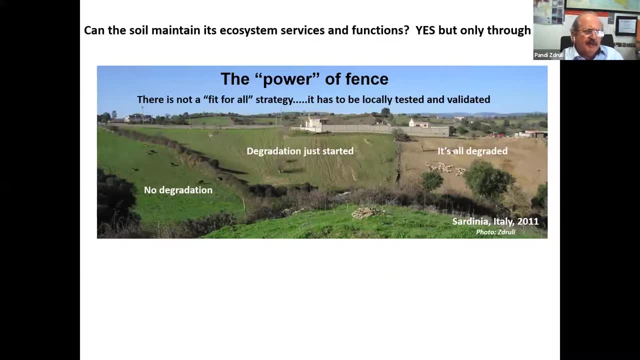 We did, with Paris, an assessment on the Mediterranean countries, and sometimes there is money, but you cannot use that money for a set of reasons, including the socioeconomic and political conflict. So, coming almost to the end, I posed the question: Can then the soil maintain the ecosystem, function and services on a sustainable way? 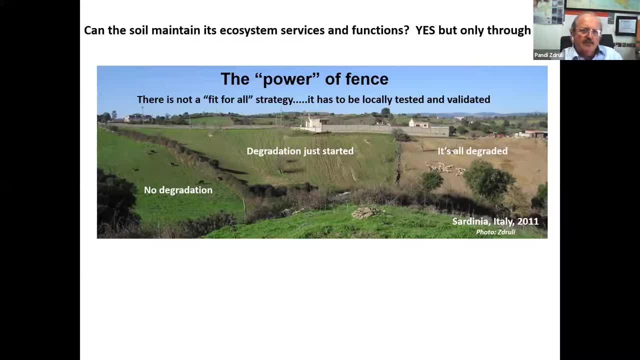 on the long run, I would say yes, but only through sustainable land management. And to do so, I give you a very practical example. I took this picture myself. we were in Sardinia in Italy in 2011,, and you see this piece of 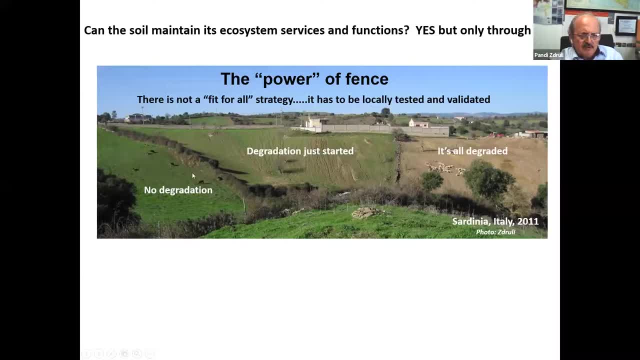 land in here. It is the same slope. It is the same soil: Characteristic: physical, chemical, biological. It is the same soil. It is the same soil Characteristic: physical, chemical, biological, whatever you want. But it is a big difference between all these three parts. 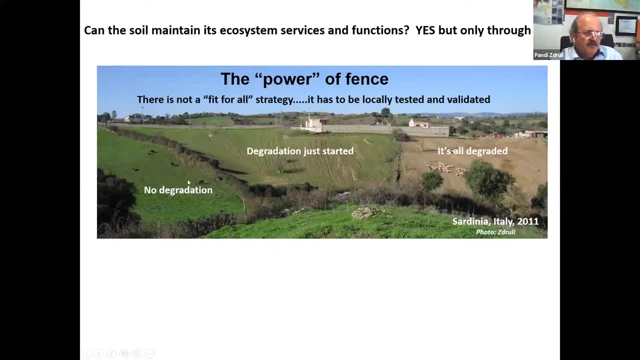 There is almost no degradation here. A very few number of cows grazing. I don't see any form of erosion, no compaction either. Here the farmer decided to plow up and down And you see this rill, And maybe after 10 years they have become gullies. 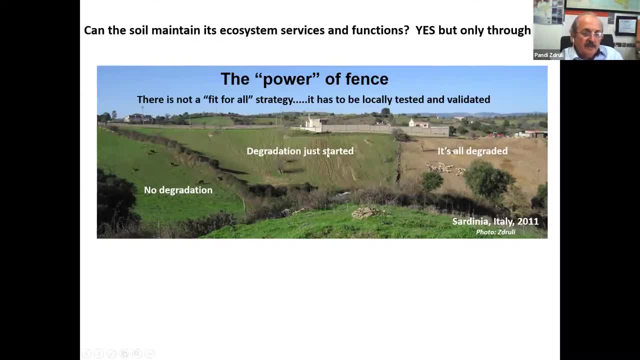 It would be nice to go and see what happened in here, but here the degradation at that time it just started. It is almost all degraded. It is overgrazed. number of animals here and there is not a single grass somewhere. 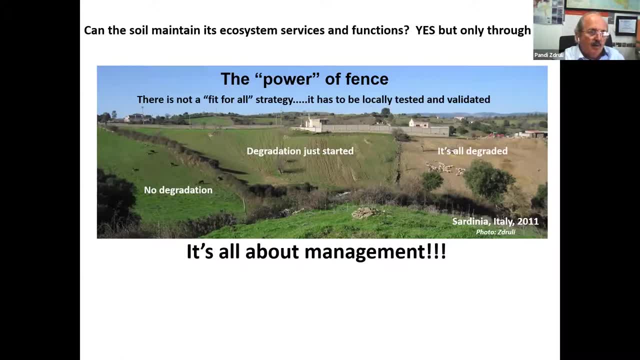 So it's all about management: how we manage the land and the soil and the water, And how we discuss today about climate-smart agriculture, and that's fine. But let's face it that there is kind of- I would not say- competition, but there are. 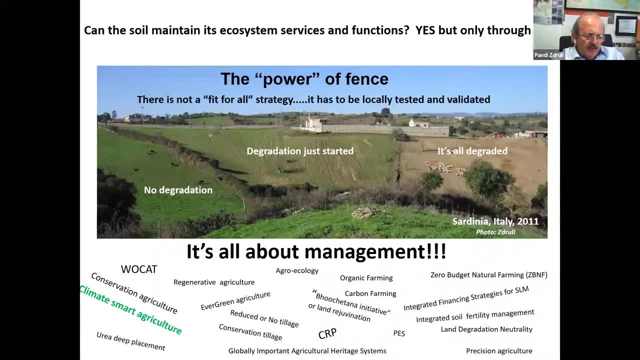 so many names that are moving around, Like, I don't know, Conservation agriculture. Claire described that In the US and Canada they prefer much more to speak about regenerative agriculture. I was reading the other day a paper in Vogue, and even the fashion industry is producing. 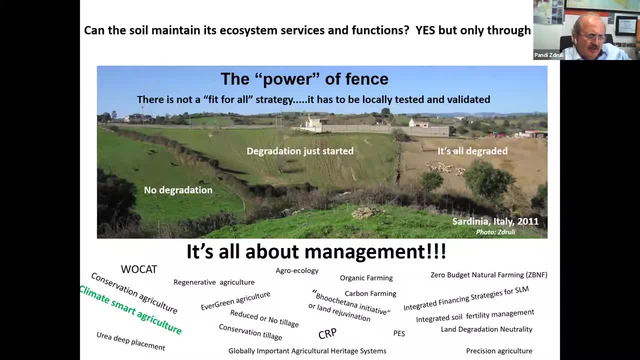 cotton in India through regenerative agriculture, which is fine, perfectly fine. Agroecology was mentioned, Organic farming. I gave you examples. There is also carbon farming, So farmers are paid money for sequestering carbon into their soil. You can have precision agriculture. 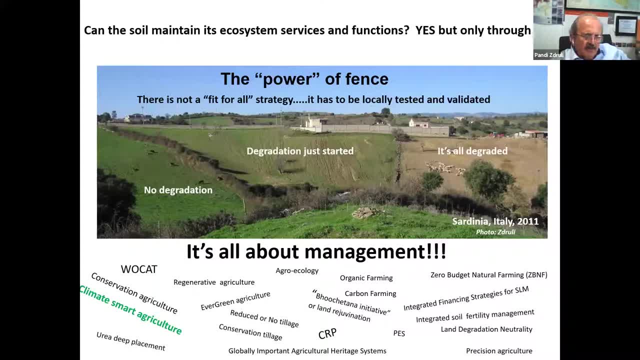 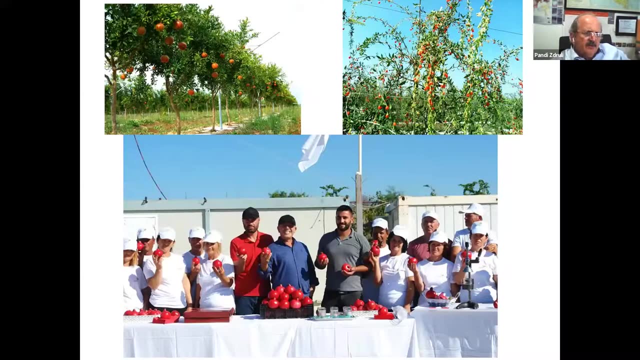 So there is a set of technologies which are not that different, in my point of view, from each other. Important is if we implement them in the right and in the correct way. So this is my last slide. I'm showing this because it's quite interesting. 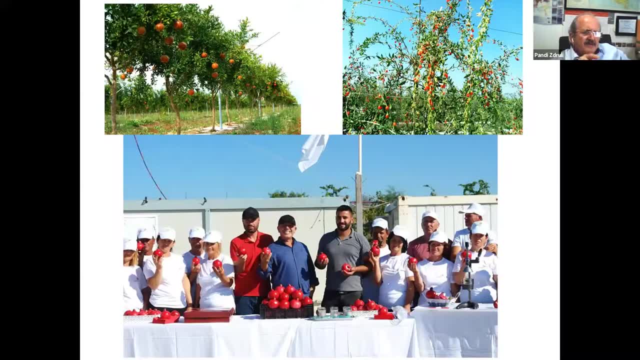 This comes from my home country, by the way, in Albania, and this is an area where the soils are still Quite salty. That's a lie. there I surveyed myself about 20 years ago, and here now there is a farm with 500 hectares. 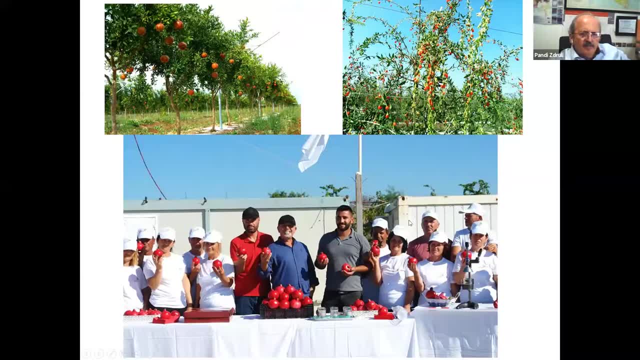 by a private businessman that's been in here with some other people, probably through implementing sustainable irrigation systems, sustainable land management system and finding the right crop. You can see we're talking about here pomegranates and goji berry. 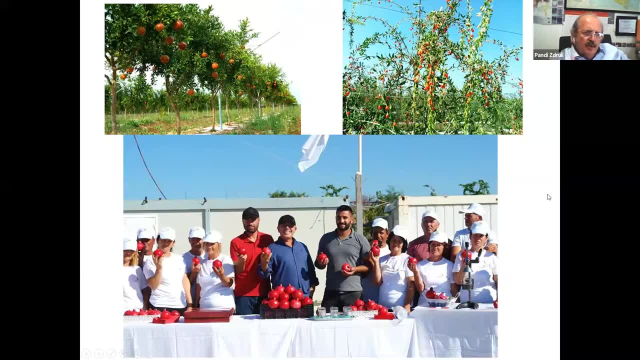 Both of them are quite salt tolerant, So they are now in full production. They employ local people- You see many women as well- so people don't need to move to the city or migrate somewhere else where options are given, like the example energy that I showed, or even this one here. 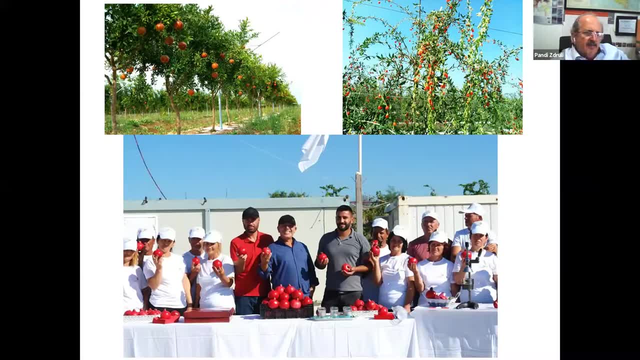 It makes sense and it shows that things can be also done if we put together this holistic combination of all stakeholders. And with that I'm done With that. I thank you very much for your attention. Hope I was within my time, well located. 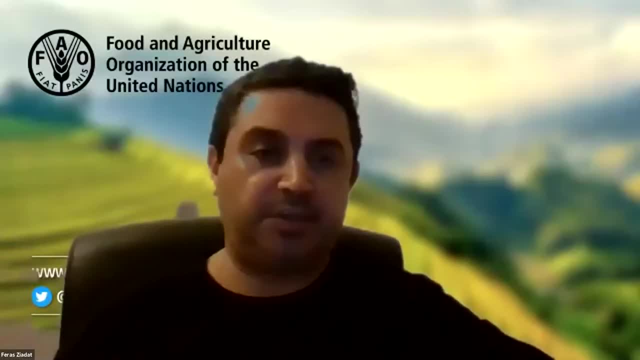 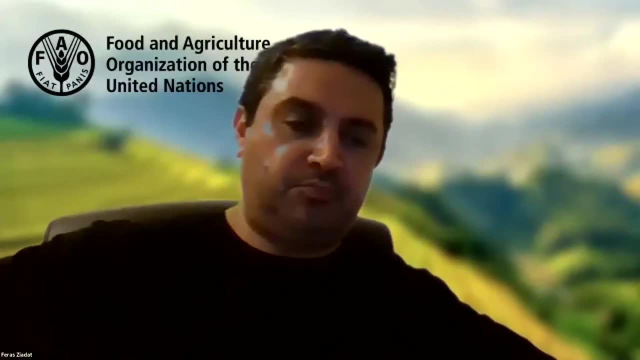 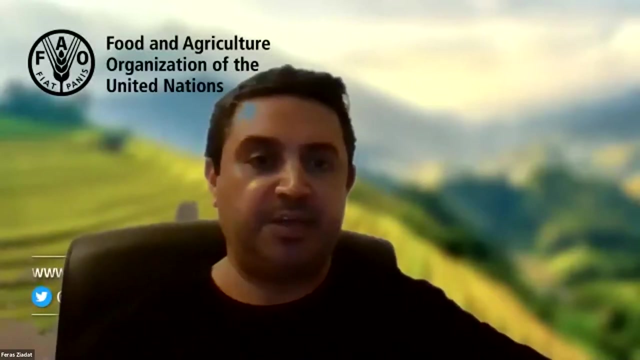 Thank you very much, Andy, for this presentation. I'm glad that we have the two presentations. Now we shall move to answer some questions. We have some 30 minutes to interact with the participants and we have quite a number of questions. 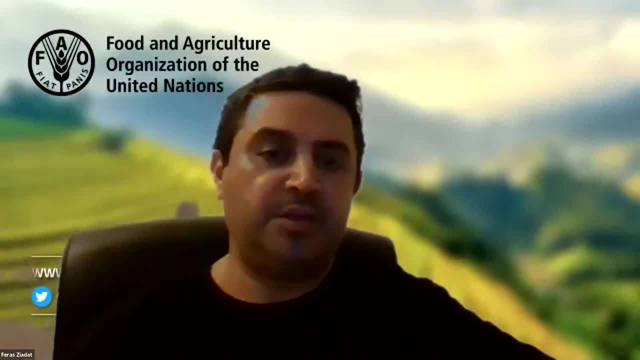 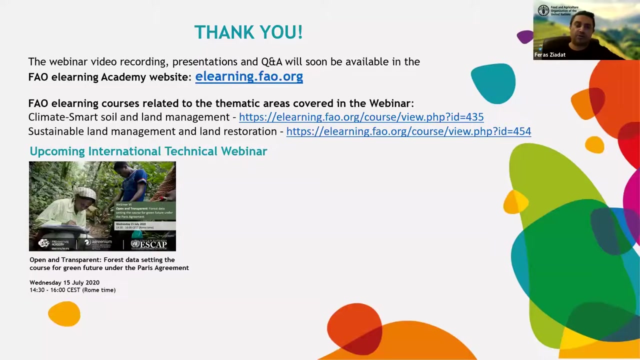 And the Q&A bar. So I will give first the floor to Claire. If you have picked any of the questions that you have you would like to comment on, or we can pick some questions, because I don't think we will be able to answer all questions. 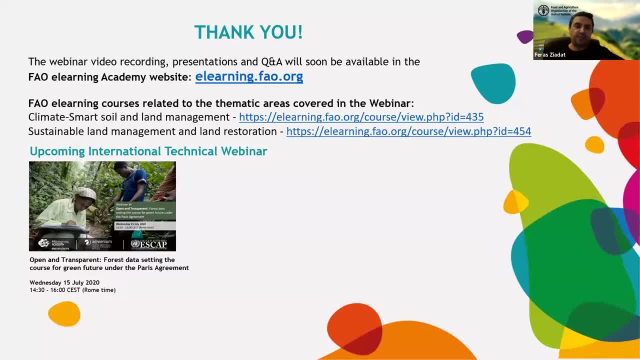 We will if we missed any of the questions. And if we missed any of the questions, Thank you. And if we missed any of the questions, we will try to answer all these important questions. Do you hear me? Yes, Yes, Claire. 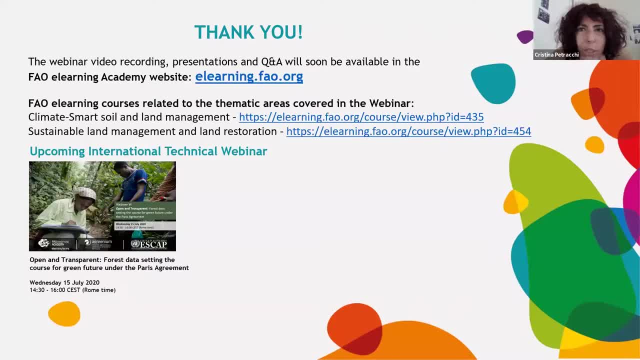 Please go ahead. So basically just a second. what Faras was mentioning is that we will try to answer to some of the questions And then we will also put together the Q&A. Okay, prepare a document. after the the webinar where, where the experts Pandy and Claire 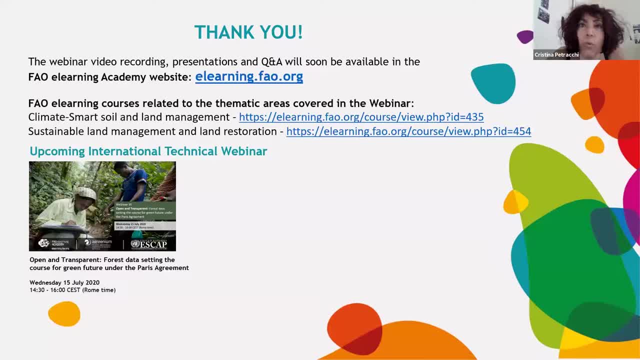 will respond to most of the questions, and this document will be available on the FAO eLearning Academy together with the recording of the event. so, Claire, please, the floor is yours to answer some of the questions that that you picked. okay, well, there are many questions and many exciting question, I mean. 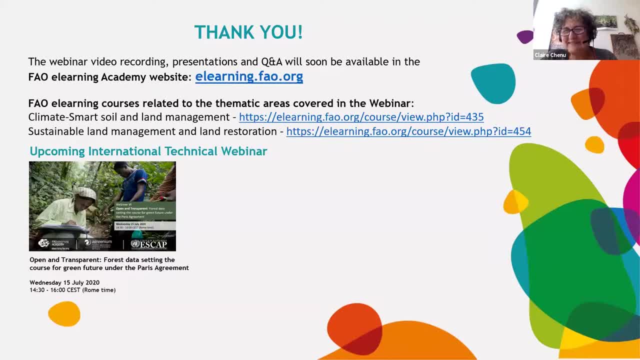 challenging ones, so thank you to all the attendees. I saw that there. maybe I will first pick up questions. I answered partly typing, but there are several questions about the risk, when you implement sustainable management options, such as conservation agriculture or agroforestry, that your yields decrease. 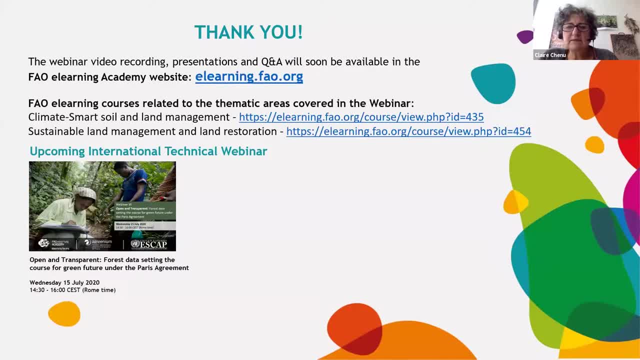 so the answer from that is that it is extremely dependent, of course, on the context. that, regarding conservation, agriculture is quite often- while at least publications show that it's a temporary issue- time of learning, time to learn how to master to control the pests. we're time for the earthworms to be back. 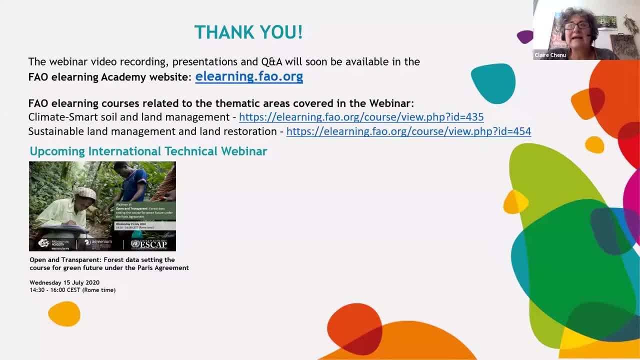 to improve soil porosity. and but well it's. there's a point of this transition period regarding of agroforestry. it is true that when you plant trees, you decrease automatically the surface area of your crop there because of the roles or the places where you have planted the trees. 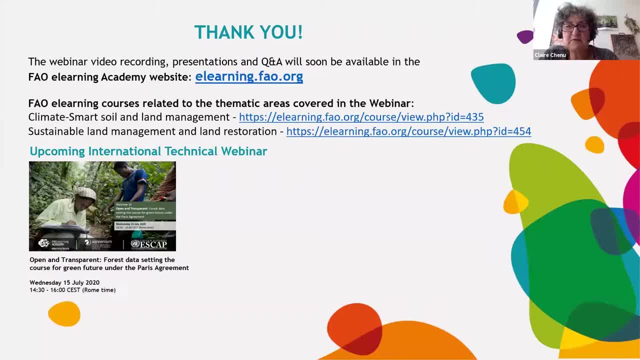 yet there are two facts. first, and it was mentioned in the question, it's an important option to choose trees that bring you some revenue, for example fruit trees, and also there are situations where, in fact, the yield per surface area is higher in agroforestry, and this is quite 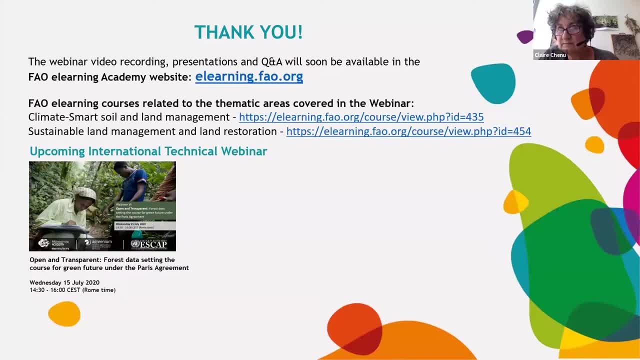 uh occurs quite often and has been analyzed in mediterranean areas as well as in tropical areas, because of indirect effects of recycling, of maintaining the nitrogen at the in the upper layers of soil or shedding the crops. so yes, it's a complex analysis. so maybe pandi wants to develop on that. i think maybe you could. 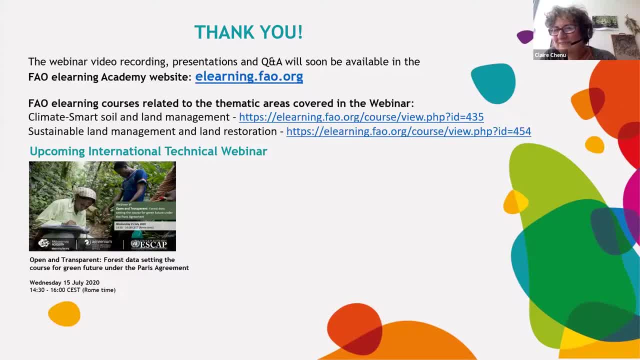 do you want to complement? well, i, honestly i was also looking at all the research that has been done on agroforestry, all the questions that were made and uh, uh, the uh. the topics are quite diverse and uh, of course, there is not a single answer that could respond to all. all what, uh, what was? 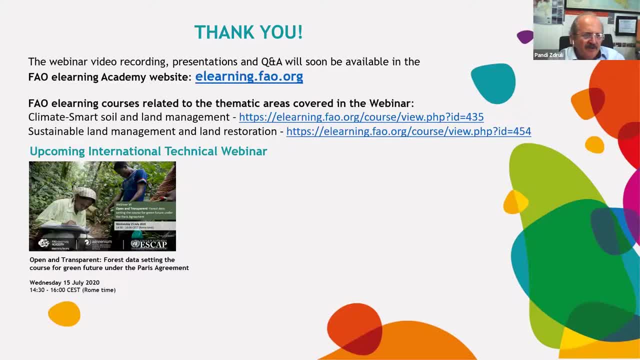 mentioned. uh, for example, i have in here that how small farmers in africa can improve yield and preventing soil from erosion and degradation is small farms or farmers have small acreages, so of course, the size is also an important factor. if you how to to implement that. the examples that i showed are some of them- that 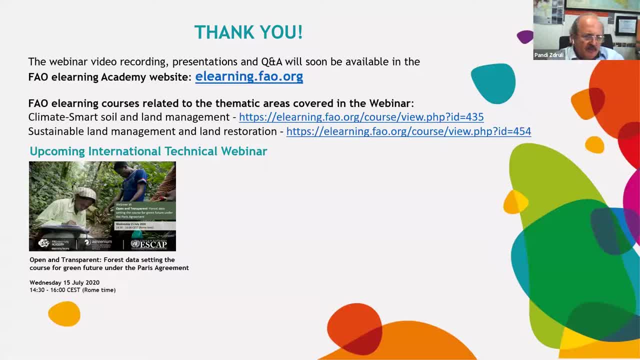 are being uh implemented also in in in terms of cooperation with various development agencies uh, which also provide the advice to farmers through extension services, and they can also help to disseminate and to uh uh kind of uh enlarge and outscale these practices. this is, of course, it's a it's a long process, it's not going to be done immediately, but it is also. 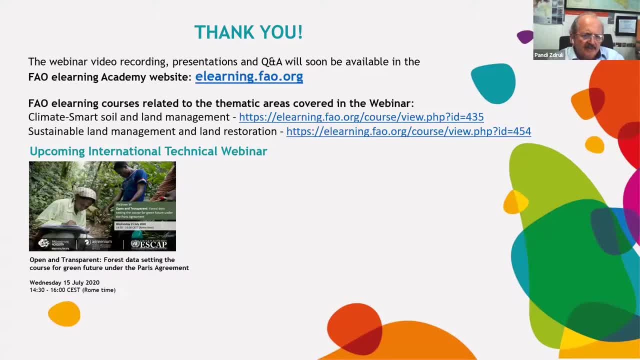 good to know that farmers learn from each other when they see that there are results. if they they kind of in the beginning, they they will not accept immediately whatever technology is being offered. uh, they want to make sure that if i change something, i need also to get the, the benefit i need to have, uh, the income from my, my farm, and then, of course, 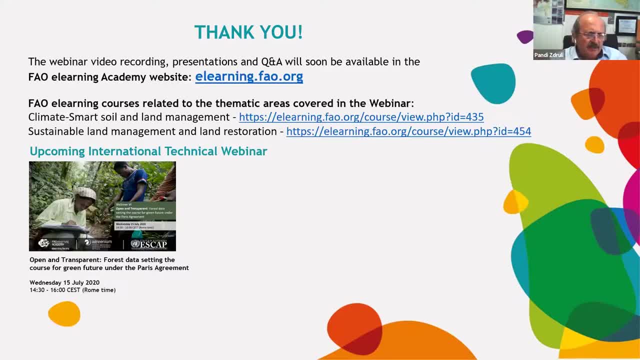 they'll be definitely interested to keep their soil healthy on on on the long run. so that's what i i could add to the whole topic of discussion that is uh, uh being given here, uh, one question i also would like to pick up. um one of you asked what are the easy monitoring and evaluation of soil? 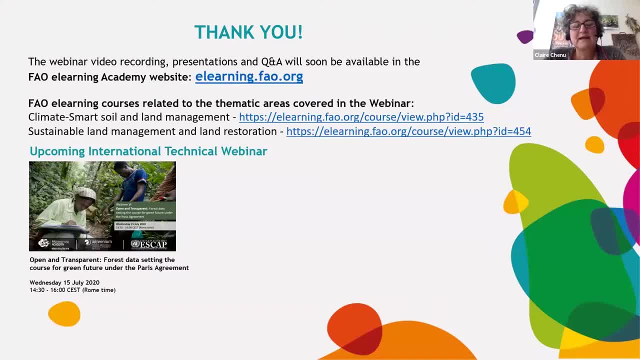 methods that the novice young farmer could use. and well, i think- and i guess pandy will also have his opinion on that- what i would propose is what is named visual assessment of soil structure. it has been developed. i know a lot in brazil and latin america. there's also- it has been a lot, quite a lot. 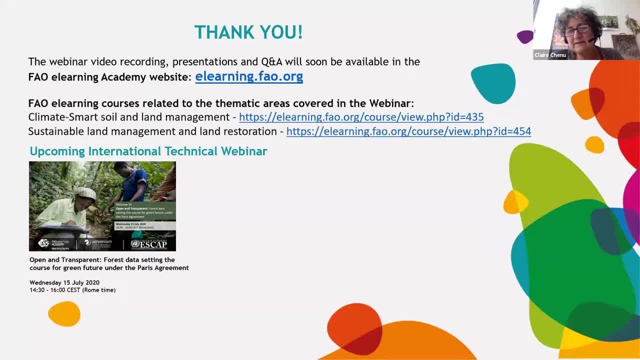 developed in switzerland, in the us. it's basically, uh, taking a small volume of soil with a shower, well, and analyzing it, so you have a guideline, and analyzing the porosity, the color, the presence of earthworm galleries. so it's, it's very easy to well, you do not need any equipment and i think you learn a lot from just observing. 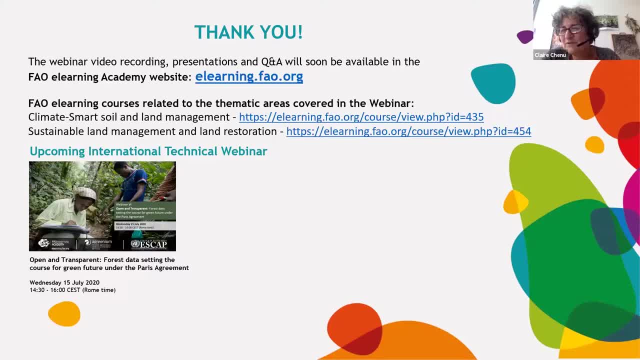 your soil using these, uh, these guidelines. so i don't know, pandy, if you have even even fao had developed a visual, okay, for the uh defining the main basic soil characteristics. so those are are quite simple and, uh, you, you, you can use them without too much. uh, i mean, of course you need some basic training. 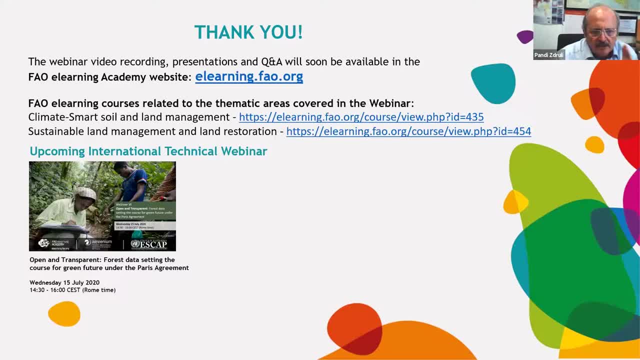 but it is rather quick and and easy going to identify what are the main basic soil characteristics that one can identify in the field and make a kind of uh, like you can look at the earthworm, for example. the number of forza- yes, an indicator of soil health. 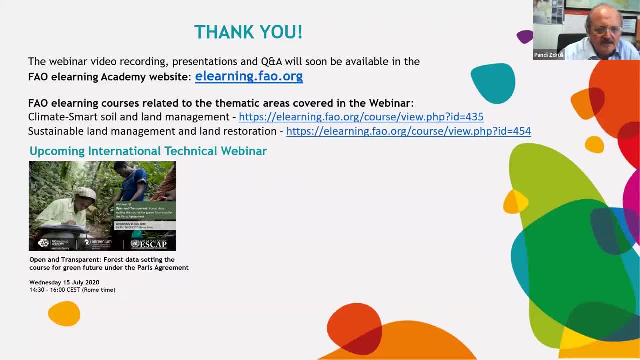 and many other characteristics that are easy to to look at, i think. thank you. many participants are asking about a certification and uh, i just wanted to mention that. uh, on the fao e-learning academy, we have a series of courses related to climate, smart agriculture and also uh. 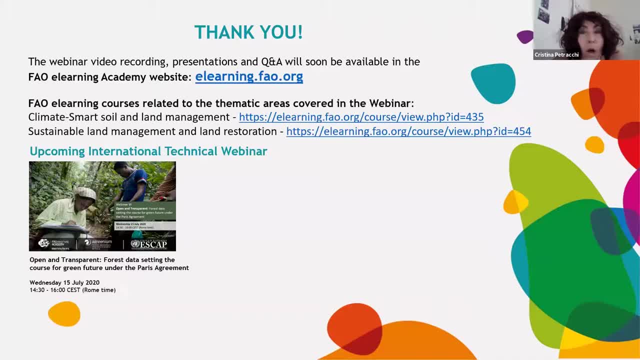 management- soils management. These courses are all related to the webinar of today and they are all certified through the digital badges certification system. So this is a certification system that certifies the acquisition of competences. It is a very, very valid certificate. 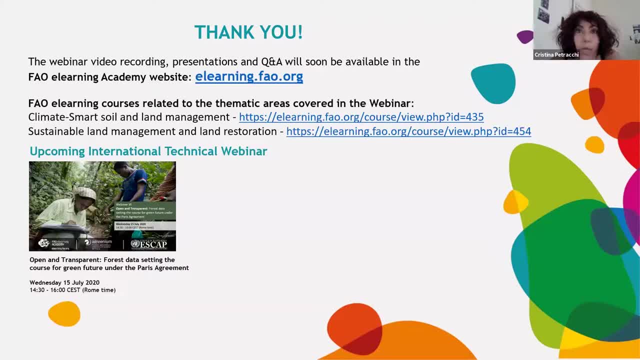 Also, especially now that the FAO e-learning academy is actually the official legal certifying body of FAO. So please visit the academy and you can do the ones on climate smart agriculture and soils and soils management And so that one you can get is associated the certificate. 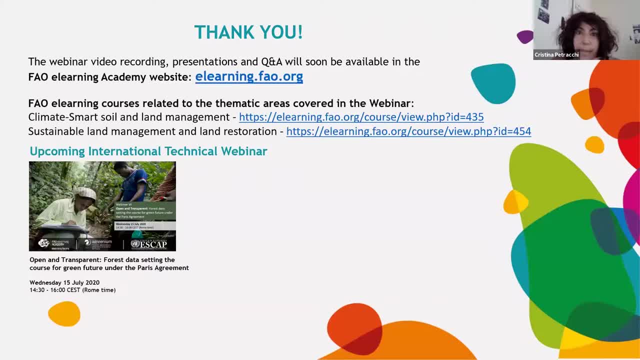 is associated to the course and you can get it and it certifies your competences. So you have the links here. also on the screen, You have the link to the academy and to the courses And Feras. would you like to add something? 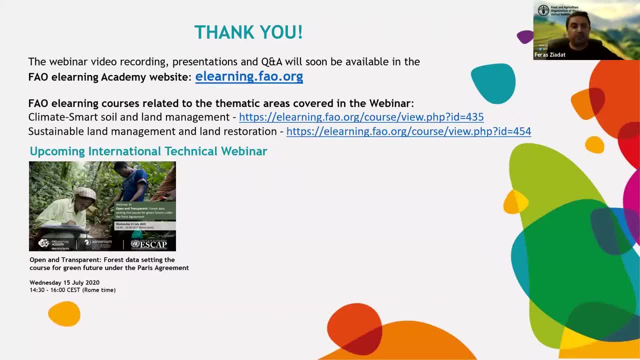 Thank you very much. I'm sorry I was dropped from the call. I missed the discussion. Thank you. I would like to add to the point that was Pandy and Claire mentioning that FAO is also now developing the soil doctor program where people are trained how to characterize. 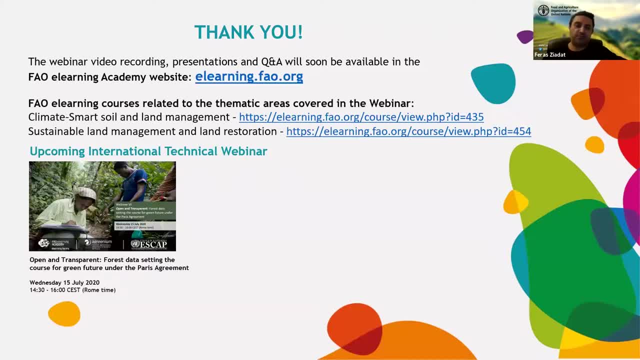 the issue, the problem, and then how to find some solutions, which is based on the FAO, which is based also in some robust but easy and affordable techniques that will be used. That's just to compliment the comment. I find I lost the question, but I have one. 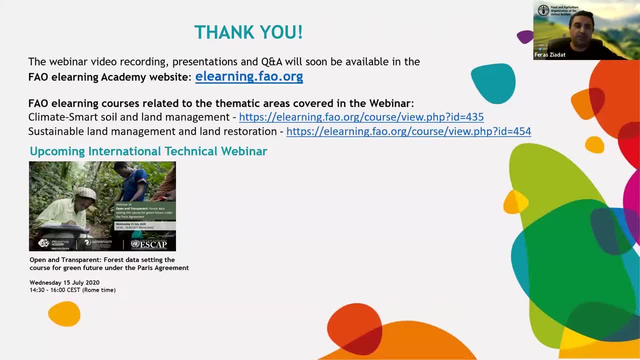 question which probably is important. The question is that no tillage agriculture is significantly important for soil conservation. The question is that we have to use the soil for natural conservation and save energy and labor. However, it has not been widely used all over the world. 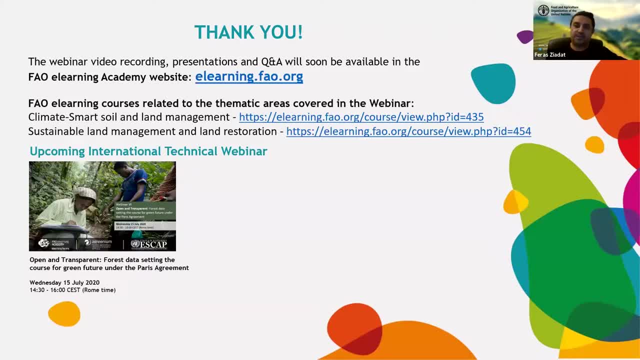 Reasons and what could be done for it. I think this is a general question for sustainable soil and land management that, from a technical point of view, we know a lot of techniques and practices that have been tested and evaluated in different conditions. However, the scaling 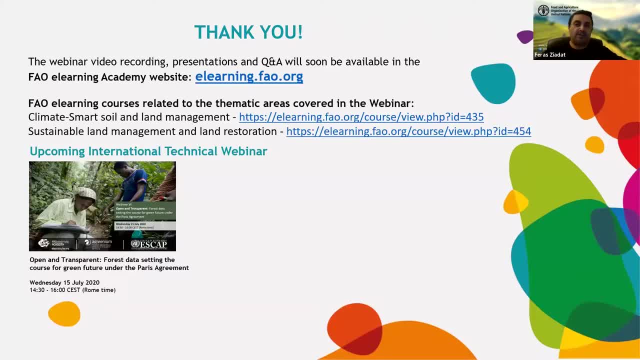 of soil can be very difficult. I think that we need a lot of time to analyze the systems and if you have many questions, please feel free to ask. You will get a lot of time to answer them. of these at larger scale is still not as we we want it to be in order to to 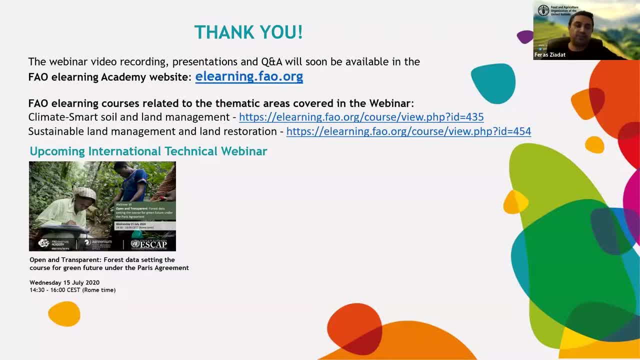 really enhance a tangible impact on land degradation, and this is a challenge, because we have knowledge, we have the needs, but we don't achieve a larger scale implementation and behind that, both brandy and clear touch the enabling environment and all the whole process behind scaling out these technologies. 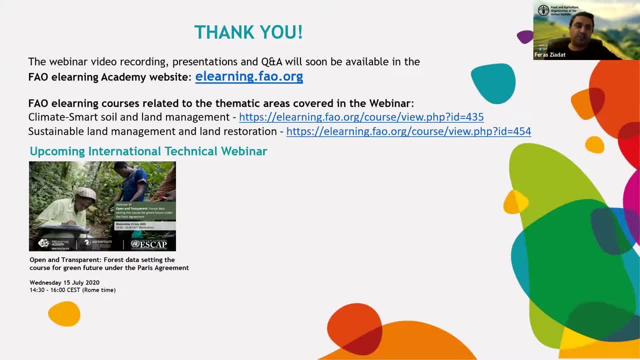 and practices, that there is a lot of requirements in order to make this happening, from the knowledge, the training, the capacity building to the finance availability of resources to start this process to the. also to provide some evidences that this will work in different environments. also to provide 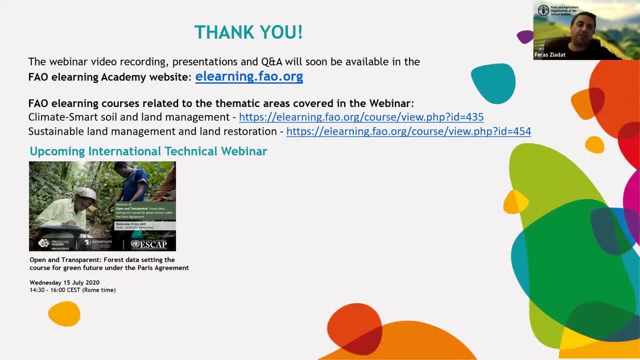 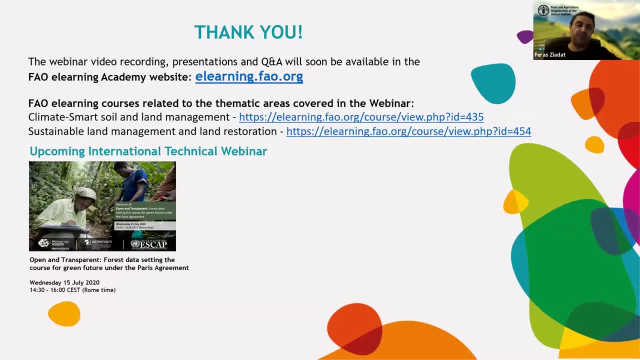 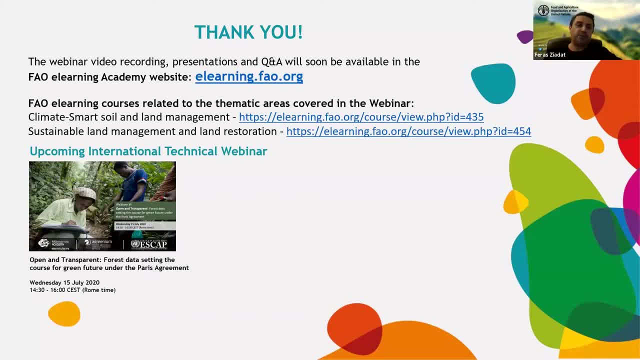 some by two spots where we have some implementation of these technologies, for example in the greater green wall, in different parts of Asia and Central Asia. there are, by two spots where the scaling out and implementation of some technologies are gaining some, and back to you, Christina, maybe to manage the time and tell us what now. just thank you very much to all.